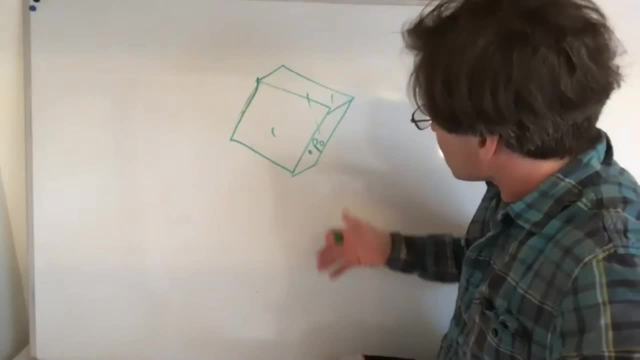 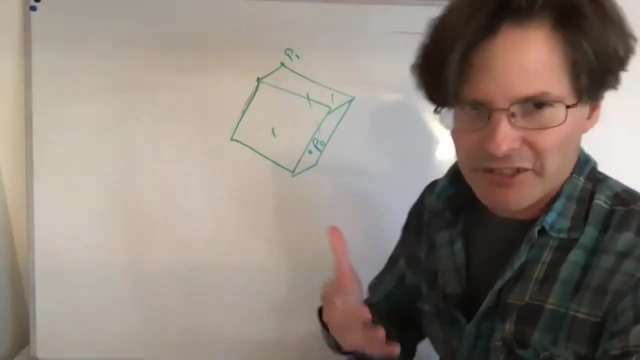 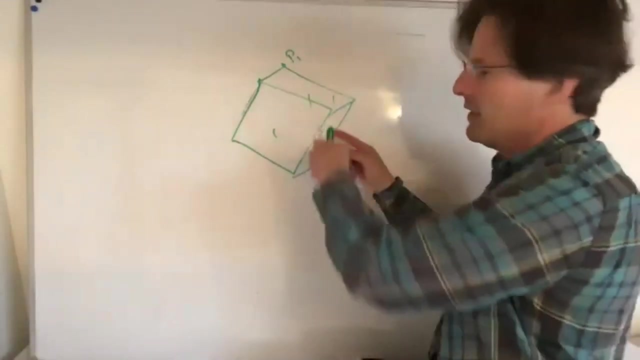 problem in math. So there's some other point which is farthest away from it, and if you ever say the surface of a cube, there's two ways that you could do this. One way is you could say what's the farthest point just in terms of the distance in three-dimensional. 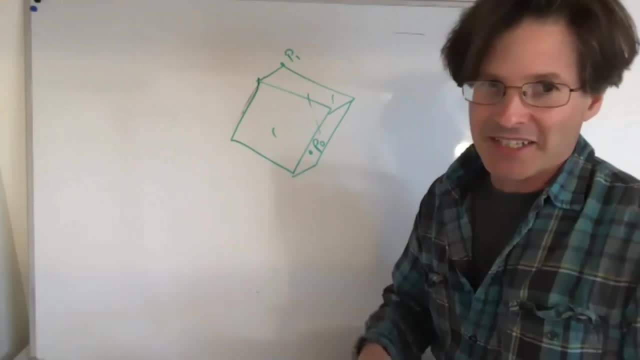 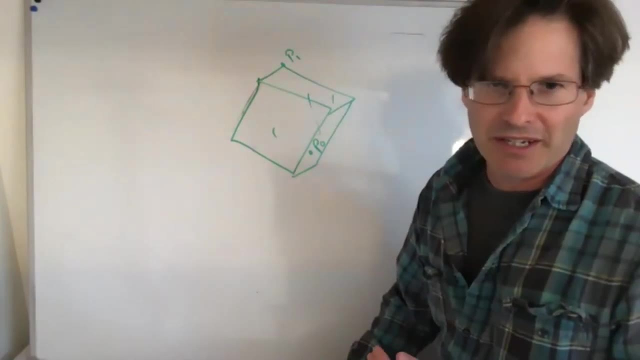 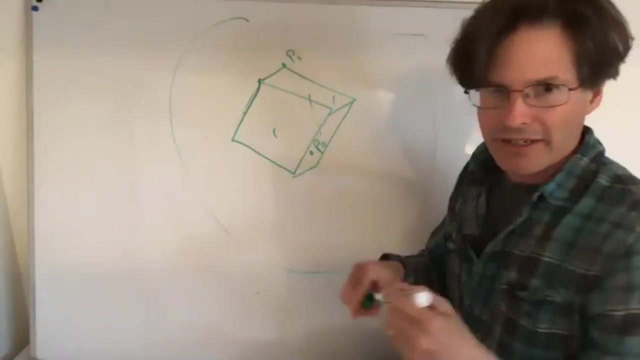 space, And in that case it's not that interesting, because the farthest point is always going to be a vertex of the cube, And the way to think about that is imagine something like a, like a big sphere that's centered at this point, and now imagine this thing just kind of like shrinking like a balloon, and then when 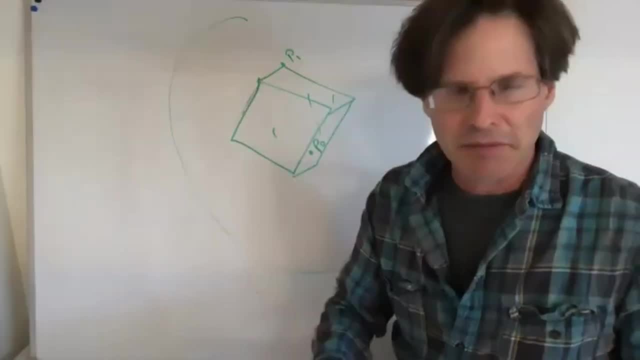 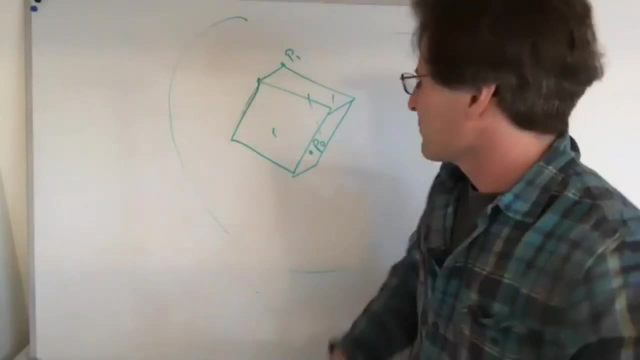 it when it first hits. that's going to be the point that's farthest away and, if you think about it, this thing's going to hit at a vertex. So this isn't so interesting. no matter where you start, you end up at a vertex, and then, if you 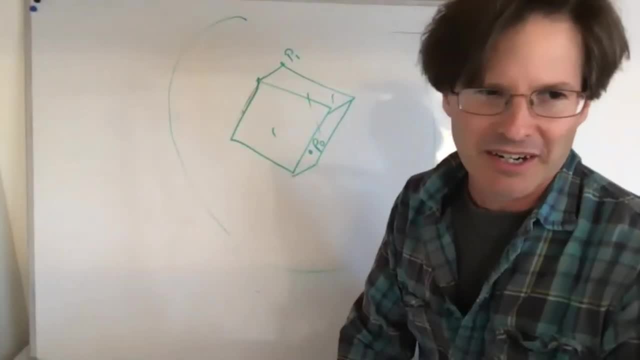 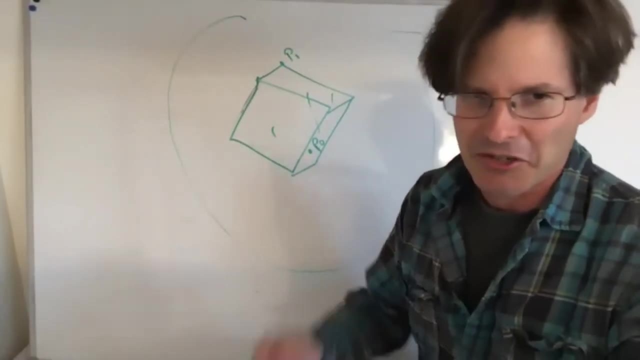 start at a vertex, you get to another one, and so on. It might be interesting, like if you had a polyhedron with many, many sides, or say in higher dimensions, and you know you could ask like which, which vertices do you hit? and you know it's. 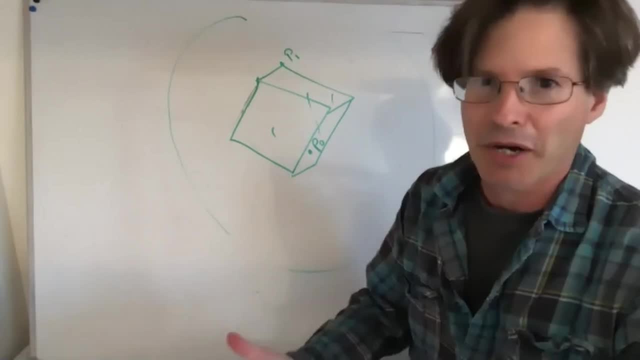 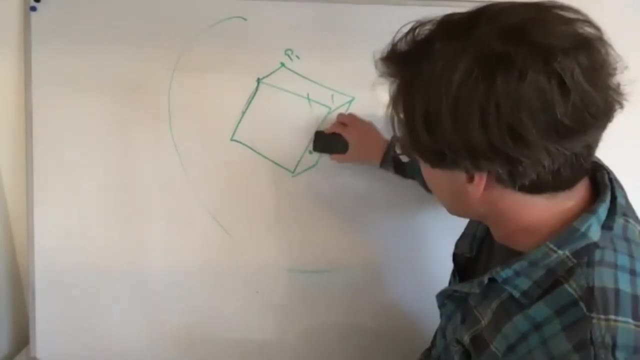 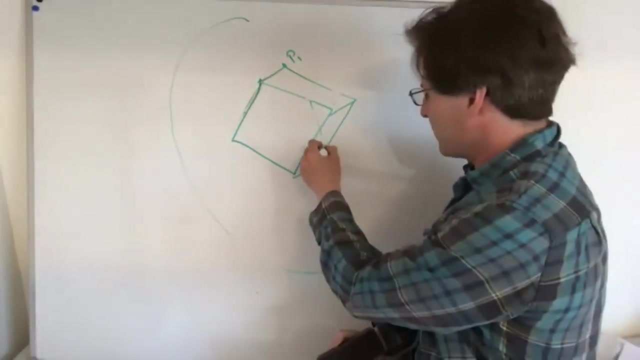 sort of a combinatorial problem, But that's not quite what I'm going to talk about. There's, there's another way to meant to measure distances on, on the, say, the surface of a cube or really any polyhedron, and what you do is you, you look at, you, look at. 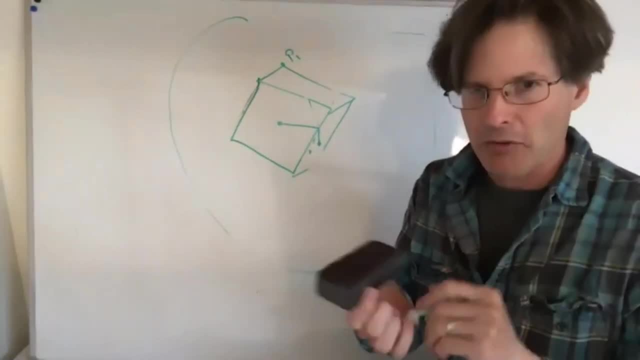 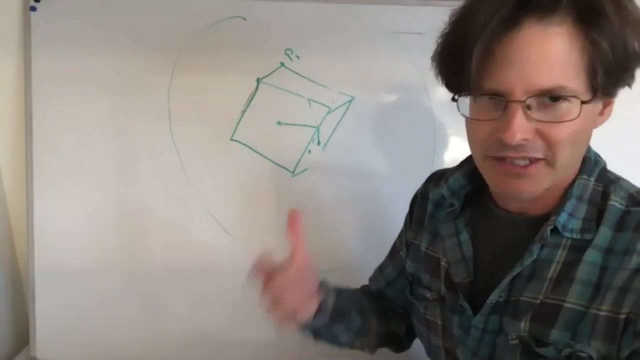 paths on the cube that stay on the surface, and then you, you take the minimum length of all the paths that join two points and you call that the intrinsic distance between the points. So so this way of measuring distances is is like you know what would happen if 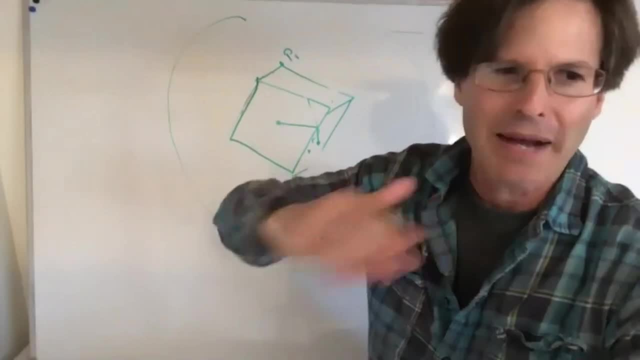 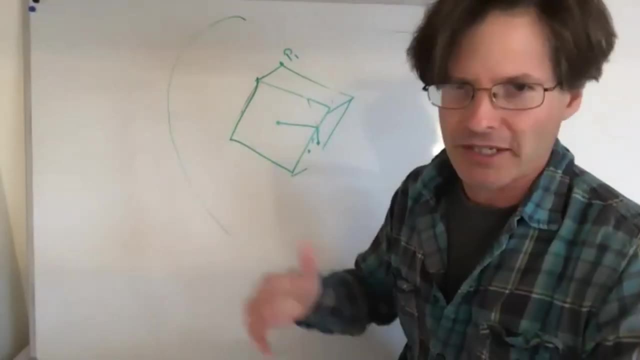 you were sort of like a, like a two-dimensional creature that was trapped on the surface. And then then it turns out it's it's no longer true that the farthest point, say, for a cube or some other polyhedron is, is a vertex. it. 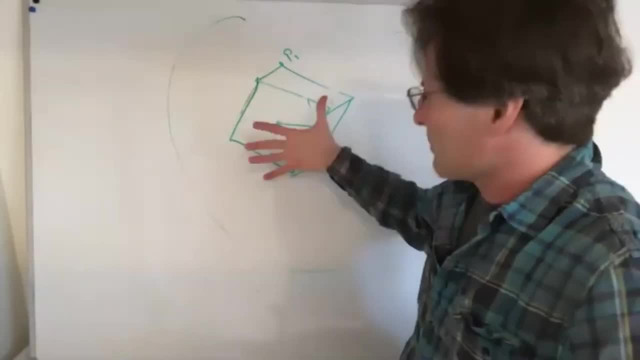 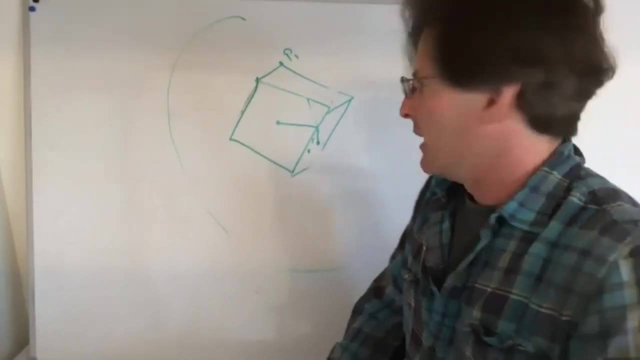 it's going to be more complicated. So this is the problem I'm going to talk about and I'm really going to focus on the, the regular octahedron. So maybe I'll tell a little, maybe say a few minutes about you know how, how I got. 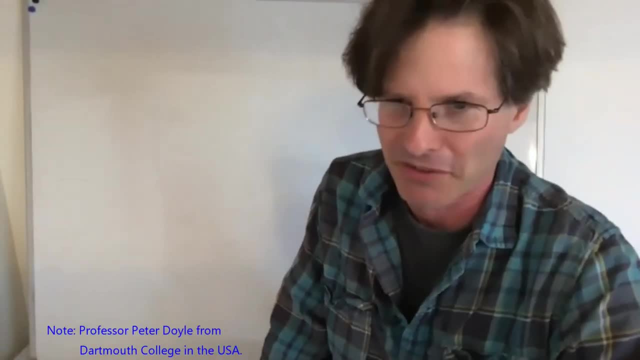 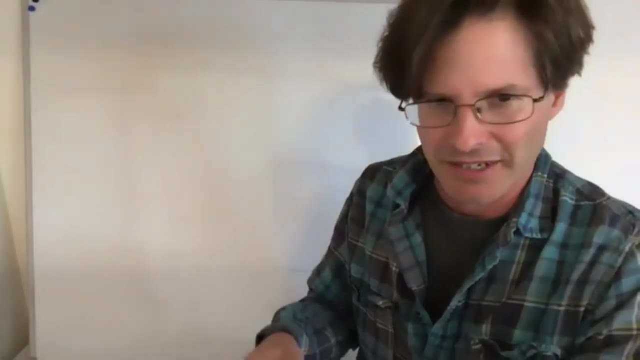 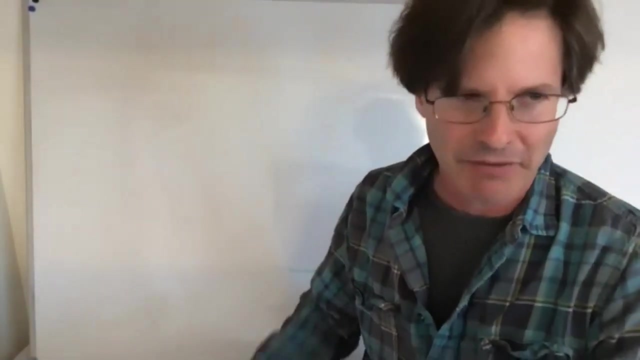 interested in this. I mean, I learned about this problem from my friend Peter Doyle, who's a professor at Dartmouth College, and Peter had had an undergraduate student working on this named Annie Laurie Maas-Pugh, and Annie Laurie had had written some stuff about this for an honors thesis, but never. 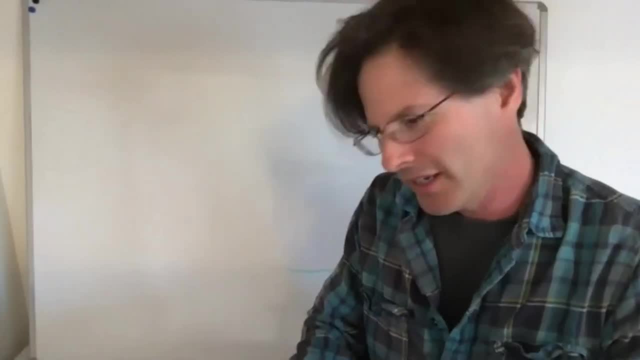 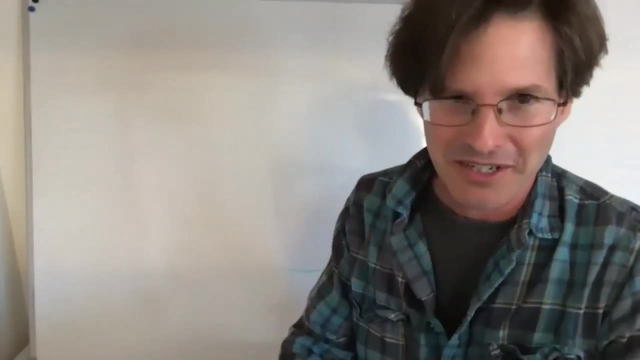 never really solved it, just sort of made some partial progress. and then, some years after she graduated, I said: well, you know, Peter, you should really like use the computer to try to understand this thing. So so in the end, what I, what I did, was I did a bunch of computer experiments and and finally figured out what was going. 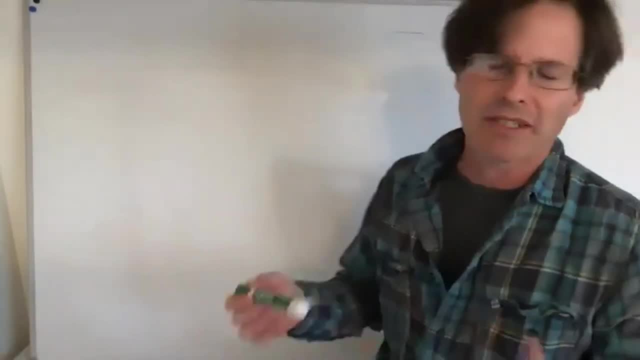 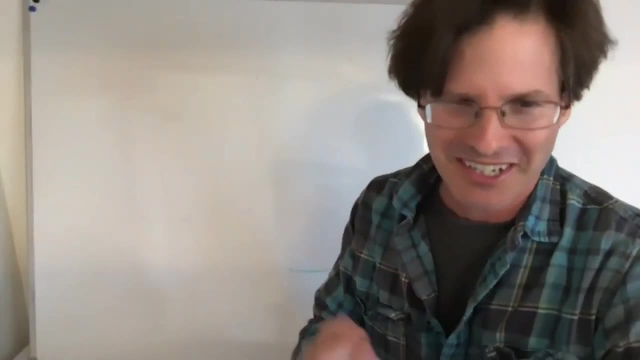 on. So maybe, before I say what's going on, I want to talk about, like, what's the nature of the computer experiments, because there's like this one technique which I've used like 50,000 times. it's sort of the only thing I know, but it's. 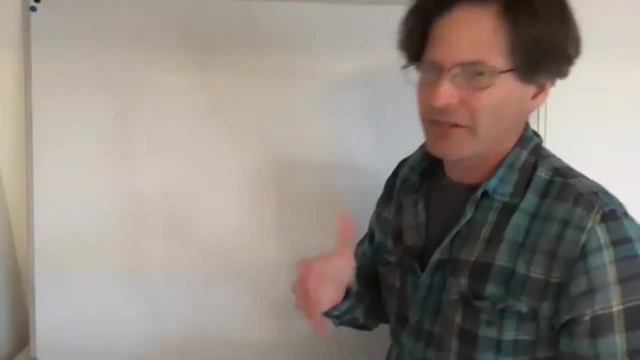 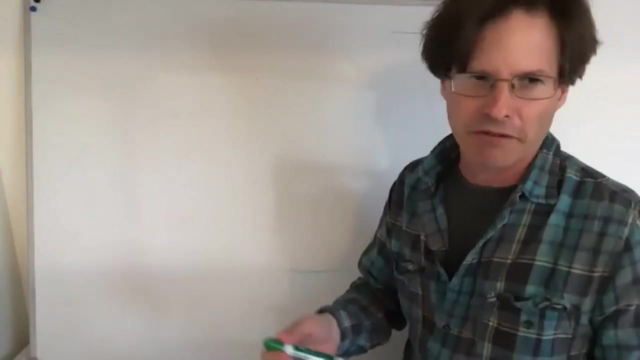 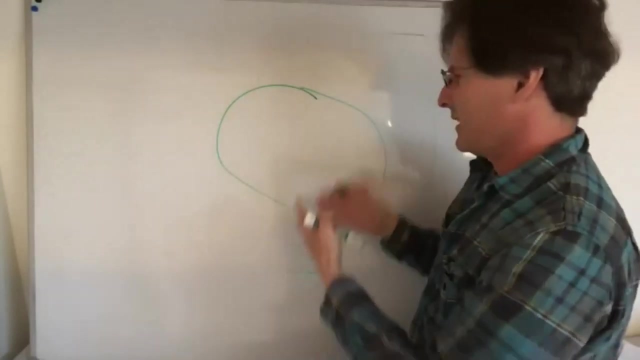 worth knowing. There's something called- people sometimes call this like a hill climbing algorithm or something like that. Some people it's also sometimes called like stochastic gradient flow. What it is is: you, you've got some function, you've got some some space. you know, in my case, 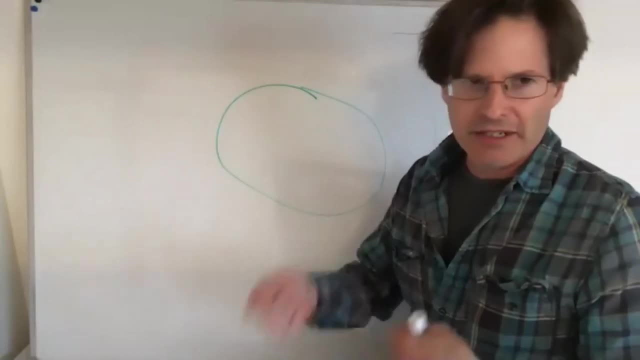 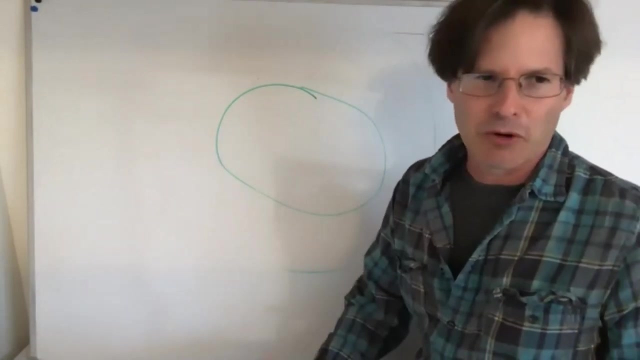 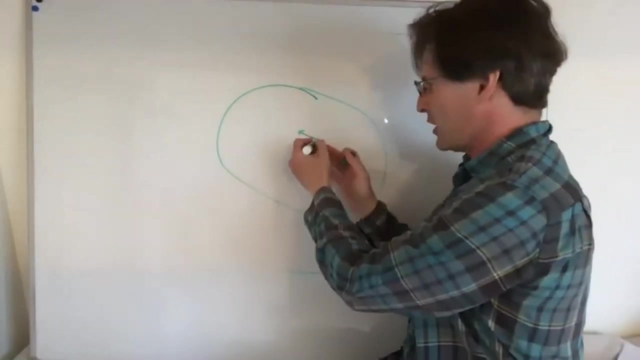 it would be like the regular octahedron and you've got some function on it and you want to maximize this function. and the question is: what do you do if you don't know anything more than the function? One sophisticated thing you could try to do is you could try to compute the gradient of the function and 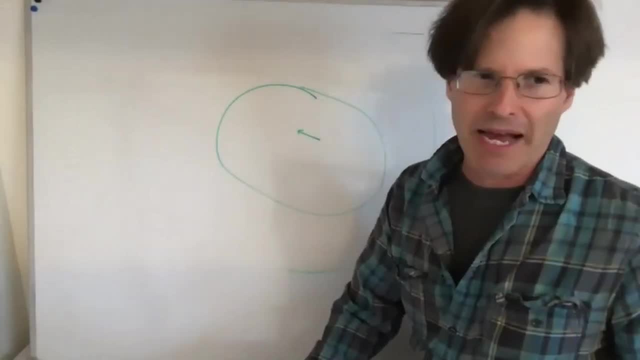 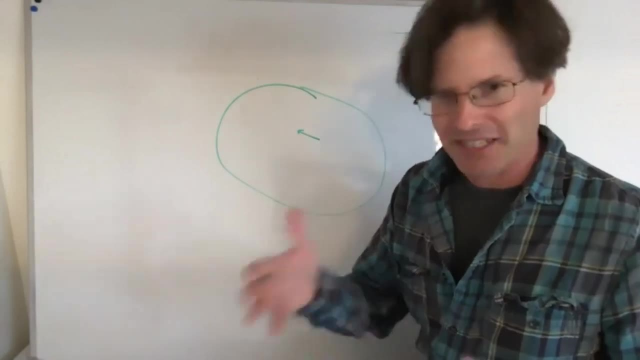 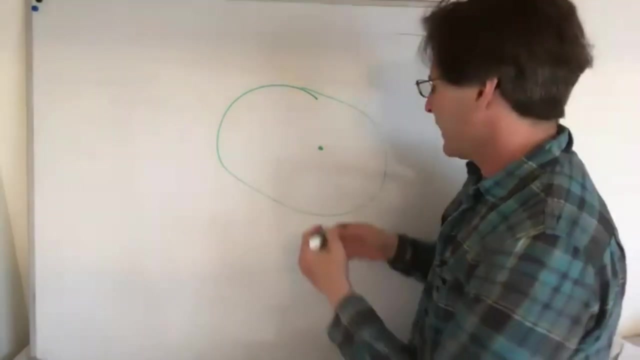 move along the gradient and this would take you towards a max, or at least a local max. but you know what do you do if you're too lazy even to compute the gradient, or maybe it's not a smooth function, it's just a continuous function. So what you do is you just randomly pick a point and then you you kind of send. 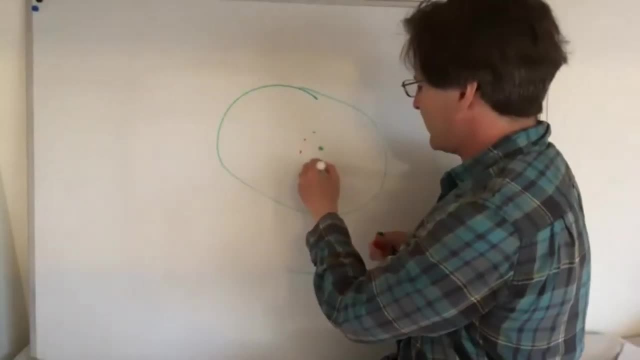 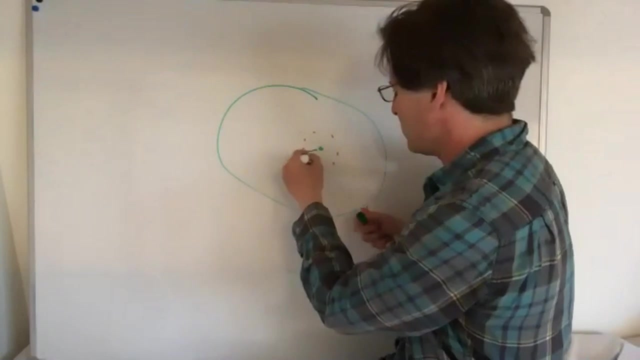 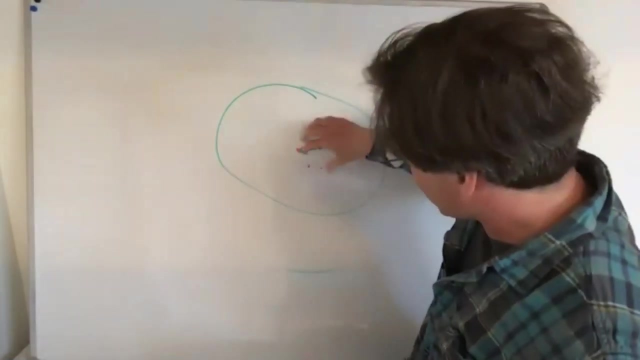 out scouts and you, you pick kind of nearby neighboring points and if, if you can find a point where the function is is higher, you just move to the new point and then you repeat and the the art in doing this is so just sort of telling, deciding like how far you move out. so so the idea is 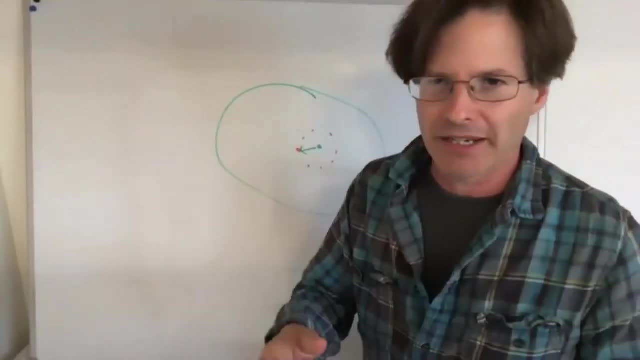 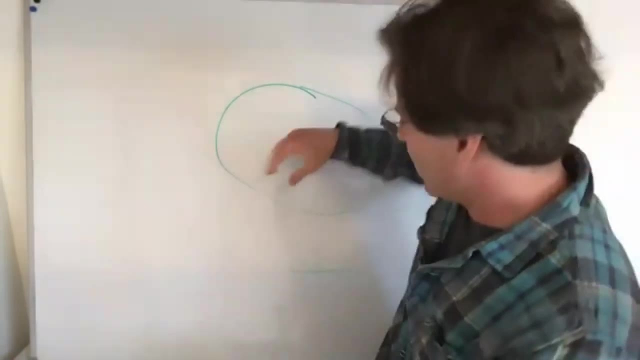 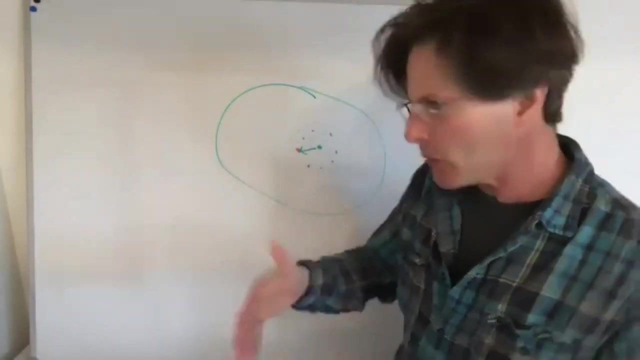 like you know, usually you should just move out a little bit and then occasionally you should take a big jump to avoid getting stuck in some kind of local well. So you know, you, you make some kind of, with some probability you move out like one half and, with some probability, one quarter and one eighth. 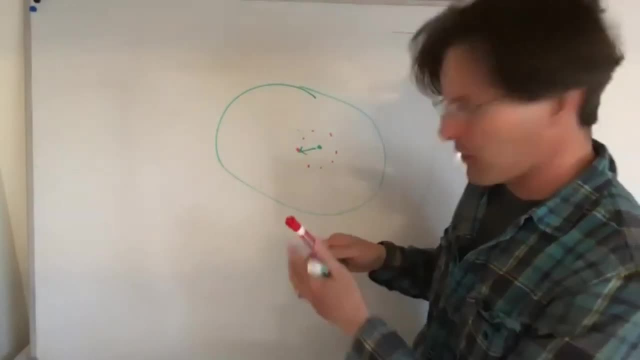 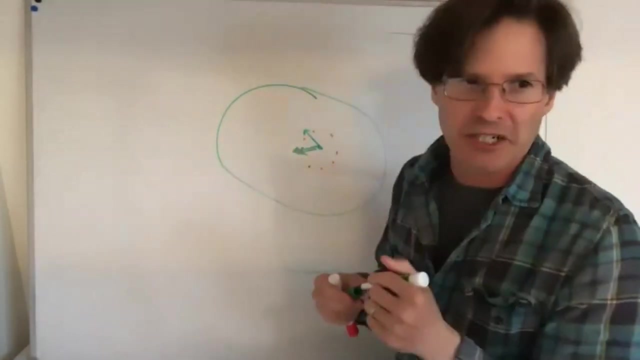 and what's really good about this thing is that if there was a gradient, if the function had a gradient, then you know, 50% of the time you're sort of moving in the direction of the gradient anyway. so, even though this thing doesn't know what, 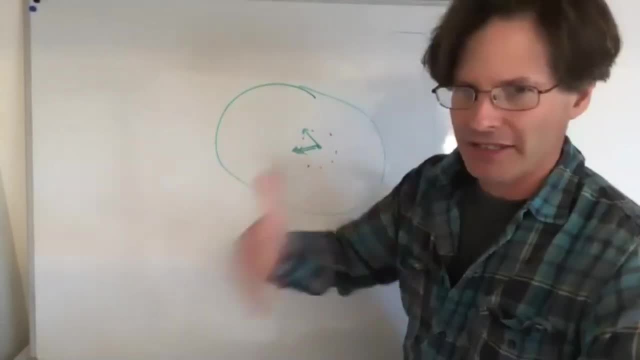 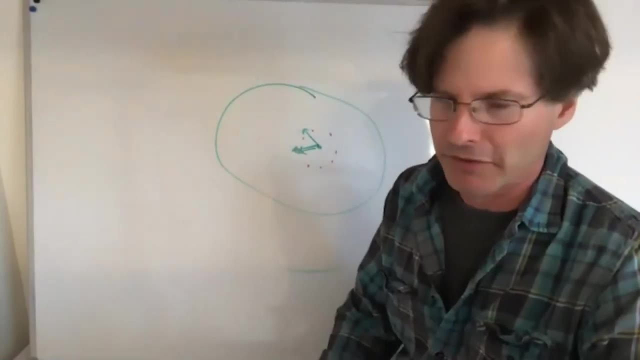 the gradient? is it actually more or less? by just accepting the things that you know that increase the function, this thing sort of simulates gradient flow and if you run it on a computer it actually looks a lot like gradient flow if you take small steps. So any other questions? 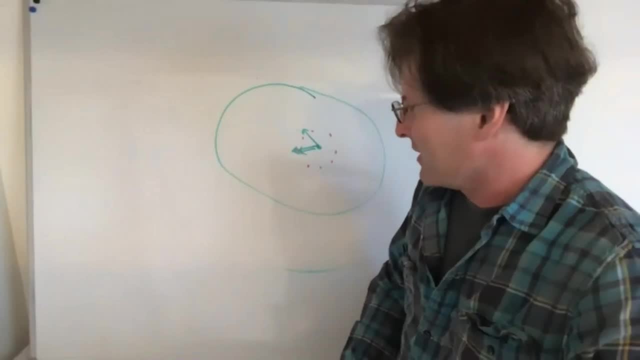 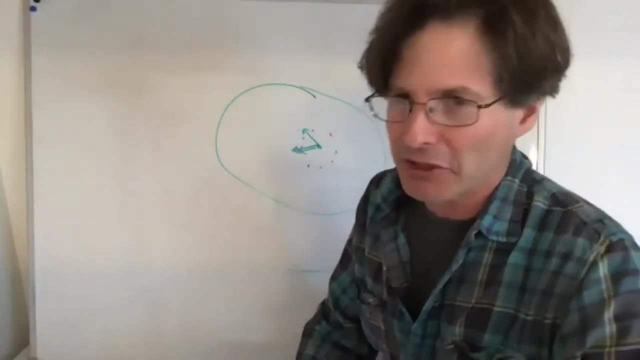 Any other questions? So anyway, when I got interested in this problem, I just made a program that draws the regular octahedron and and then does this process and I sort of right after looking at this thing for a long time, I, you know, I figured out what was going on. 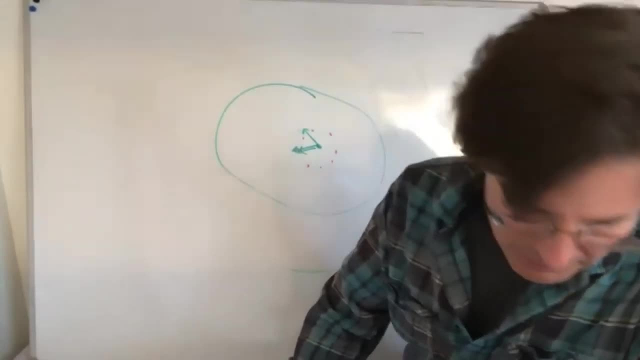 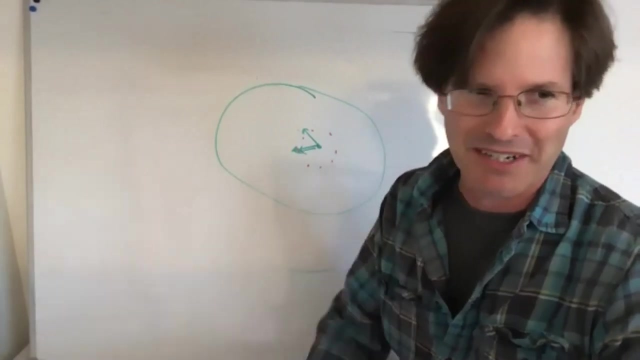 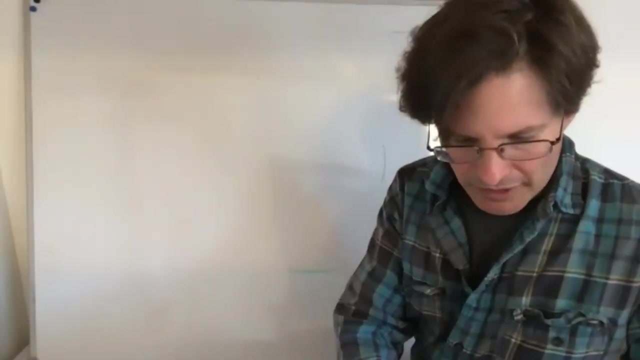 So anyway, that's the experiment. I mentioned this just because, if you ever have some problem like this, some kind of optimization problem, I recommend hill climbing as an experimental method for figuring out what the thing does. So now we're on the, on the regular octahedron. I want to talk a little bit about this intrinsic. 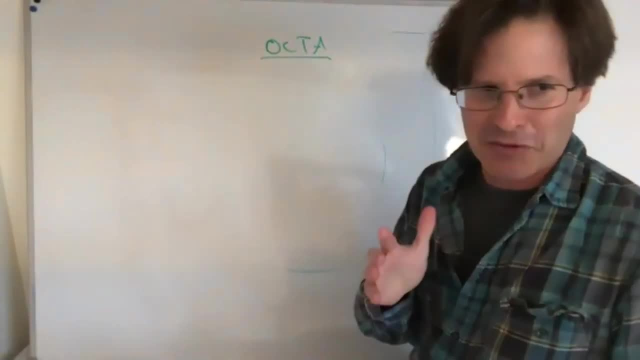 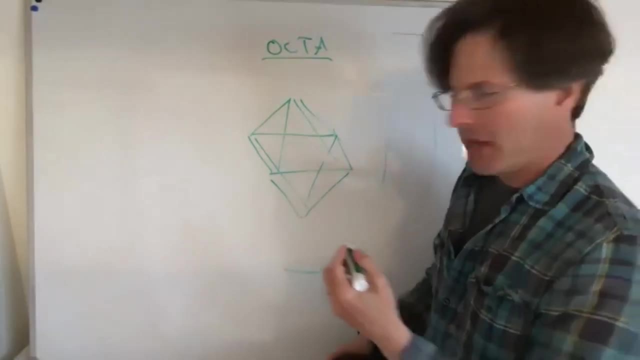 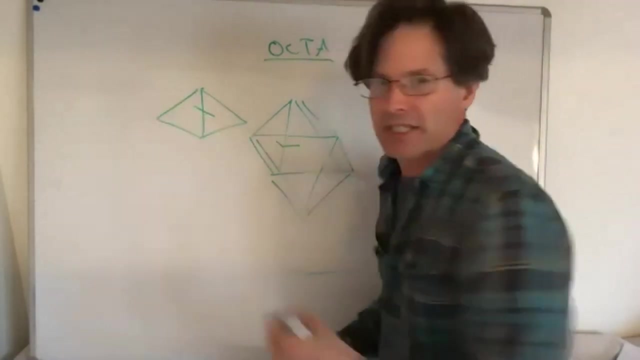 distance it's. if you haven't thought about this before, it's. it's really a weird and amazing thing. okay, so that that's an octahedron, more or less, and what's amazing about the intrinsic metric is that if you go over an edge, it's completely indistinguishable from two equilateral triangles. just sitting. 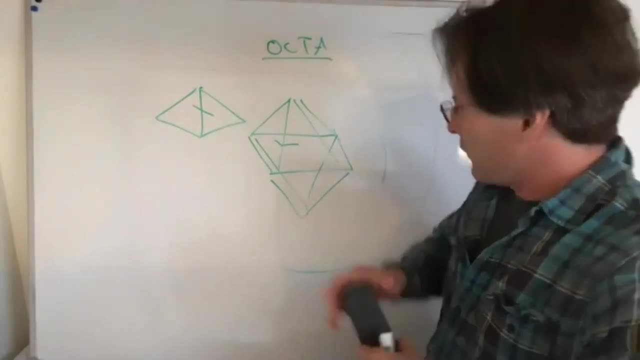 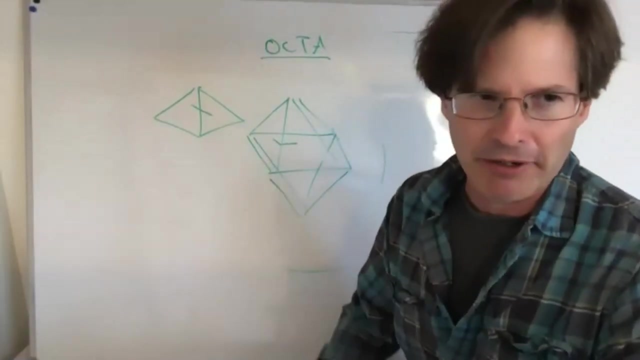 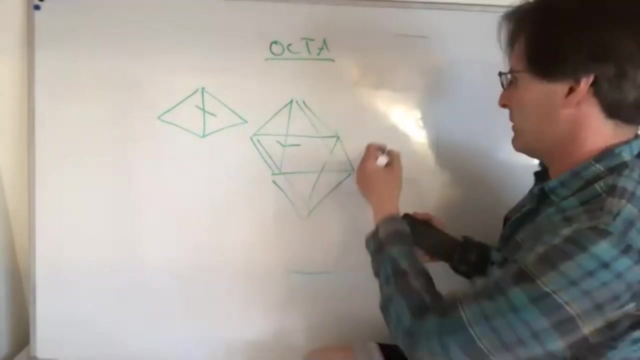 in the plane intrinsically. So if you were a creature embedded in this surface, you would think that the thing was completely flat like a piece of paper, except for the six cone points. and the six cone points. you don't even see the edges around them. in fact, like you would sort of think you were something like on. 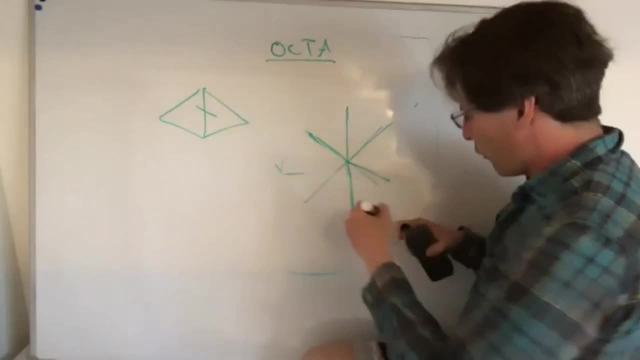 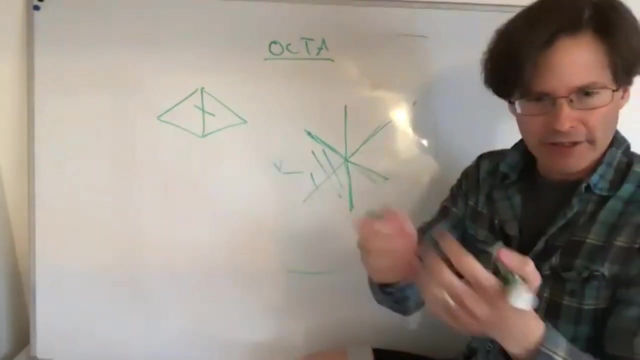 a like. what it would look like is you would take like four equilateral triangles and stick them together and then you you'd cut this stuff out of the board and then you'd glue it together. this would this would make like a like an ice cream cone. So somehow the the regular octahedron are. 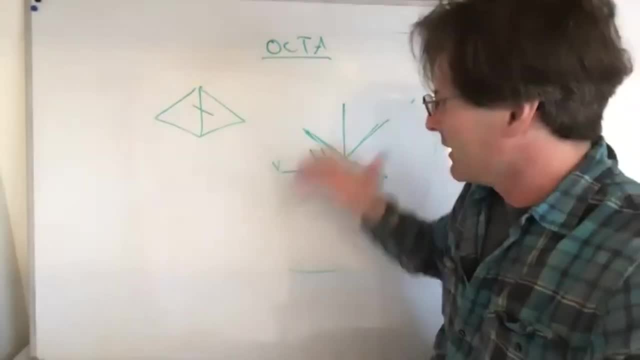 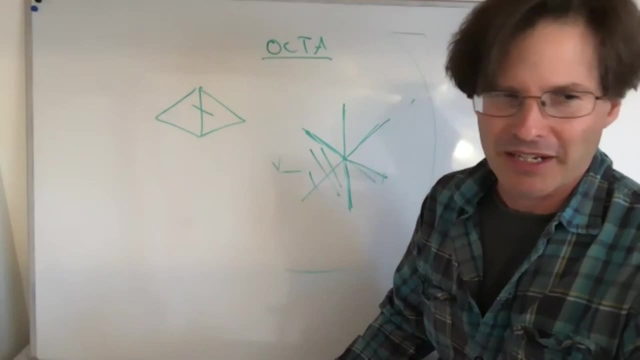 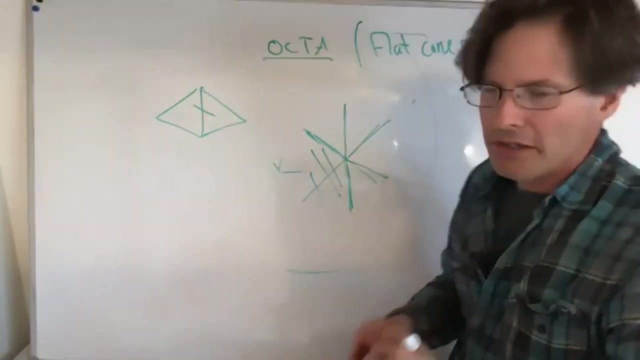 really any, any polyhedron with its intrinsic metric it's. it's flat everywhere, except for a finite number of points where it looks like an ice cream cone. So so that that's a pretty neat thing. These things are sometimes called flat cone surfaces. So any questions so far. 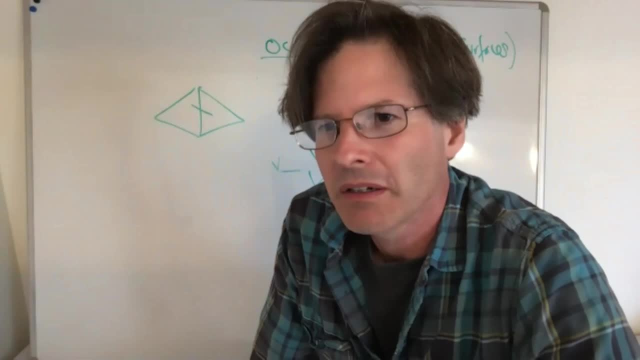 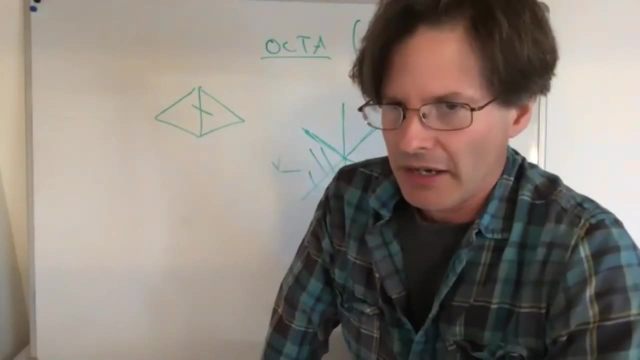 Do we need to include anything else, but just which edges we cut off on the way? Because for no, no, no, that's that's. that's a great observation. If it just is combinatorially counting, which combination of edges are we going, or is there anything? 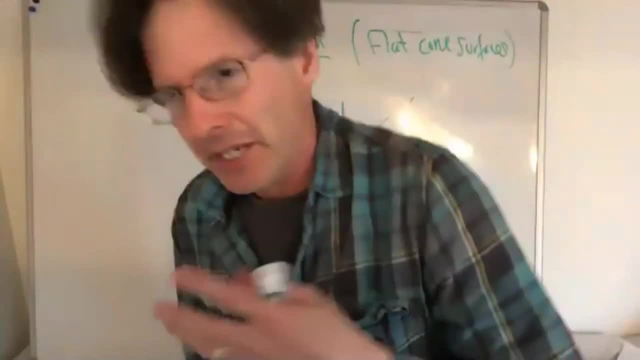 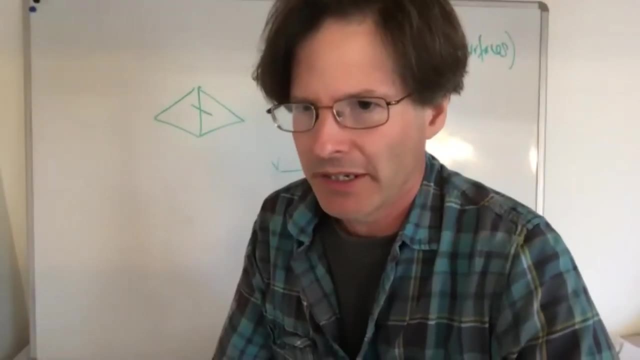 Yeah, well, I mean it's, it's a mixture. okay, so it's a. it's a mixture of combinatorics and geometry, because you might be able to get get round to the same point in several different directions, and- and I'm gonna, I'm gonna talk more about that in a little bit- So, so there might be, you know, for example, 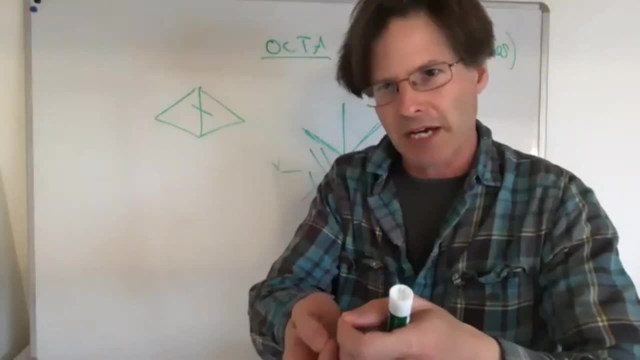 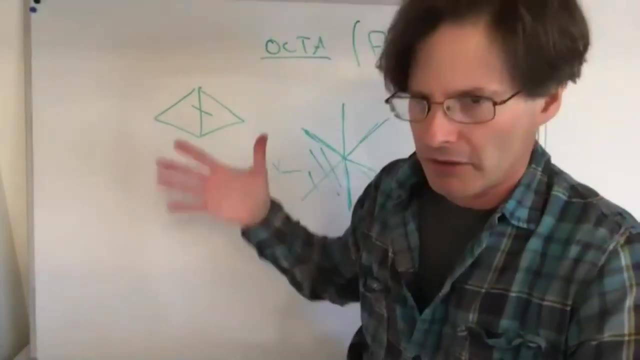 like if you think about the surface of a sphere and you're going from, say, the North Pole to the South Pole, there's there's many different ways you can get there that have exactly the same length and and on something like like a regular octahedron. that that's also gonna happen. I'm gonna draw pictures of. 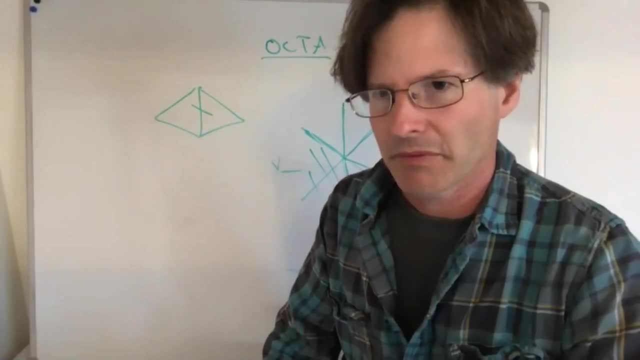 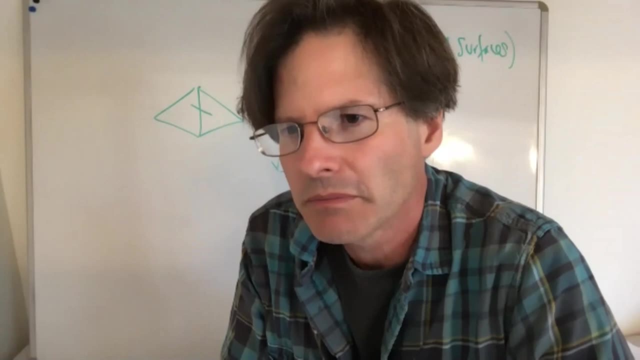 this in a little bit. Yeah, perhaps I can quickly paraphrase. Sorry to interrupt so early. Are the two paths that are both length minimizing but go through the exact same sequence of edges. No, right, once you keep track of some sequence of edges, you. 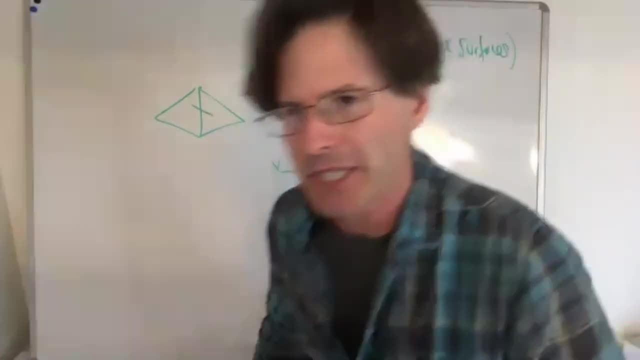 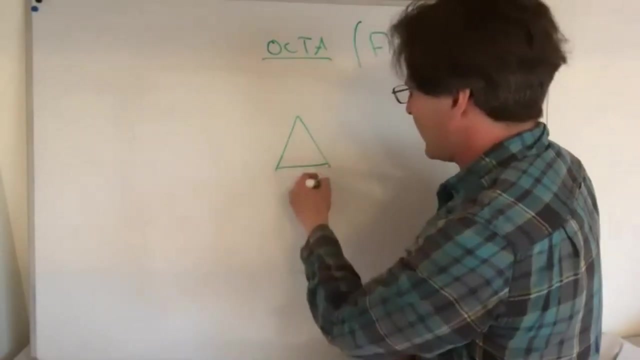 could then say: well, how do I actually get to the point? So this this brings up like: so there's a nice calculational tool for this, and people call it the unfolding map. You could do this for any polyhedron, but it's especially nice for the, for the regular octahedron. What you do is you imagine: 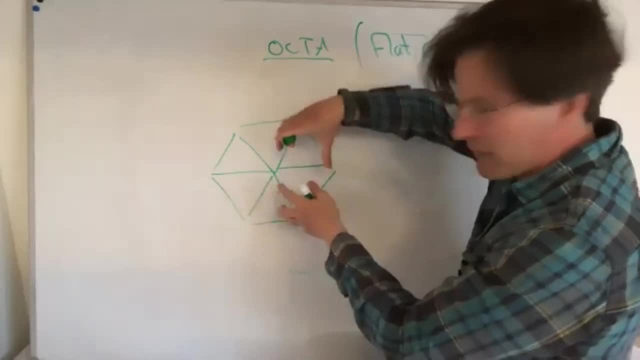 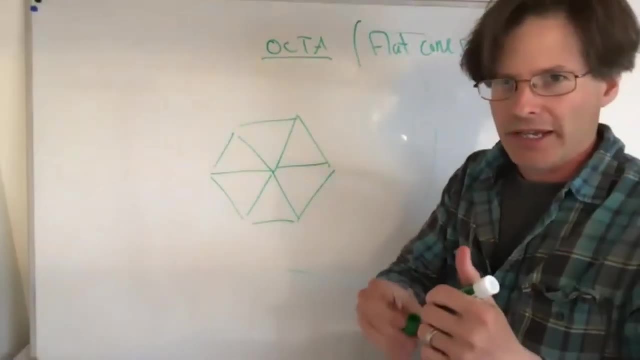 that the octahedron is is like sitting on one of these triangles and then you, you just kind of roll it around to the, to the next one and the next one, And this, this process is, is a little bit vague the way I'm saying it, Like you. 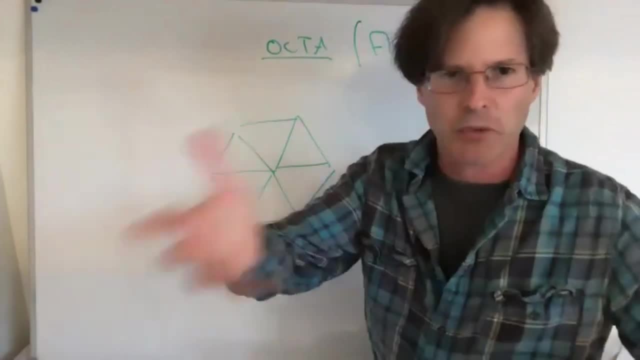 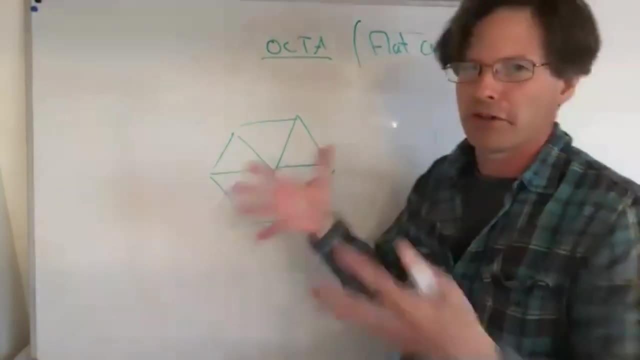 could just say: you take the thing and you start rolling it every which way, and if you've learned about this in an algebraic topology class, I'll tell you that the right thing to do is: you take, that, you remove the vertices, you take the universal cover and then you, you roll the universal cover around into the. 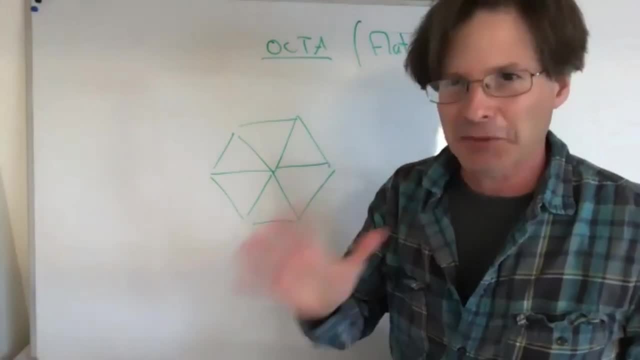 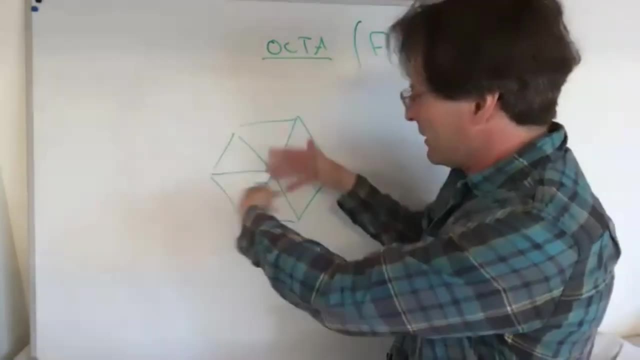 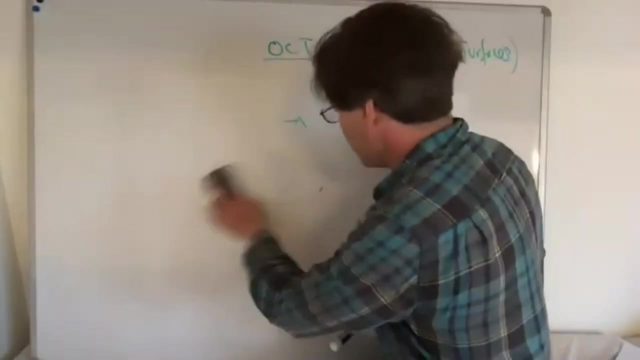 plane. But if you haven't had an algebraic topology class and you don't know what the universal cover is, just forget about what I said, because you're only looking for, kind of you know, get paths that go all the way around, so you don't really have to roll that much of it. Really, what you, what you do, is you. 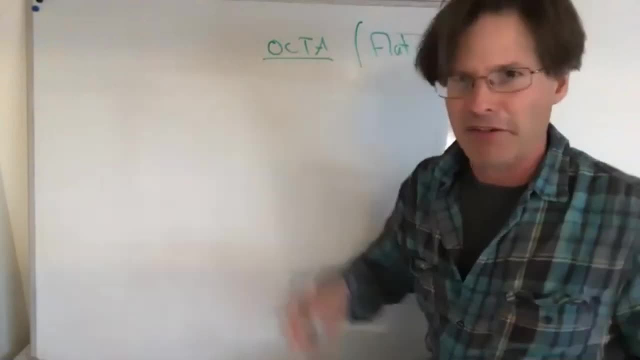 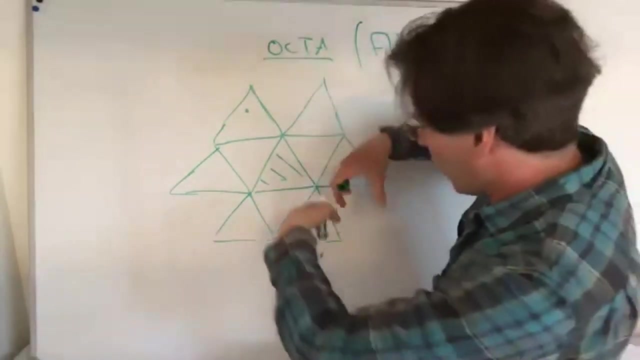 kind of draw, a sort of what I'll call the playing field, So this one's sort of the home base. Well, there are two ways to think about it. You roll the octahedron out into this thing, but then you can also roll this thing back up onto the. 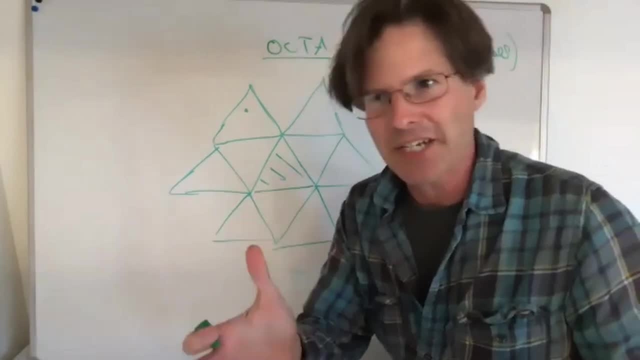 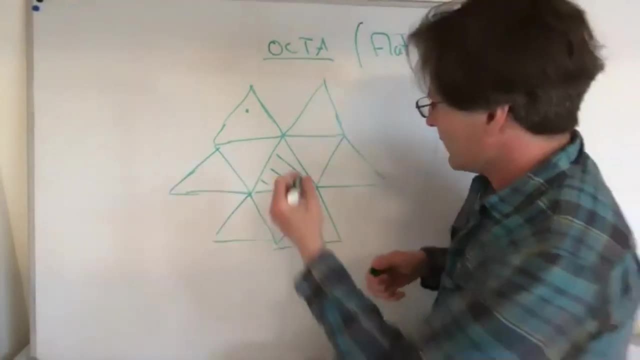 octahedron. The way to think about this is like you have an octahedron and it's a present for somebody and here's your wrapping paper and you just go like this And there's a little aid to figure this out, like there's a coloring of the vertices. 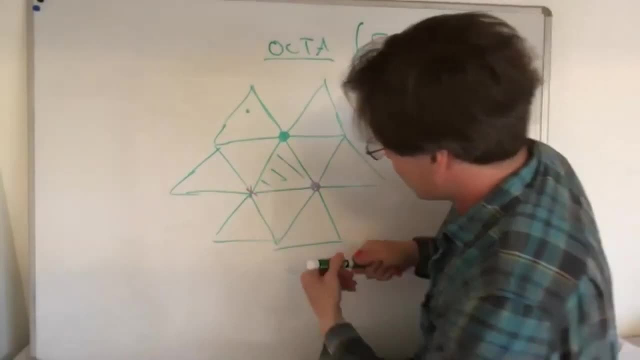 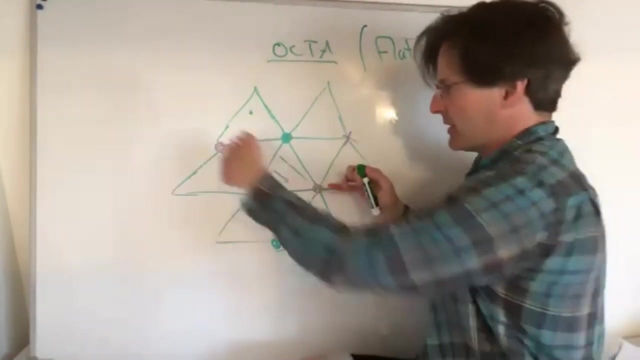 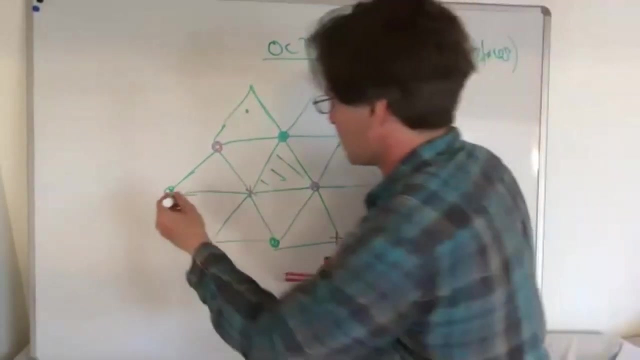 Say black, pink and X and the coloring you propagate it by. whatever the color is here, it's the same across from it. So I think I said black, but I'm using green, so so maybe let me switch to black. Okay, there you go. so each, each vertex is: 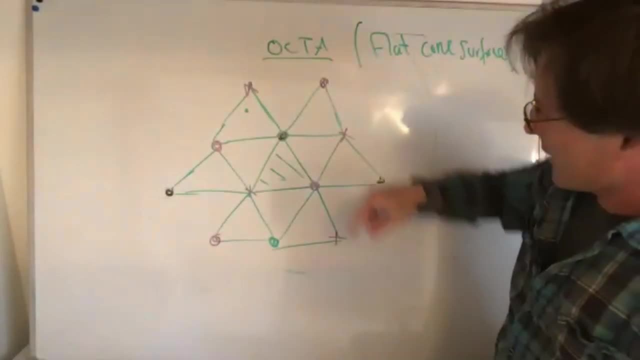 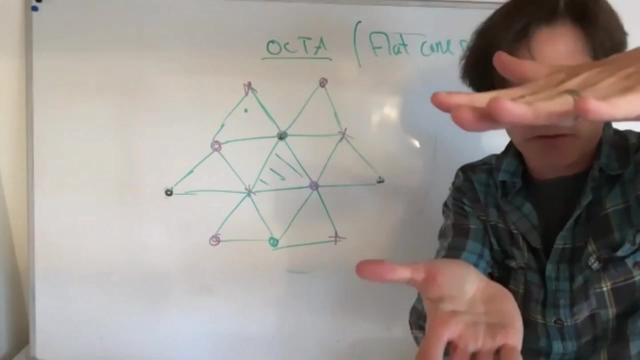 colored, one of three colors, and the idea is that so there's sort of a one face of the of the octahedron, and then there's another face which is on the other side, which is called the octahedron, And then there's the other face which is the antipodal face, and and all of these. 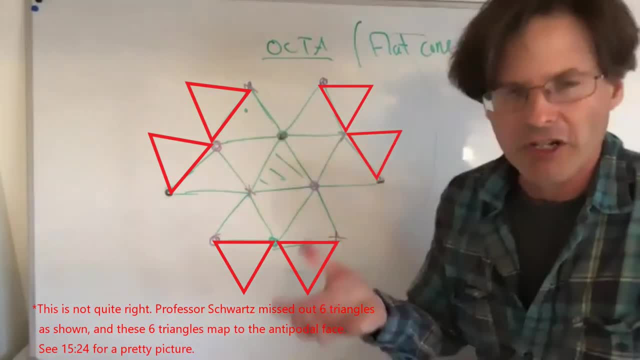 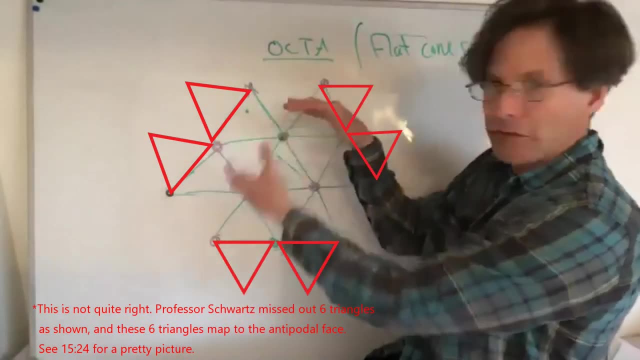 six regions. they all go to the, they all wrap up to the antipodal face. so so you have to sort of picture this thing just kind of sitting above this, and then when you, when you fold it up, it just you just all these six of them close up and the. 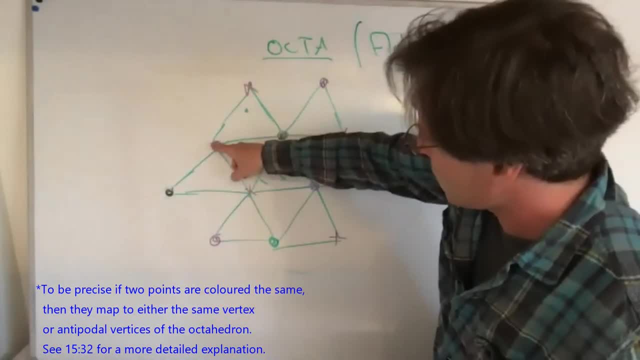 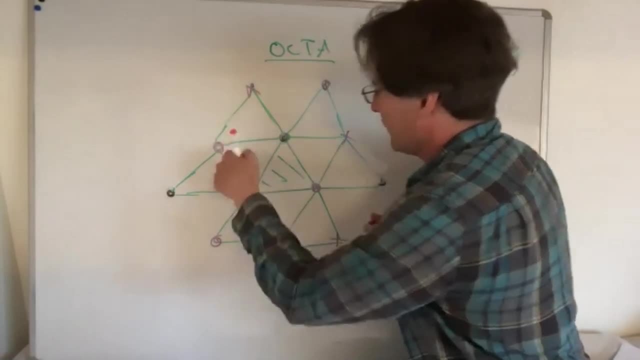 colors indicate where the vertices go, so that, like like, this point here goes to the same place as this point here. So if I have a point over here, like right here, which is sort of fairly near the pink, it's the same as this point over here. 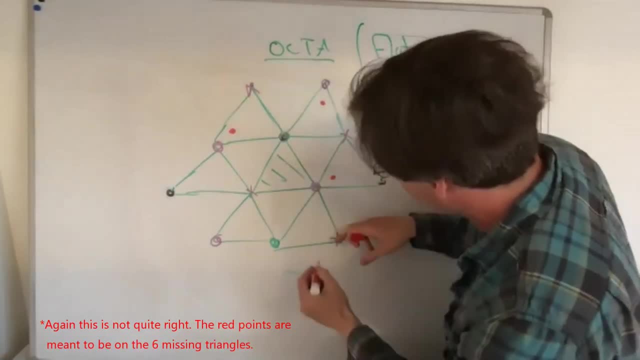 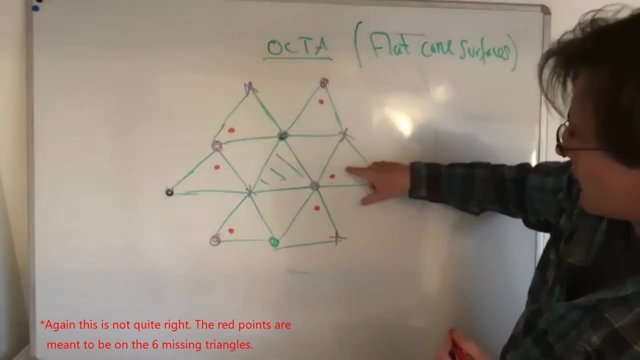 and also it's the same as this point over here, and the same as this point over here, and this point over here and this point over here. so so all of these six points I've drawn, they're in the same position with when I fold it up. 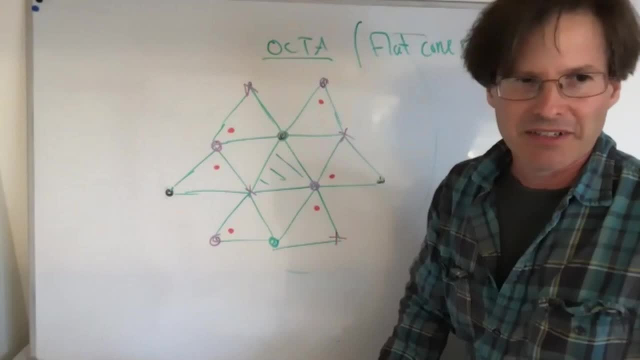 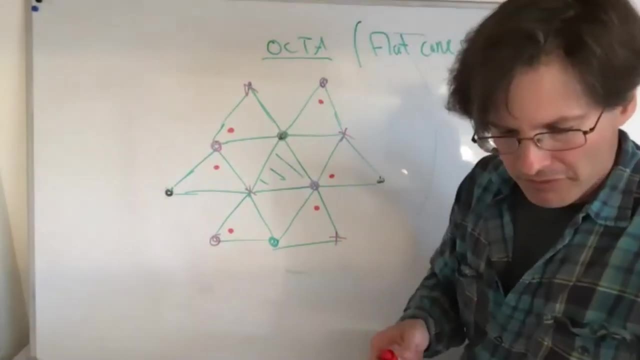 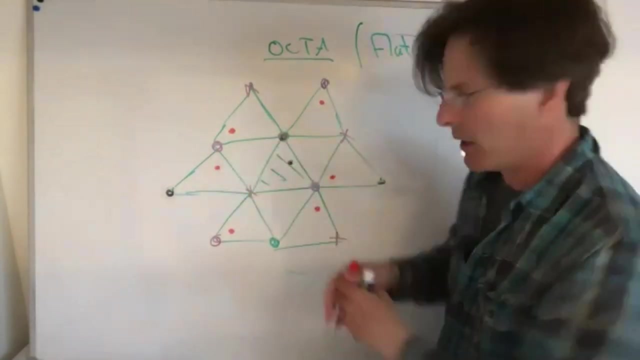 they all these red points go to the same point. so so this sets up like what you could call a competition, Like you know, you, you have, you have some point here and you want to know, like, how far is it to this red point? well, you, you know the red points on the other face. 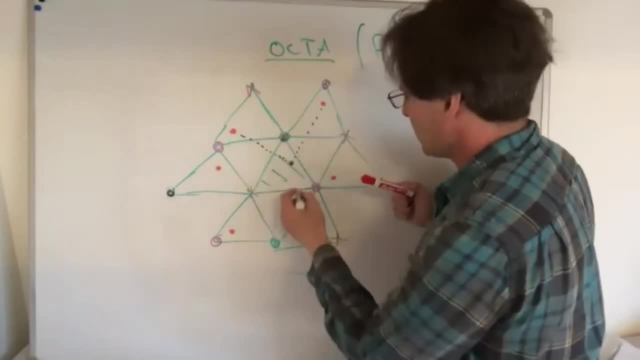 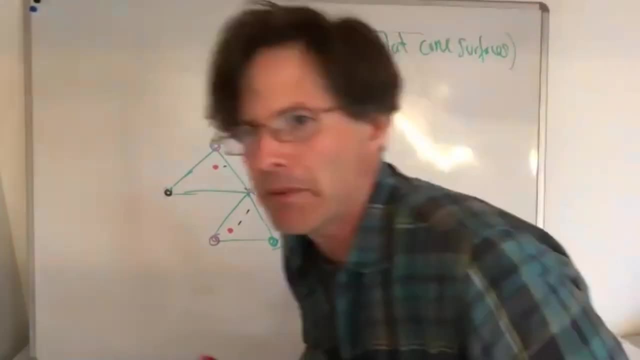 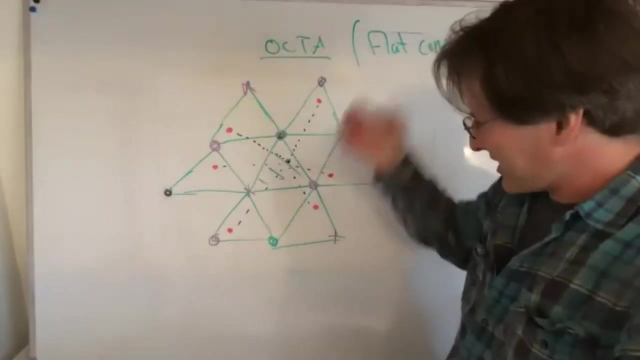 and you unroll the thing and then you, you measure these six distances and you take the shortest one. So this is maybe answering Misha's question. Yeah, thank you. In that picture it becomes very clear. Yeah, yeah, this is anyway. so this is, this is the thing, so okay. so now I'm going to tell you about a new so. 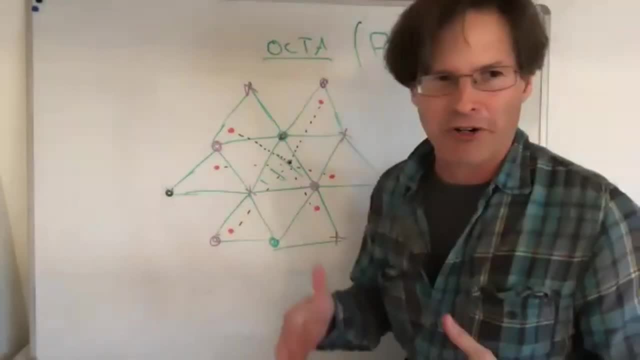 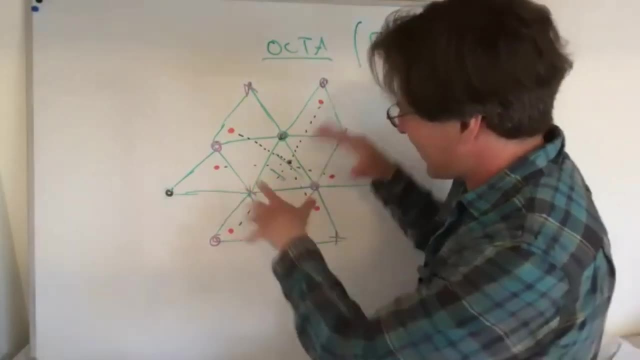 so you could imagine. so there's this. like I wrote this program which I'm going to show you in a minute, and I called it spiders embrace, and the reason for the name is that, well, it's a six-sided spider, like you've got this point and you know it reaches out to these six points and you want to measure. 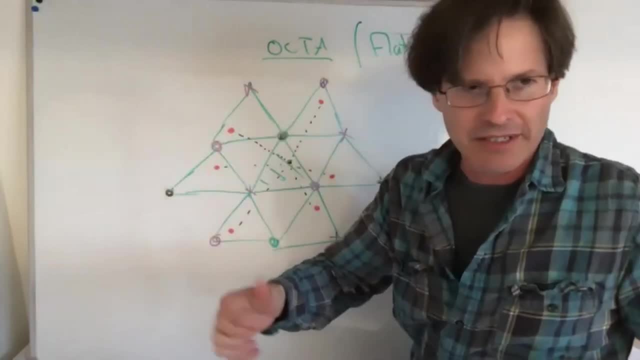 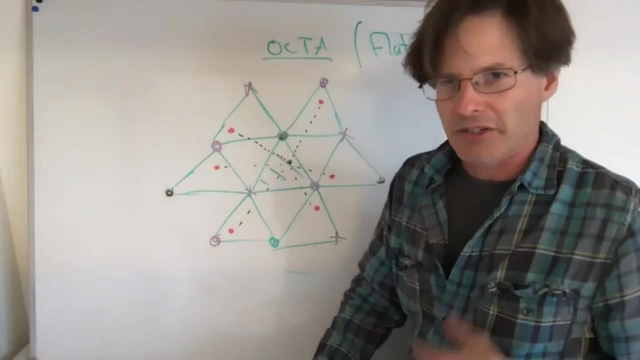 the distance. and you know, usually one of the legs is shortest and that's, that's the. you know that would be sort of the distance between the legs, Those two points, so you can use this thing to compute different distances. so now, now I'm going to tell you, there's another object in geometry which is: 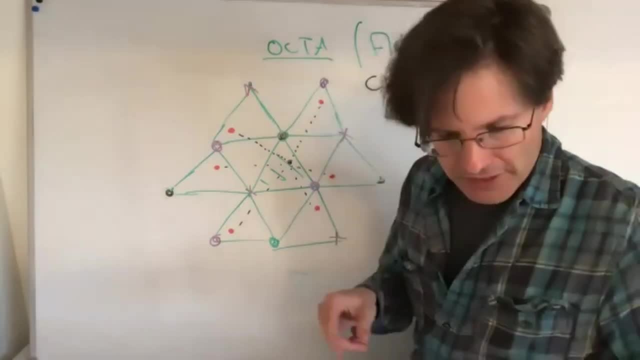 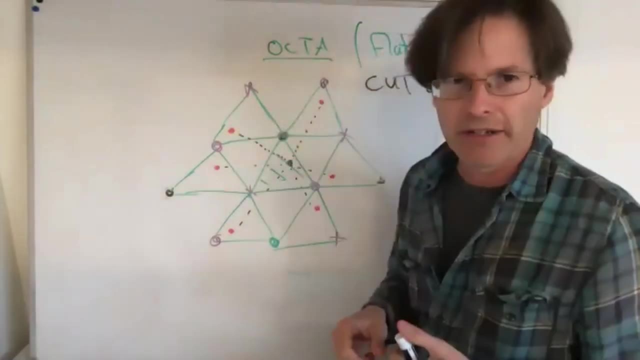 called the cut locus. it might turn out like if you fix a point, so I'm going to fix the point here and I'm going to, and I'm going to sort of look. look at, you know distances to this point. the answer would change if I move this point. but 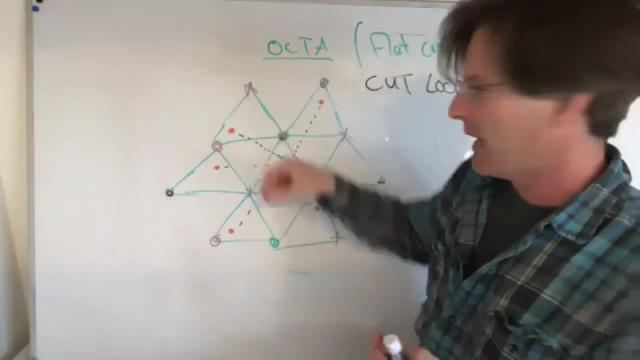 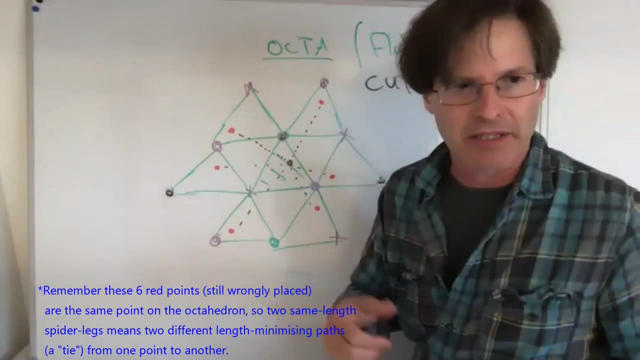 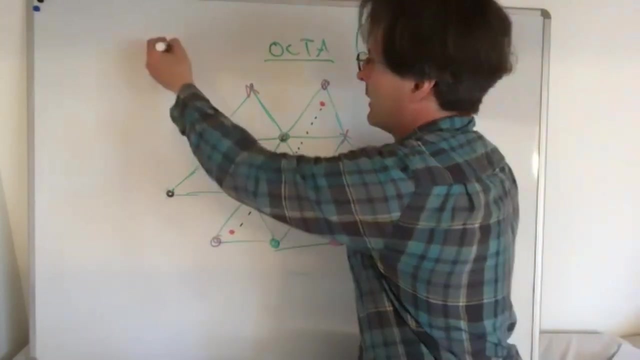 anyway, certain of these red points are going to have the property that there's more than one, more than one of these spiders legs that has exactly the same length, that reaches it and in fact, if, if some point has that property, if you think about it sort of. 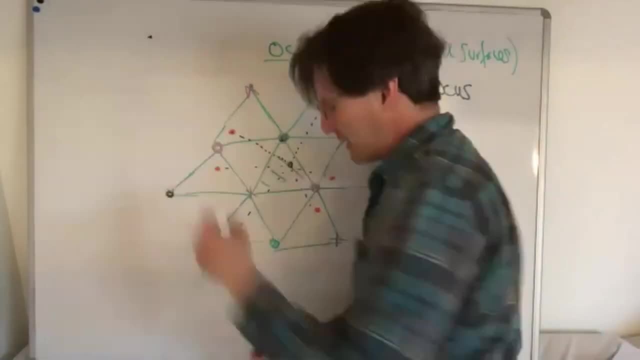 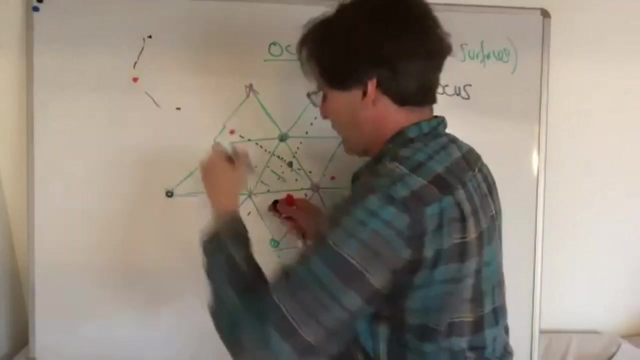 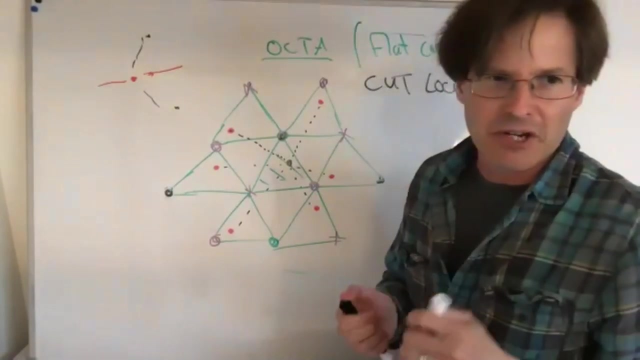 kind of abstractly. what imagine instead? your point is here and these spider legs are the same distance, then there's really kind of like a whole, a whole line of things where they're, where they're equidistant, so so in fact, if you could find a point where there's two spiders legs that are the same distance, there's a. 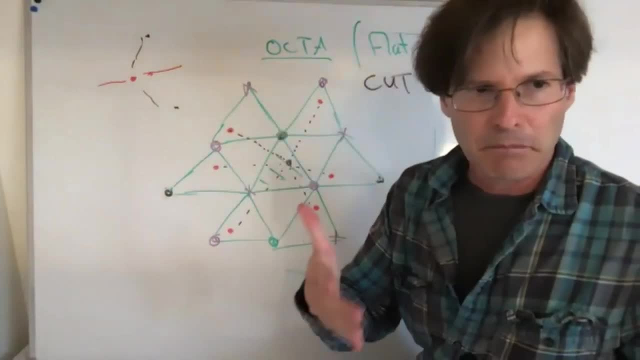 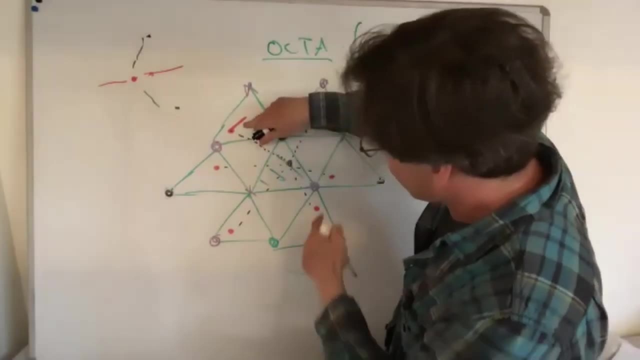 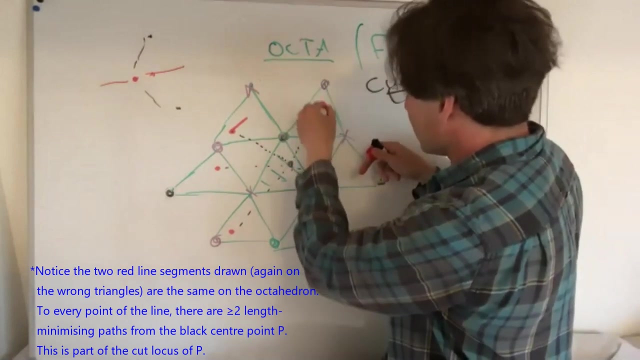 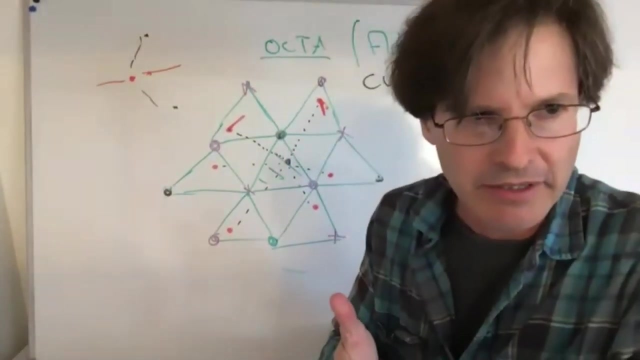 little line that that also has has that property, so so. so there's some thing like this where everything in this line say this spider leg and this spider leg. I guess it would look like this. they'd really be the same art and everything would be exactly the same. I'm going to show you guys pictures of this in a minute. 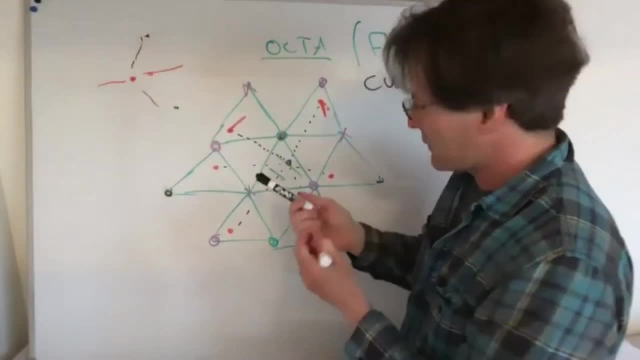 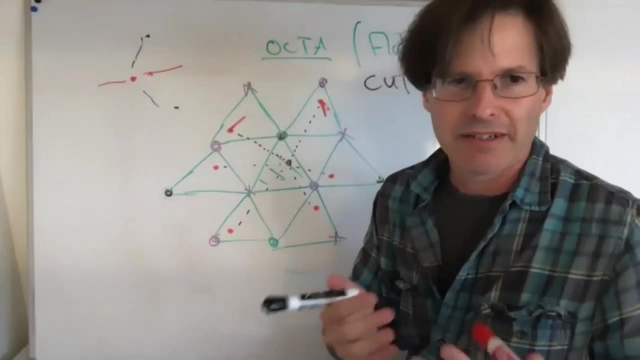 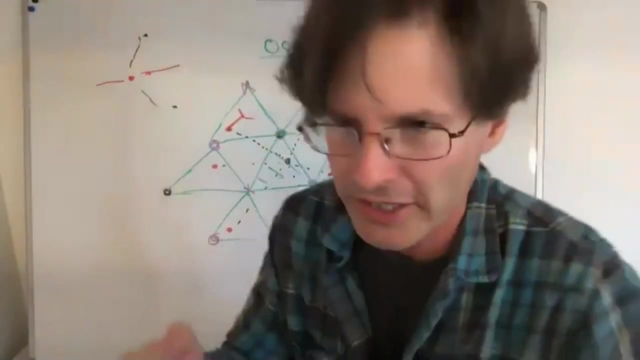 and then there's something which is even neater that happens. you've got these various kinds of red arcs, of kind of like the points where there's ties, but then there could be a three-way tie and then you would have see some picture like this. so so, actually, if you look at the set of all points where there's ties, 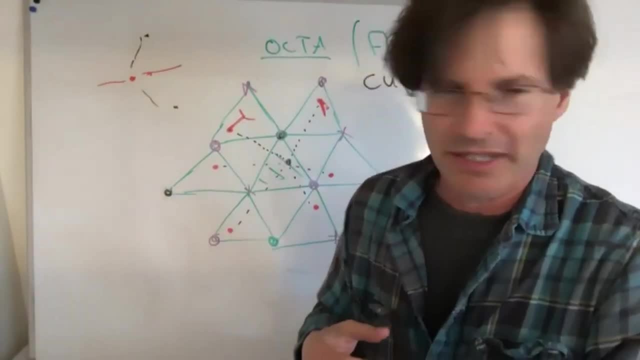 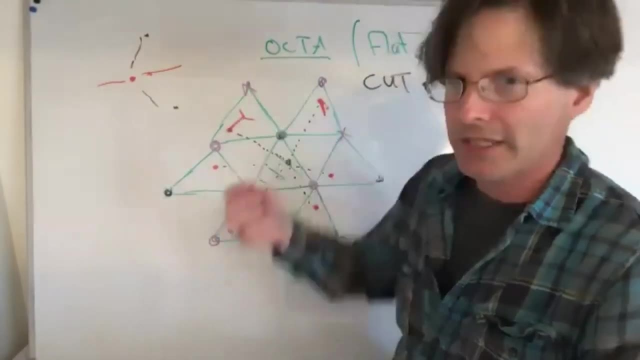 this. this object is known as the cut locus and it's a, it's a graph in the octahedron and it usually it's got this kind of like prong type singularity, but depending on which point you pick that, there might be four or more coming. 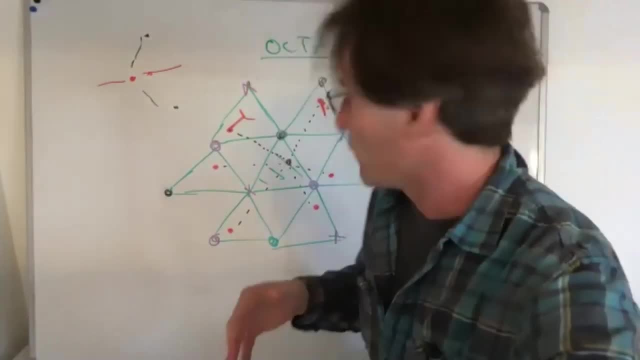 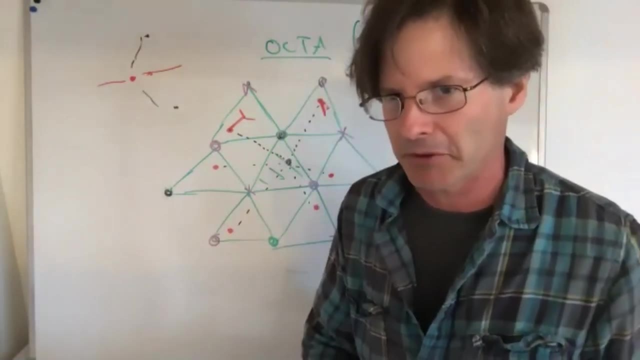 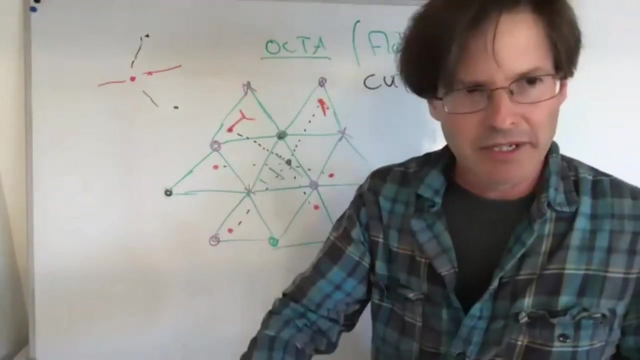 in and so, anyway, this is some kind of basic object in geometry and people often study it in when they study Riemannian geometry. like it's the same kind of thing you're looking for, like all the points where the shortest path, where there's more than one. so let me, let me share my screen with you. I'm 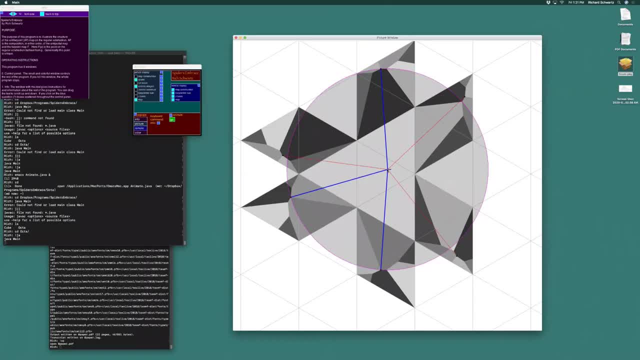 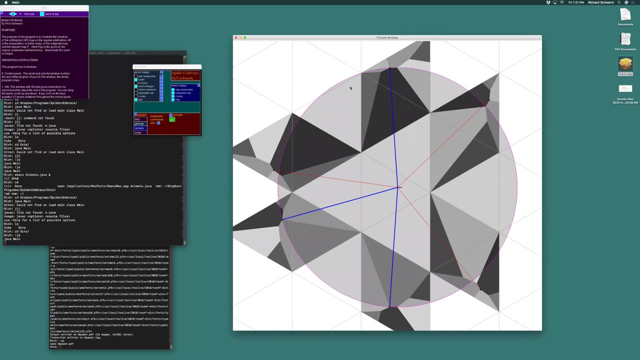 going to show you this, this program. so see, so there are these six outer outer triangles. I see a chat. let me just wondering about the diagram you drew on the board, what the colors, the colors on the vertices, represent. like there's, those aren't the same, okay, so so. so on the octahedron. the octahedron has. 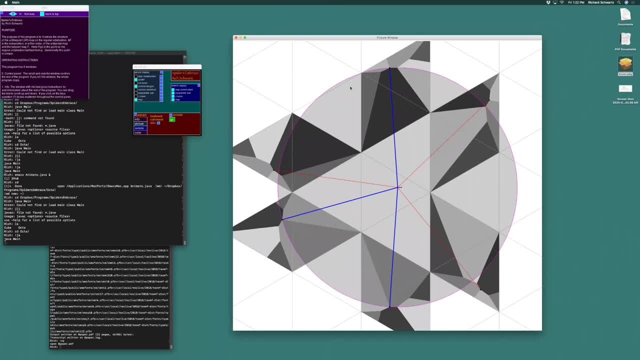 six vertices and you can color them in three colors, so that opposite vertices get the same color. okay, god, thank you. and then these colors are the ones they're like, the pre images, so to speak, under the map to the octahedron. thank you great. anyway, that's, that's how I was able to. that's how my program figures. 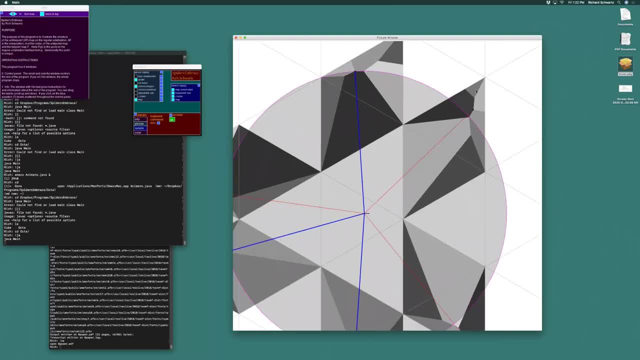 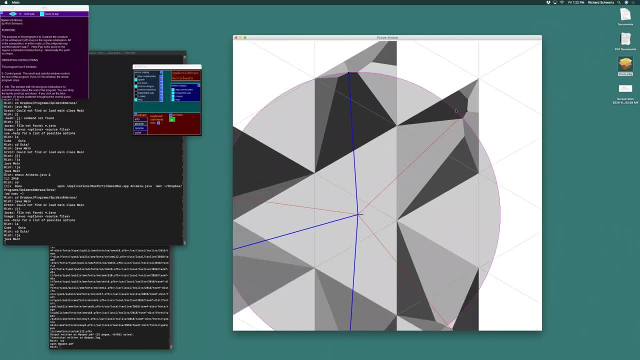 out so like. so if you look at this picture in one of these triangles, this is the cut locus with respect to the point in the middle, and if you, if you look in in the other triangles, it's, it's the same picture, it's just been rotated. 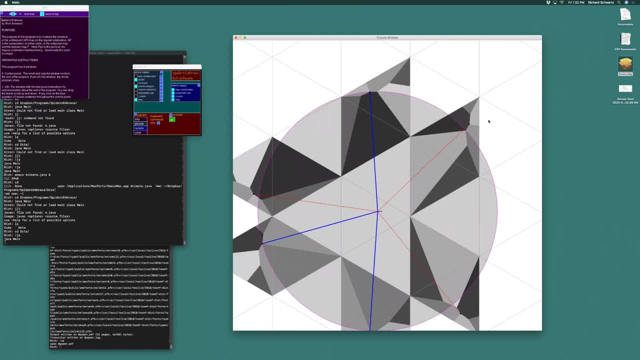 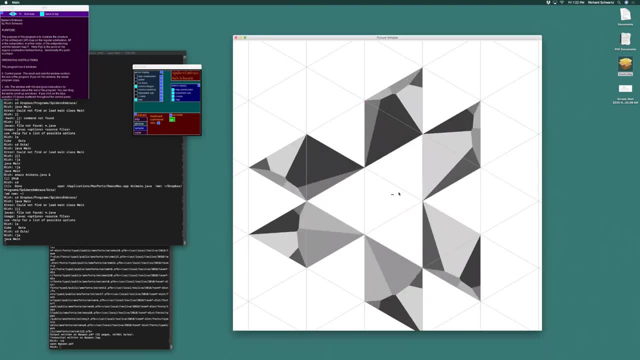 according to the coloring of the of the dots. so you can, you can sort of see: um, maybe I'll. I'll turn this off, I'll just draw the cut locus. so, as I, as I move around, my program is computing this cut locus and and so so, like in the center. 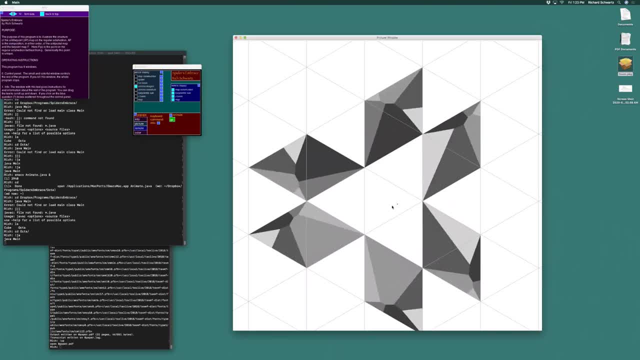 there. now I've turned off all the distracting features, I think I can even animate it, yeah, so. so this shows, like you know, here the point is moving around and this is showing you how the cut locus changes as you go. details. you just can animate anything you want. you know this induces well like: what were we able to日? 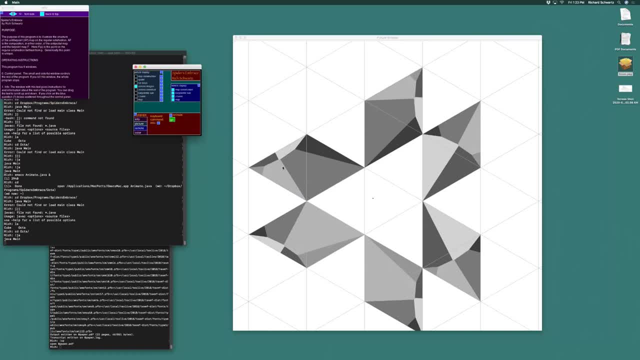 Are you guys happy with what this cut locus is? Does it make sense? It's the set of points where, when you go to that point, these triple points, the blue- are three of the six spider's legs and they all have the same length. So here I'm showing a point in the middle and then 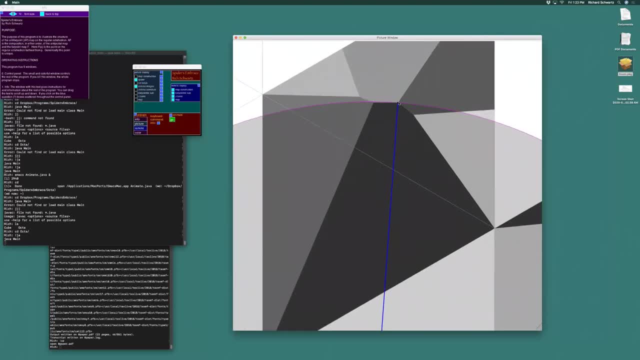 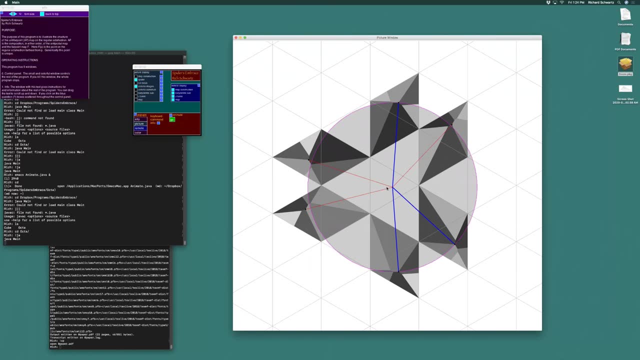 I'm showing a particular point here where there's three, three ways to compute the distance and you always get the same answer. Sorry, just to clarify, there's obviously a triangle in the middle made of four lines and triangles right, And then on each side you have two which represent 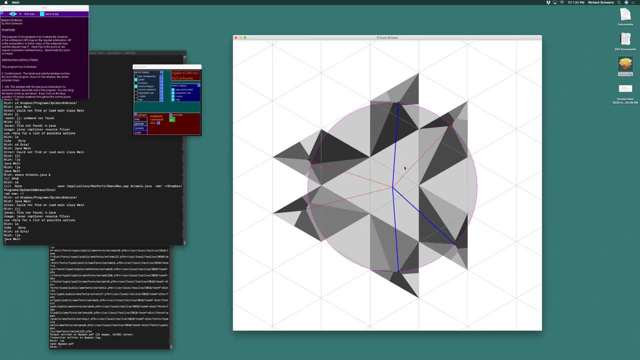 the same one, and then the six outer ones are all the opposites. Right, So that's right. So the inner one, it's just something sort of uniquely representing the bottom of the octahedron, These three neighbors likewise. 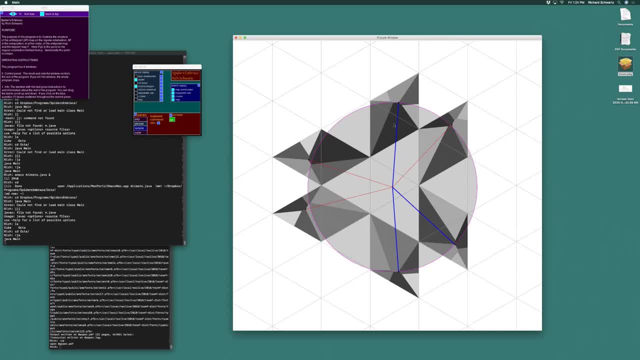 are uniquely representing points on the octahedron. And then these two get kind of folded in together, and so do these two, and so do these two, and then the outer six all just go on top. Yeah, yeah, thank you. 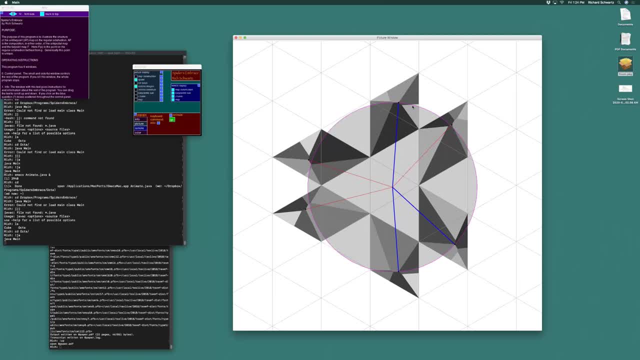 So basically, what I did is I didn't want to have to visualize this thing in space, so I eventually wrote this program which just draws it all out. Let me sort of show you a way of like. you might wonder, like how do I compute this? 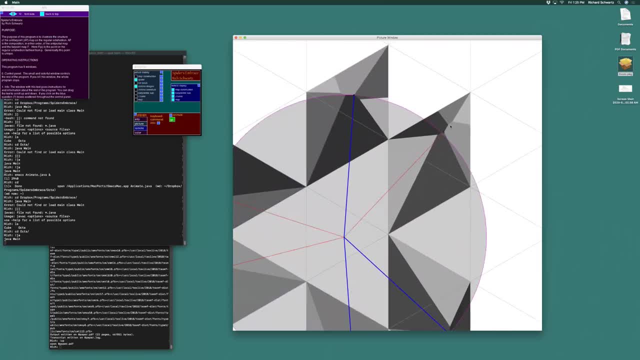 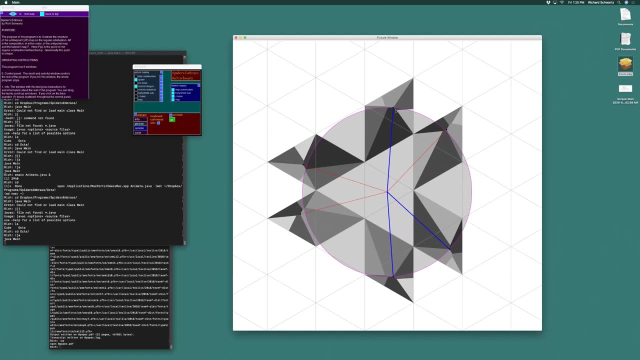 In practice. how do you compute this thing? And what you do is there's well, I'm just gonna tell you the answer, and I'll also tell you that I got it wrong about 50 times in a row before I finally got it right. 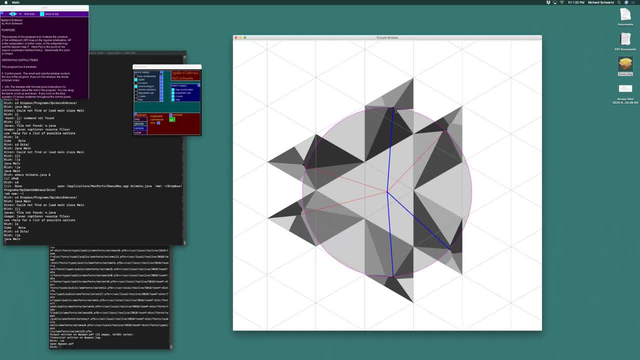 So it shouldn't be completely obvious how it works, but I'm just gonna tell you what finally works. So there's a map that maps this triangle- I picked my favorite one, this one- And then there's maps that maps this to this: 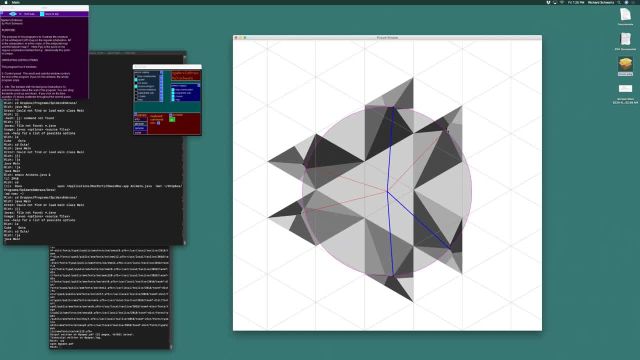 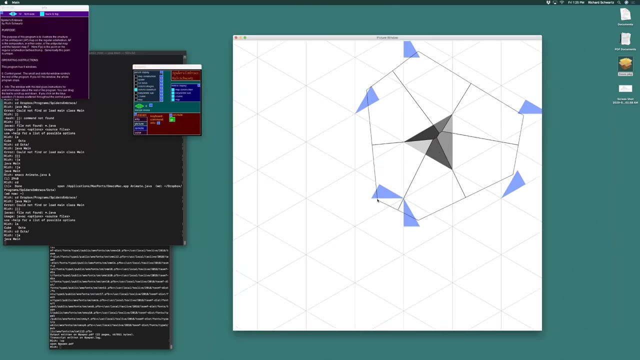 and this to this and this to this. It maps all the outer ones to a single one And I pick the central point and I apply the map to all six of those points. Let me draw this. So what I've got here is my 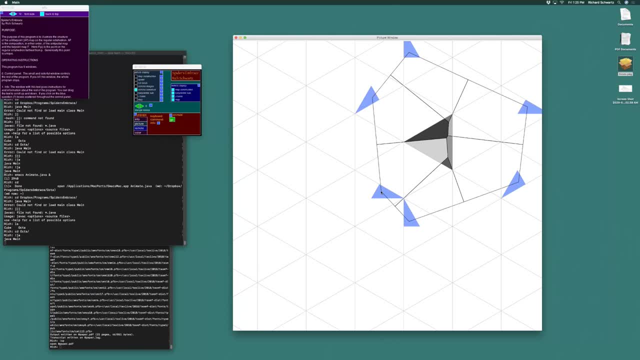 I've got my central point, where my cursor is, and then these other six points are carefully mapped to the point I want to get to. So I've got my carefully chosen points which I get by. I identify, say, this triangle with this triangle. 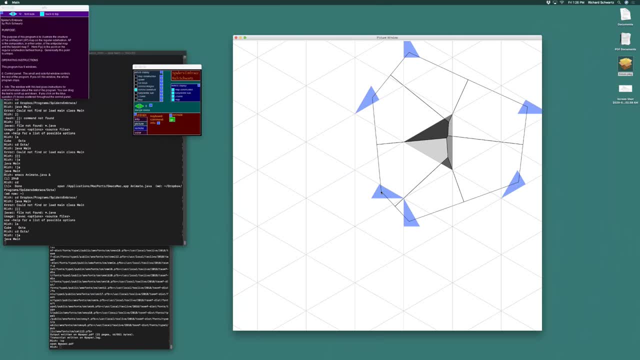 and then I use that map to carry the point somewhere else. So I have the original point and I have five identifications and I just carry this point along with it. This will give me a hexagon. It's just the vertices of this hexagon. 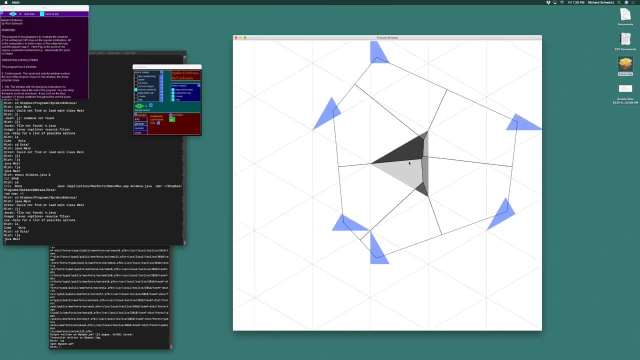 And then what I do is I form what's called the Voronoi decomposition. What I do is I this: this triangle is now broken up and I have to do a new one. I have to do a new one. I have to do a new one. 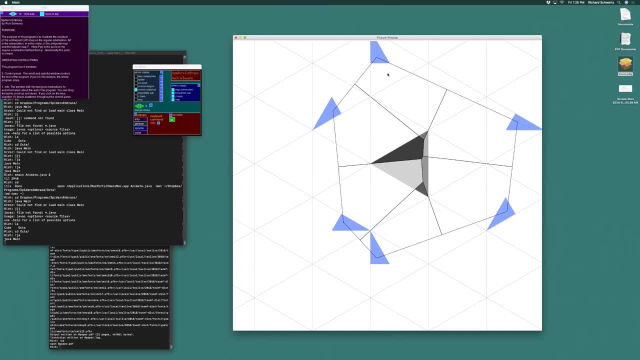 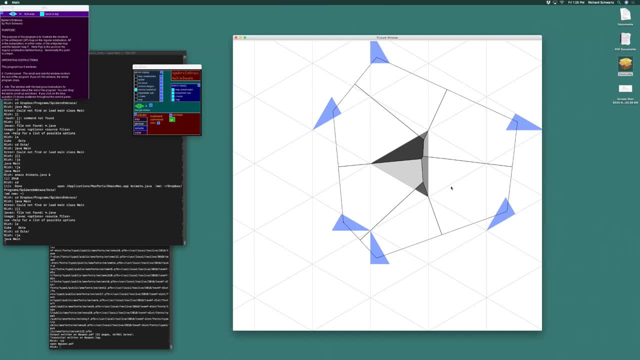 Everything in this zone is closest to this point. So you can imagine that you have a bunch of- you know- people standing around And then you can divide the room up into regions, just all the, all the points closest to person one. all the points closest to person two. 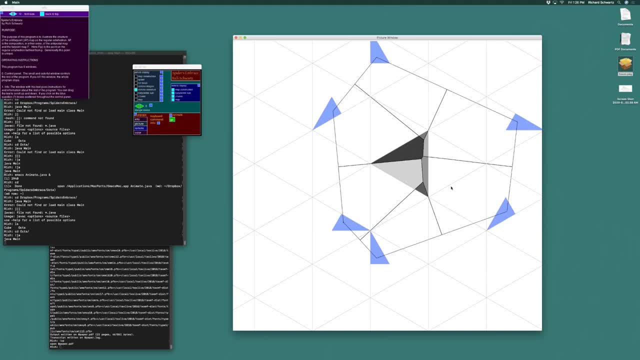 and so on. People call that the Voronoi decomposition, And so this protects you from theache. dead cells, This triangle- here it's coloring in some of the Voronoi decomposition. with respect to these six points, I could shade in the rest of it, but I didn't. 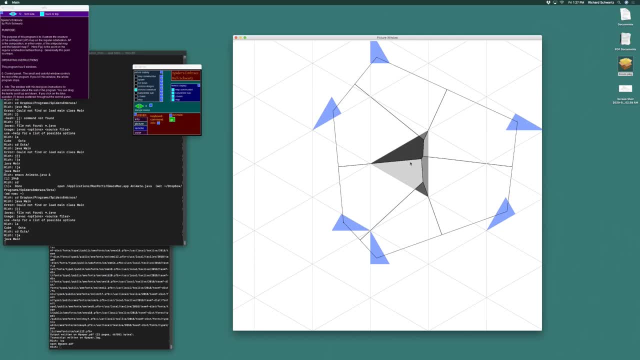 I only shaded in this one, So what I do again. the procedure is: I start with the point in the middle, I move it to the five new location using these kind of natural maps, and then I take this Voronoi decomposition and then I 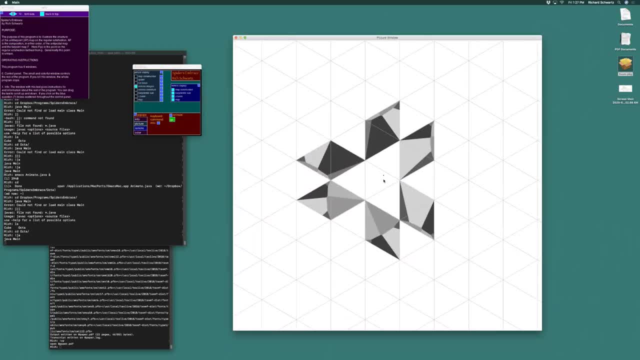 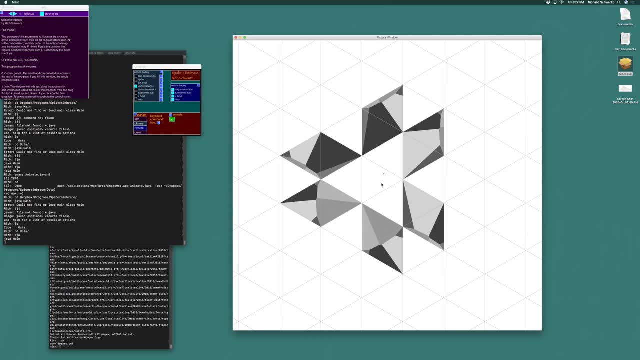 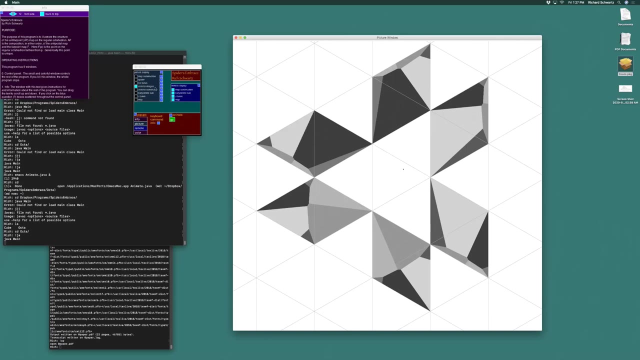 just kind of propagate it everywhere, And that gives me this graph that I was telling you about. Now, the last thing I want to say, which is I want to show you one more picture in this: See, this red region. This red region, like all the points not in the red region, there is a shorter. 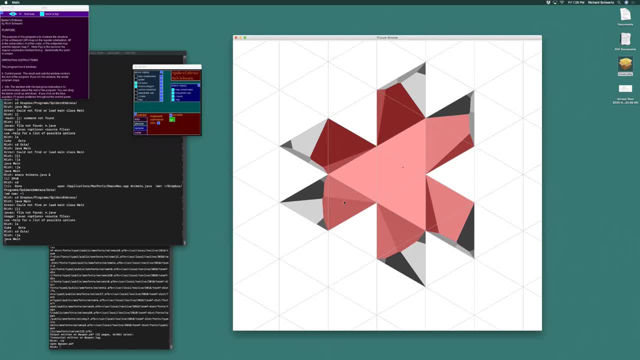 spider's leg that's in the red region that reaches it. So the red region is sort of like it's all the points where there's a unique shortest path and then the boundary is like the points where there's more than one And in fact, 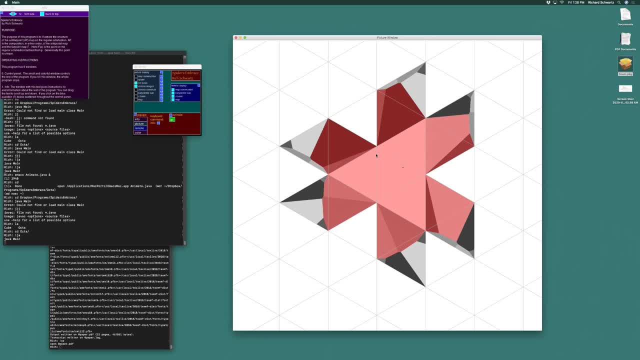 this red region exactly wraps up and fits on the octahedron perfectly. So let me get that in a little bit and then I'll take the other side and set it какrive t it to make sure It's in the circle for these points. 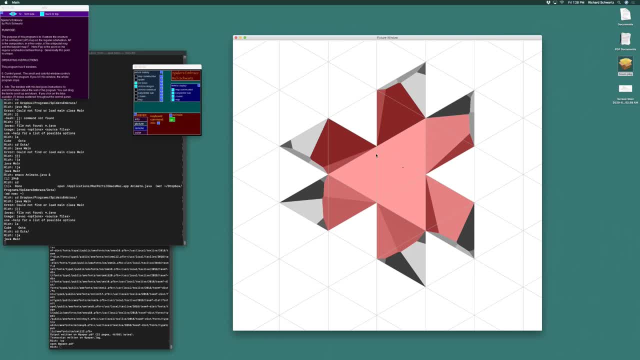 So let me get that in a little bit and see if it works. So let me get that in a little bit and see if it works. give an analogy again, like when you're, when you're wrapping a present, there's often some overlap with your wrapping paper and you may think to yourself like, well, how can i do a better job? 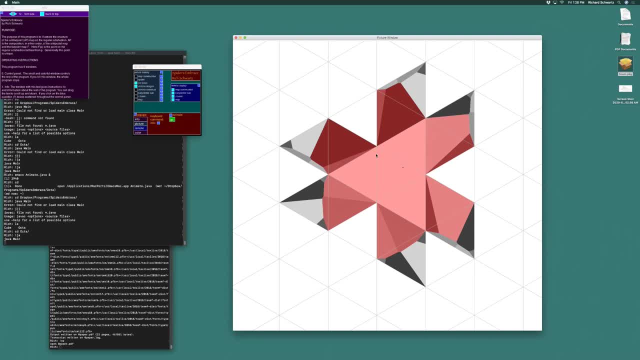 with the wrapping paper, like i don't really need it to sort of fold over so much, i can cut some of it away. and this red stuff is exactly the wrapping paper that you need to perfectly wrap the octahedron and it's. it's sort of like it's. it's sort of like the, the biggest region where every point in here. 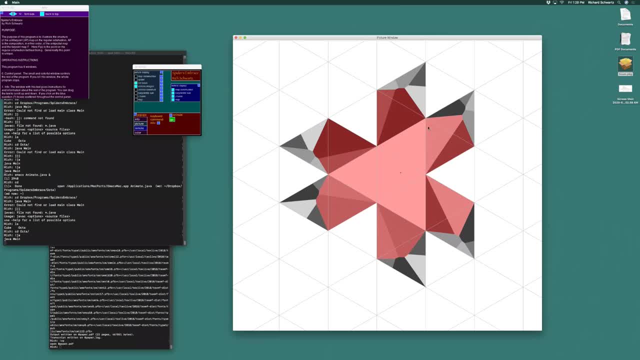 there's a unique shortest path. so, and then this boundary thing is this cut locus. so okay, so all right, so let me, let me stop and ask you guys any questions. so so so far, what I did was just I should you this kind of playing field and I tried to define the cut locus for you and in the cut locus, 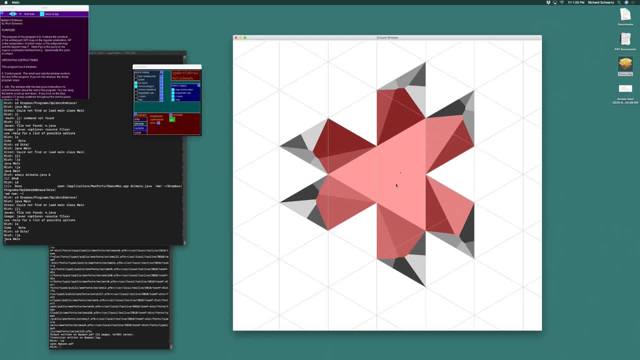 is really. you construct it using this kind of auxilary hexagon and then you, you kind of make this red polygon and that's the UM, that that's like the region, that's like the inside of where the cut locus is. so okay, so, so, so far. 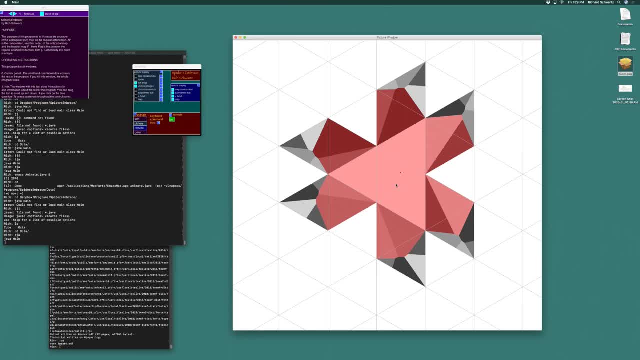 I haven't been talking yet about. I just just been talking about the geometry of the octahedron, and now I want to relate this to the farthest point now. so so I think I pick a point here, and here's the beautiful fact. the beautiful fact is that the farthest point is always a vertex of a cut. 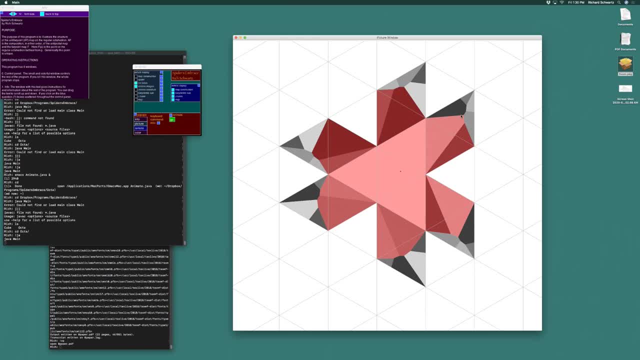 look of the cut locus. so so let me let me try to give you some intuition for why that's true, without really giving a formal proof. let me stop the screen share for a minute and then I'll come back to it. yeah, now I'm going to draw a kind of a caricature of what I, what I. 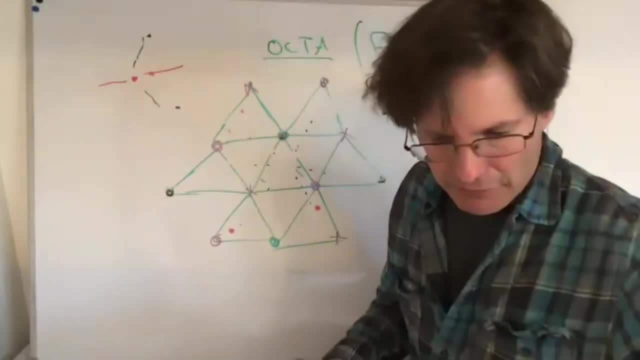 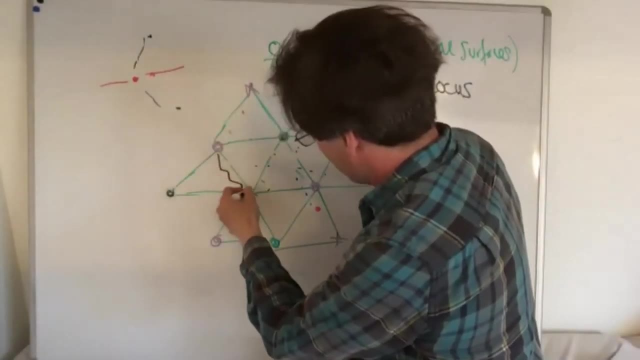 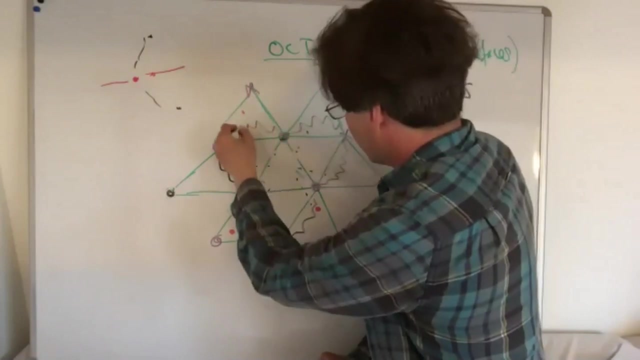 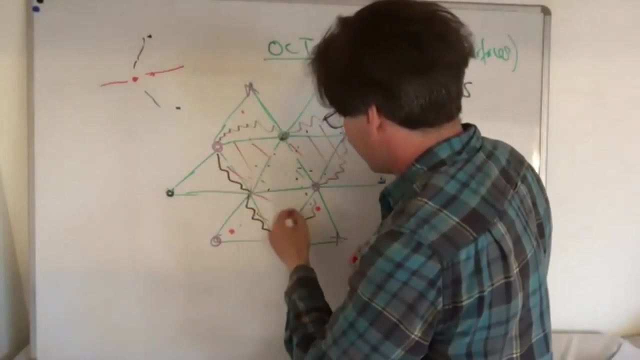 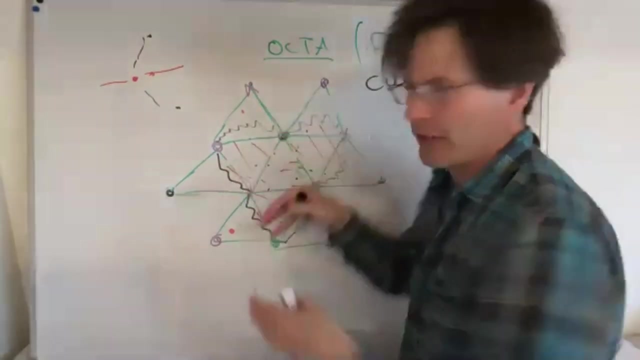 had in a computer program, so I still have the playing field. and then I've got this thing which kind of goes: oh man, how does it go? you know something, something like. and then there's this kind of red part in here. so this is the region of points where there's a unique shortest straight line and then the boundary. 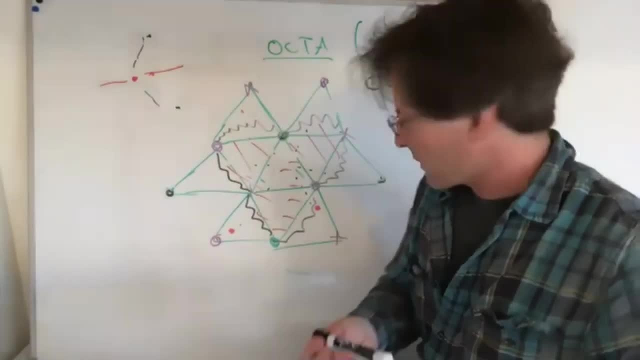 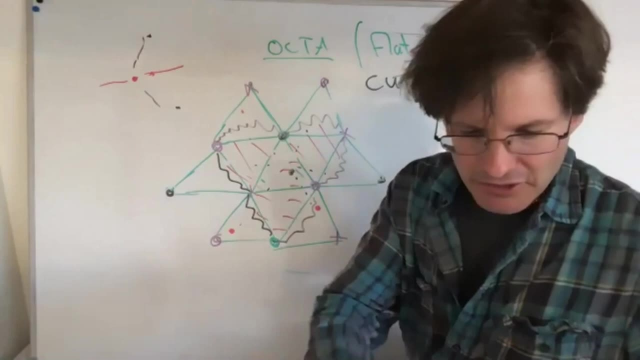 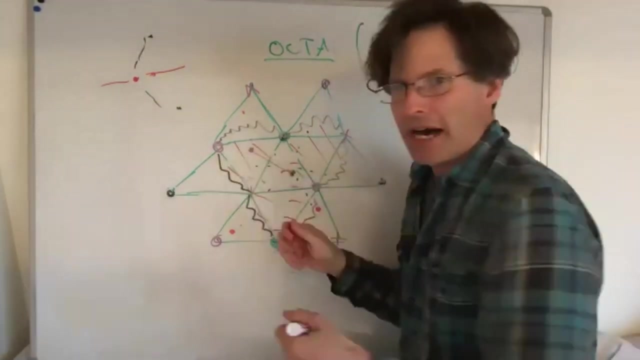 is where there's ties. um, so, so I met, and it's all with respect to some point. if I move the point, as you saw, the shape moves around. um, so why? why couldn't this be the farthest point? well, you know, there's this unique shortest path, and then, well, I could just push it a little bit further. 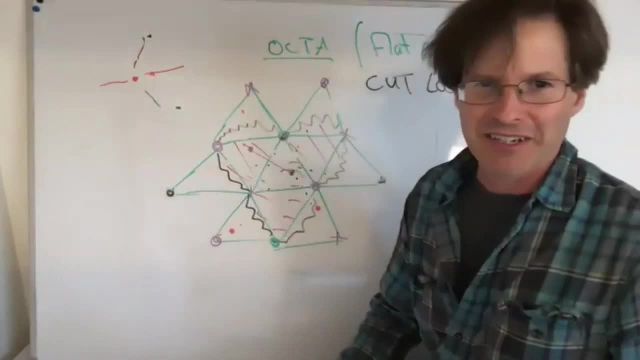 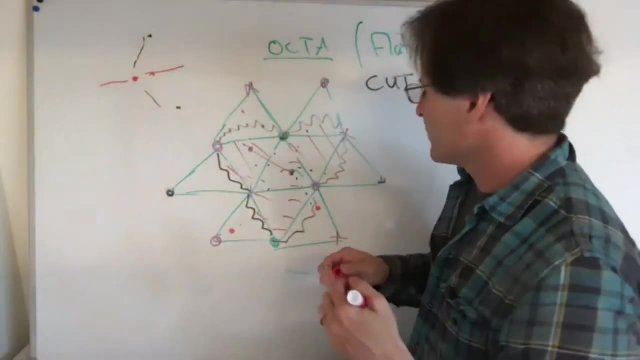 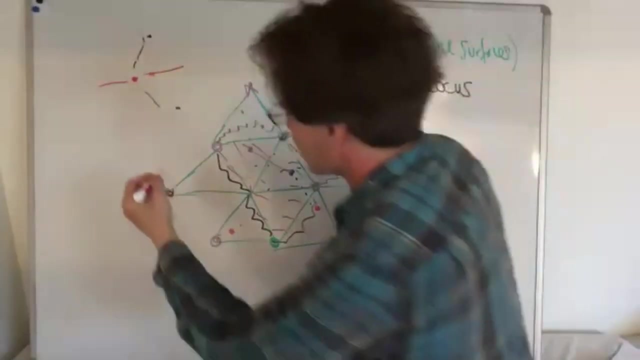 and then that I'll get a farther point. there's no other way to do it, so I'm just going to draw a line. there's no other competitors, so the farthest points really really have to be on the edge here. but what? what if they're not at a vertex? well then, the picture is something like this: you, you sort of. 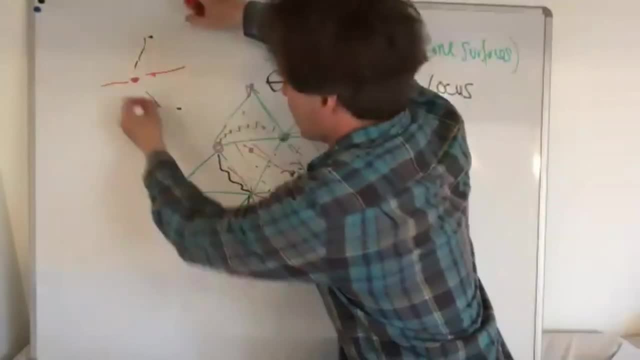 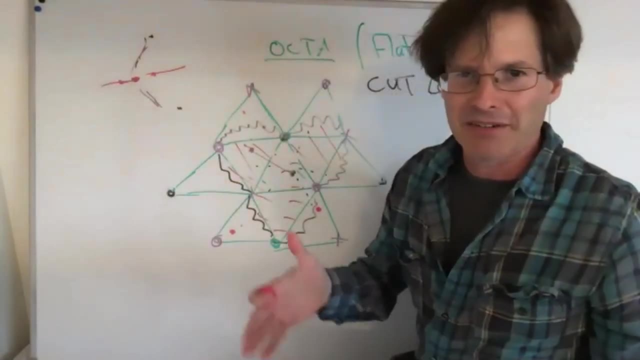 have this point here, and then here are these two things that are closest to it, but then you want to get further away. you can just slide along this line one way or the other and that'll make it. that'll make the point: go further away, and there's no other competitors. 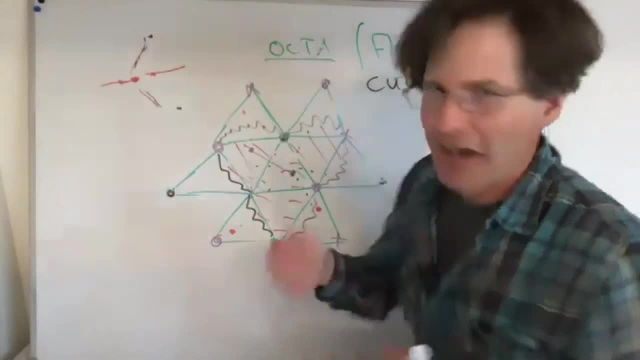 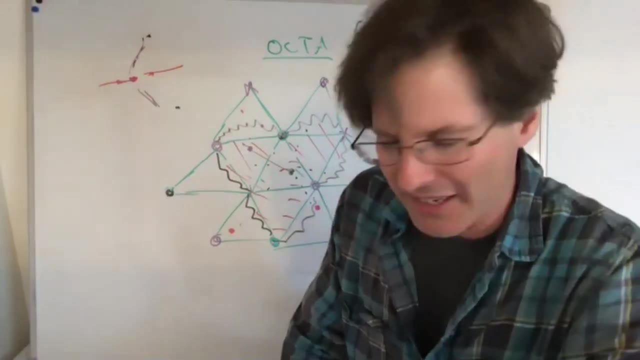 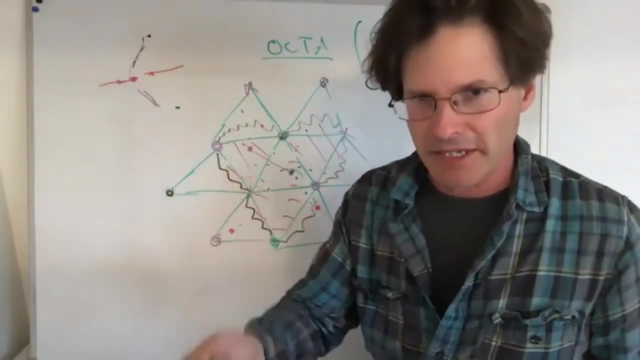 there's no third one that's closest, so so if you're not a vertex of the cut locus, you can get further away. um- and people know this- about some general kind of surface like any convex surface in space, that the farthest point would have to be a place where at least three things come together, and that that's. 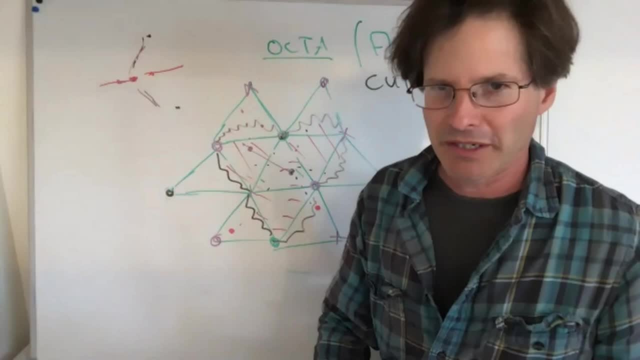 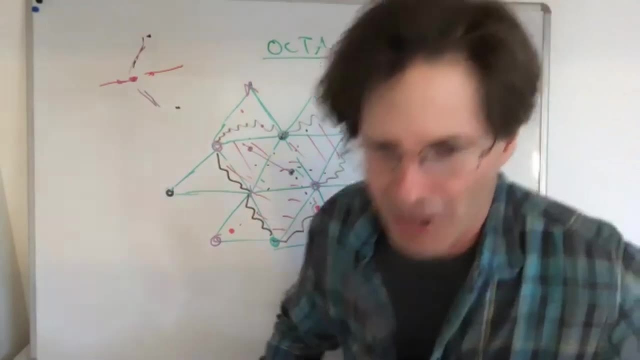 more or less the argument I just gave you. if not, you just can sort of slide it along and one way or the other and make it farther away. so okay, so now I'm going to, now I'm going to share the screen again. so I'd like to say that I 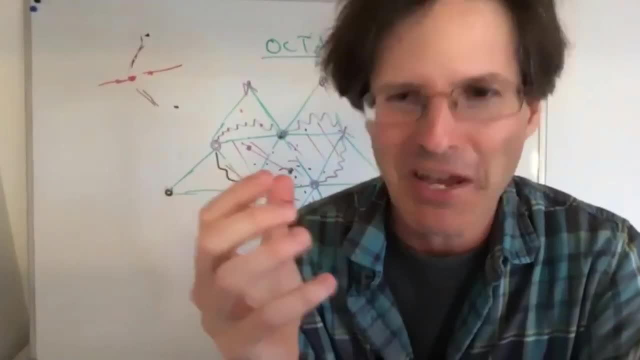 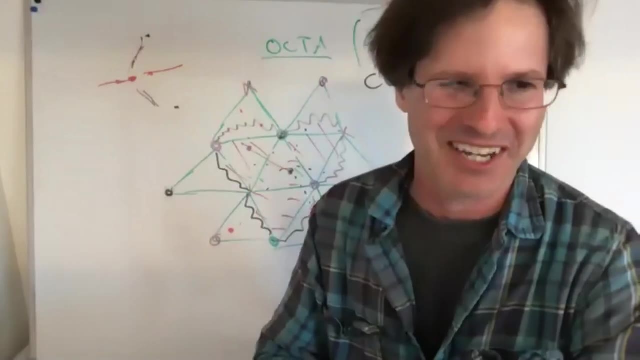 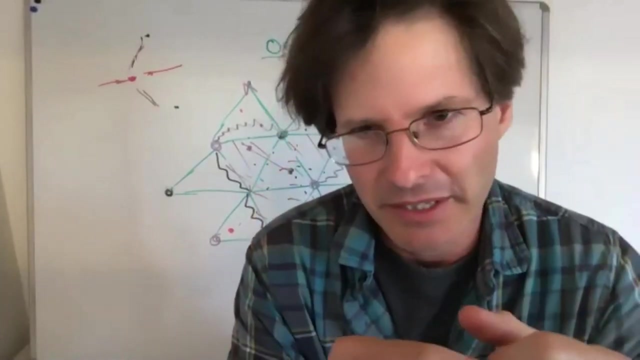 actually discovered this by thinking about it, but in fact I just kept doing numerical experiments and just drawing all possible pictures until I just sort of noticed that it was a vertex of the cut locus. then I sort of realized: there is this proof. if you're interested in figuring out what this map is, this, this: 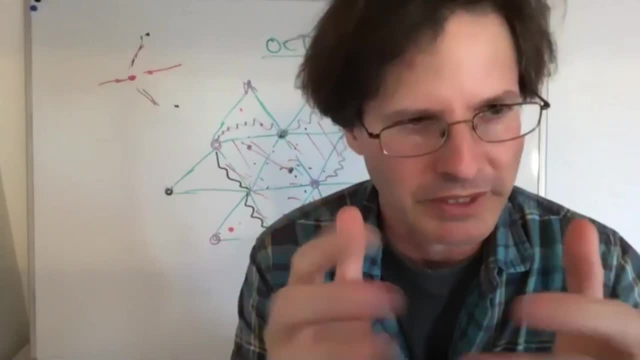 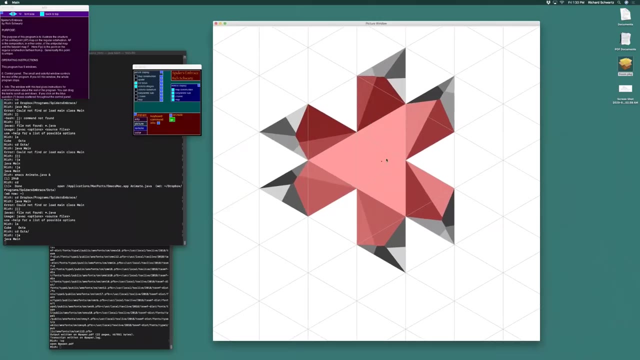 simplifies the problem a lot because it tells you what the cut locus is and what the vertex of the cut locus is, and it tells you where to look for what the farthest point is. um, let me, let me do the screen share again. so now I'm again like I'm moving around the central point, the. 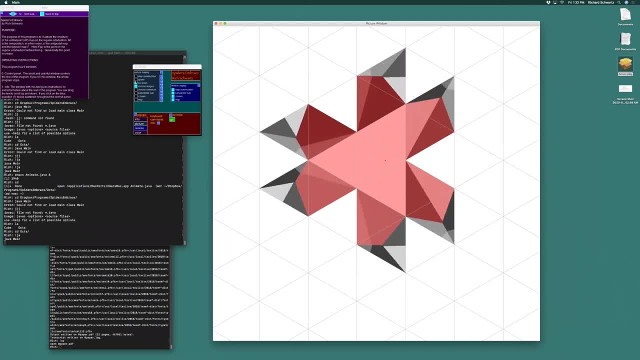 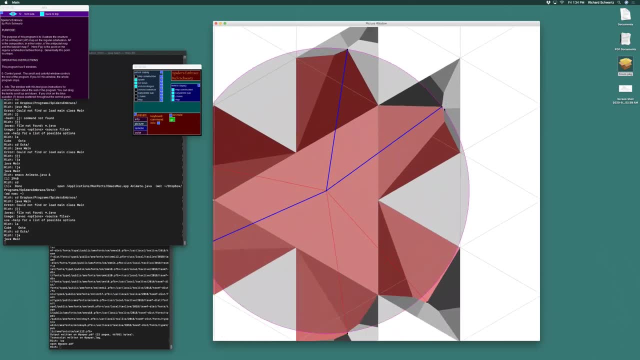 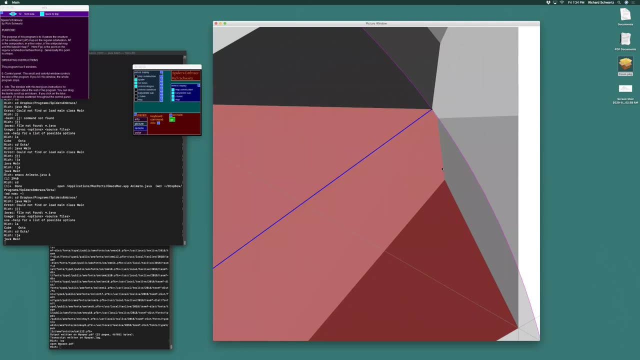 cut locus is kind of changing, so. so now I'm going to turn on what I call the spider. it sets up a kind of competition you've got. if you look at this thing, there's really four, four vertices, and and one of them is going to be the 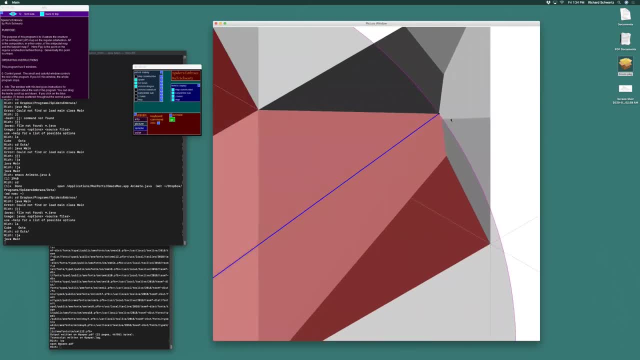 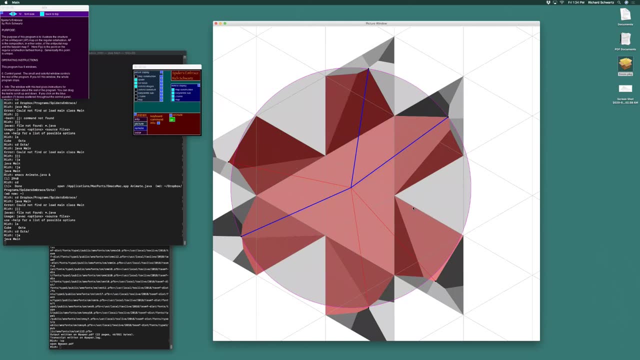 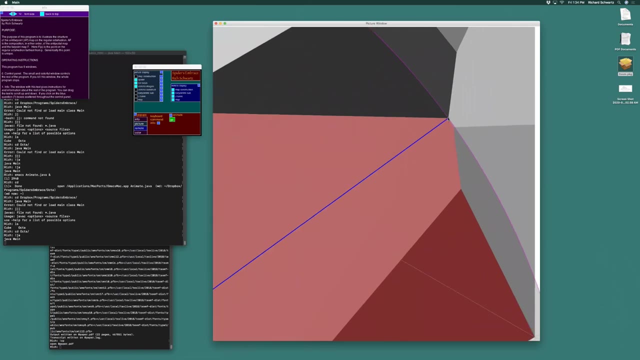 farthest point away, but to measure the distance you have to really look at all four of them, in all of the triangles, and then figure out which which one's the farthest. so, um, so it turns out that in this case, this one's the winner. um, if you look closely. 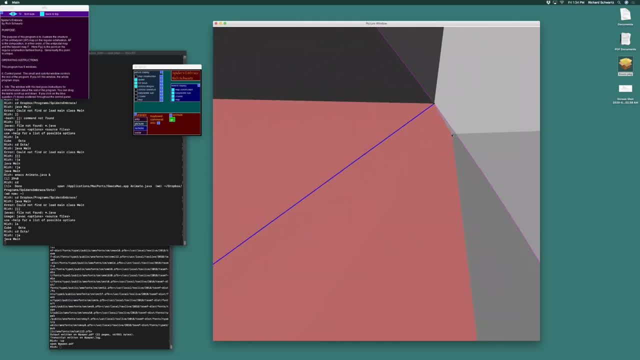 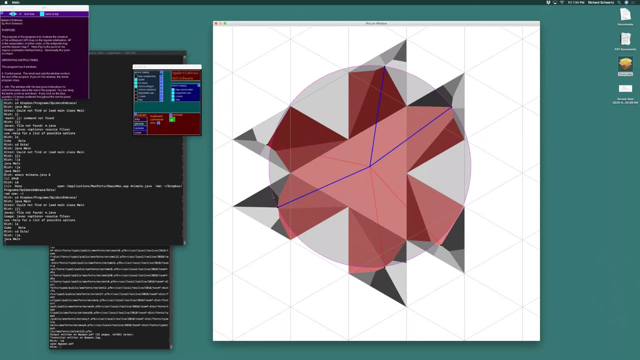 this one is closer and so it loses. and you might say: well, why isn't this this kind of dark one over here? the winner it's because, if you look at it from the other side of the triangle, it's a loser. so the ones that win are not losers in. 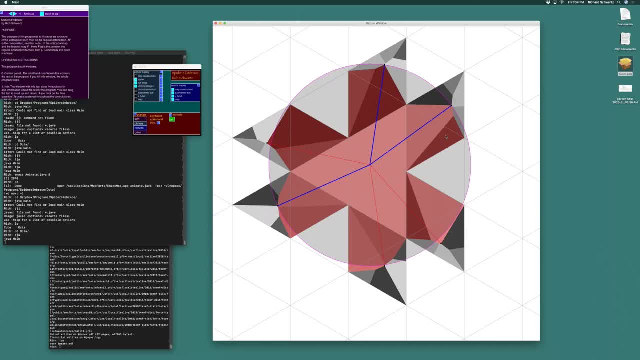 any of the other triangles- that's the way to say it- like in some of the triangles that one of them might look like it's further away, but it's if it's closer than another one, it loses. so you have to sort of run this six-way. 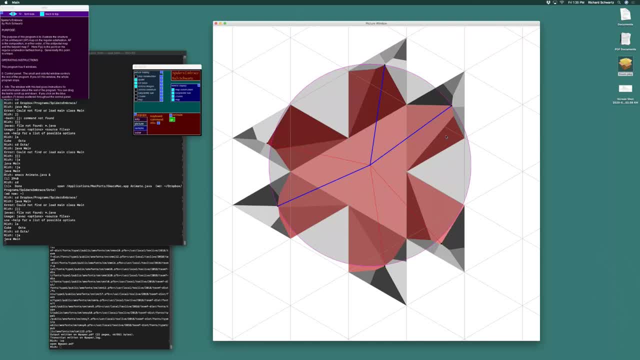 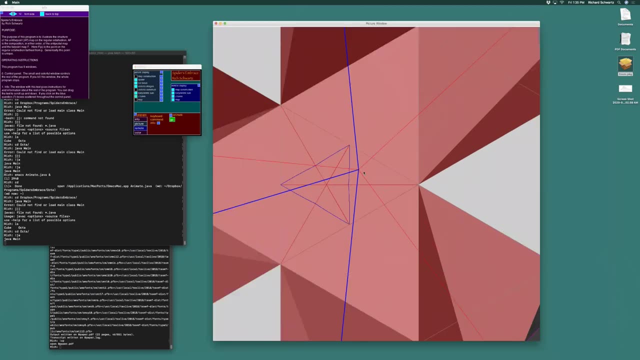 competition, and whichever one is not the loser is is the winner. so so anyway, the blue ones are sort of showing which one wins. so then of course I got organized. I'll turn on a little more stuff, okay. so firstly, the the regular octahedron has some symmetry. there's a group acting on the regular octahedron. 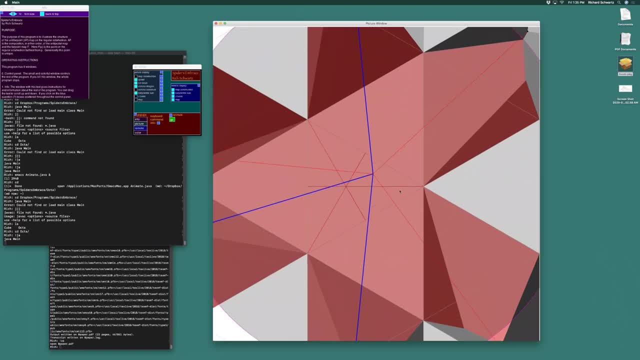 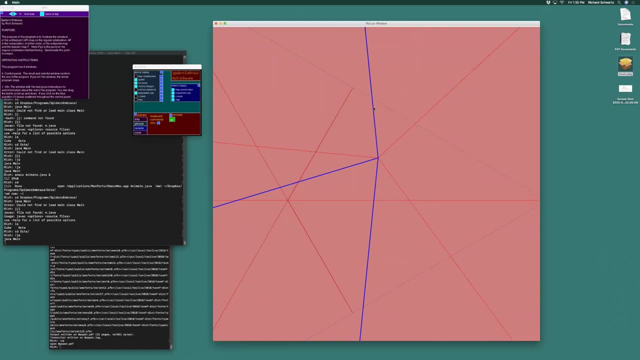 it's the group of all you know symmetries of the thing and this triangle here that I'm drawing right here, this is, this is what they would call a fundamental domain for the symmetry. it's a it sort of has the property that if you, if you move it around by the entire group, you tile the 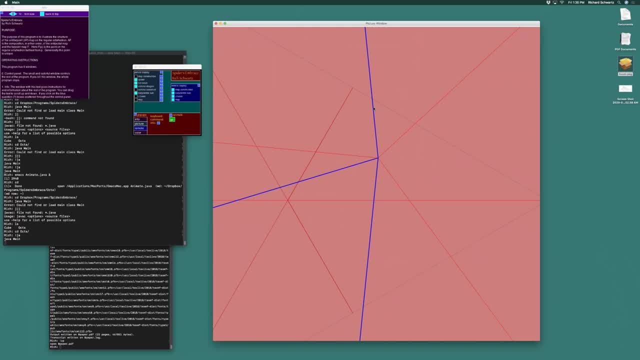 octahedron. so rather than understand what this farthest point map does all over the octahedron, you might as well just understand what it does in this fundamental triangle, because for the other ones it just follows from symmetry. so after a long time I'm gonna. 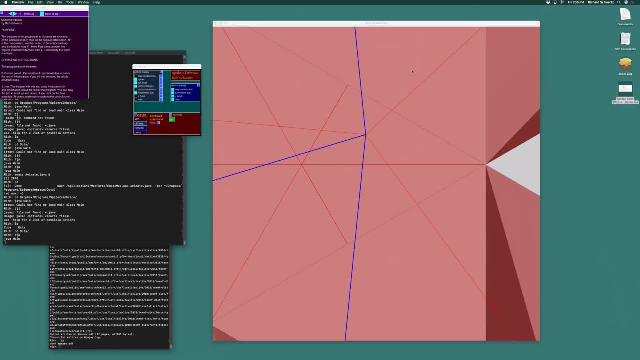 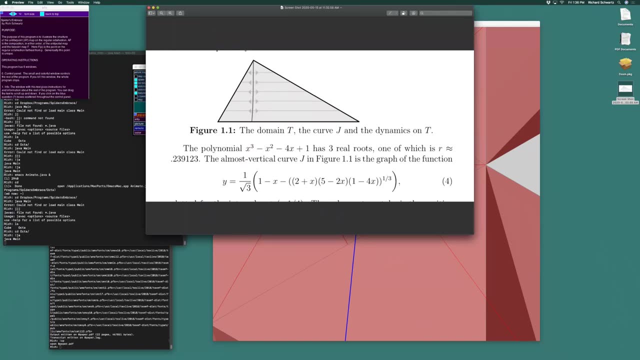 bring up a kind of disgusting equation. you, you look at this polynomial x cubed minus x squared minus 4x plus 1, and one of its roots it's 0.239, and then you plot this function from 0.239 to 0.25 and you see this thing which sort of looks like a. 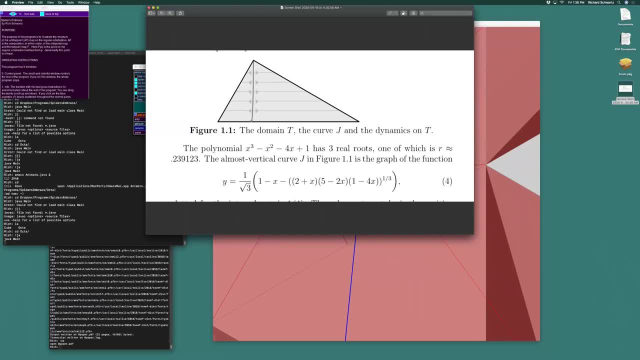 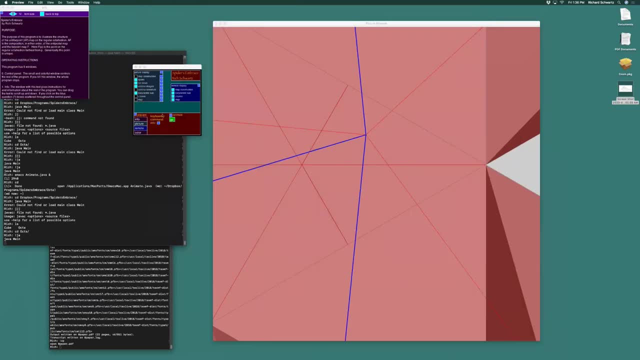 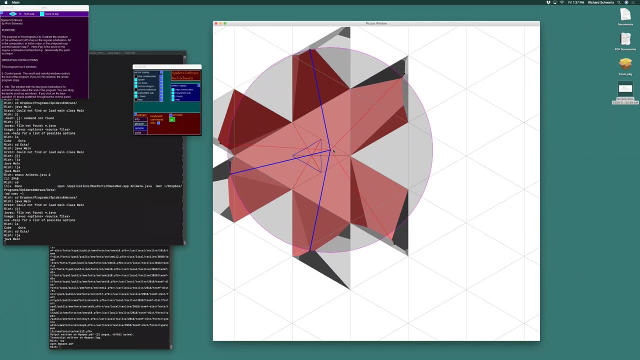 like a J I mean, and that J is the graph of this function. so so, here's the neat thing. um, here's the J curve, this blue thing, and if I stay away from the J curve, the answer doesn't change. and then, when I cross the J curve, the answer. 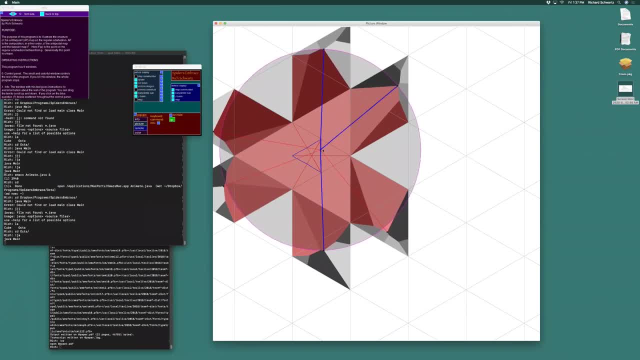 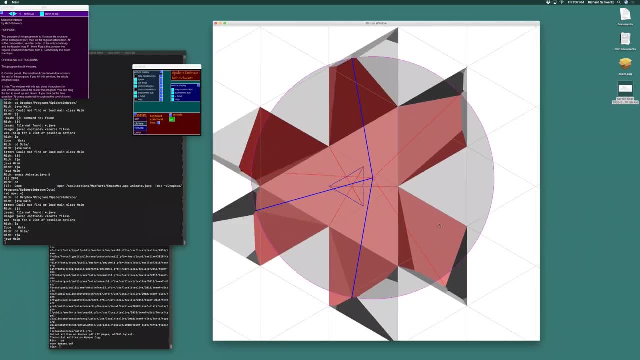 changes. but you know you might wonder: how did I find the J curve? I just looked at the picture long enough and figured out: when does this thing change? and like like the J curve, if you look really closely at it, it's. it's the place where these two 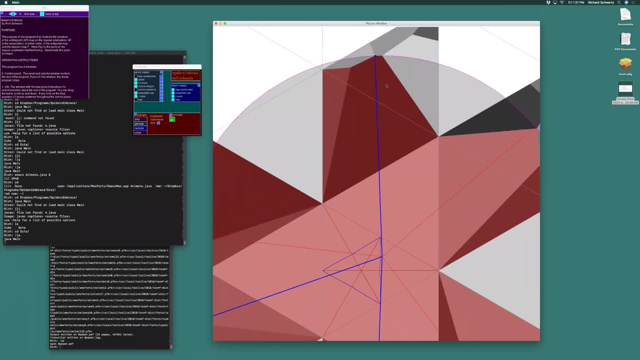 points are kind of like equidistant, and so I eventually just computed what this thing was and got the, got the equation for it. so there's two levels of things that are going on. if I, if I turn off the spider, then inside this regular curve is 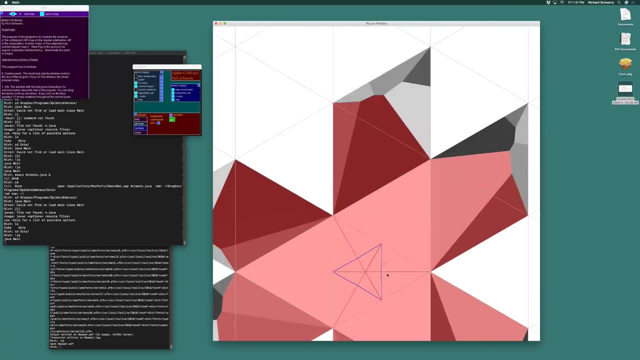 this region. the picture of this graph does not change. The lengths change, but the combinatorics don't change. If I go to the boundary, it changes in various ways. Things come together, but at least in the middle it doesn't change at. 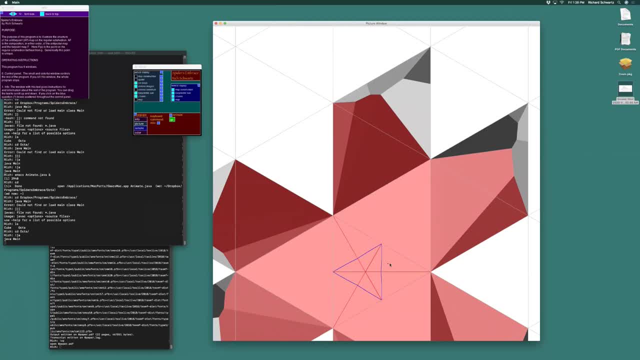 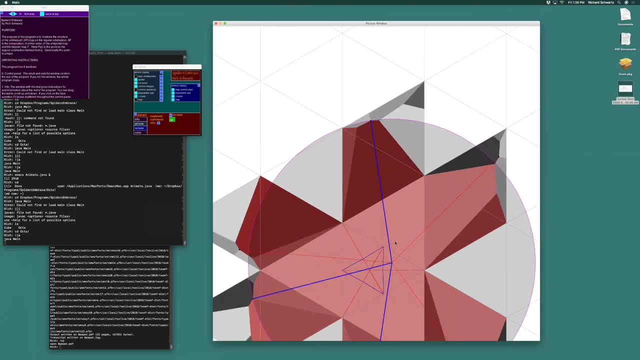 all. Then the second level is when I cross over the J curve, somehow the answer switches without the combinatorics of the thing changing. What I'm telling you is that this points the winner on one side of the J curve, and then this points the winner on the other. Before I prove that, 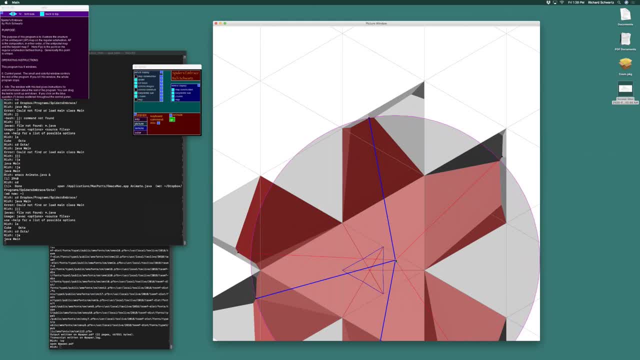 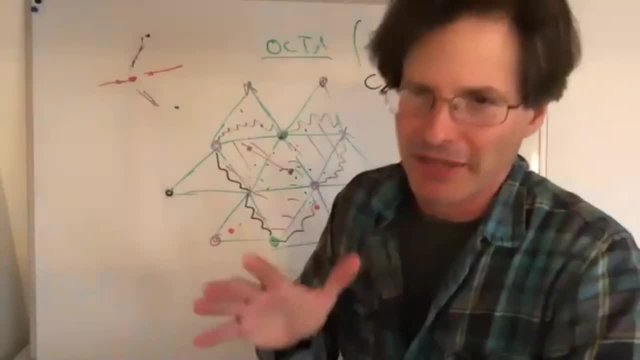 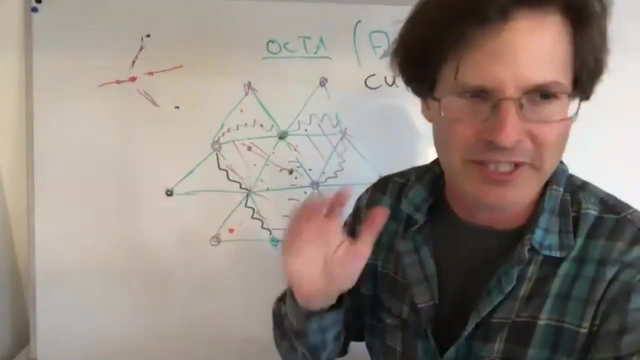 I'll tell you its consequences and then I'll go back and I'll explain the proof, at least in outline. Here's what I'm claiming without a proof, and then I'll get back to it. There's certain of the vertices. are the winners? and I can tell you. 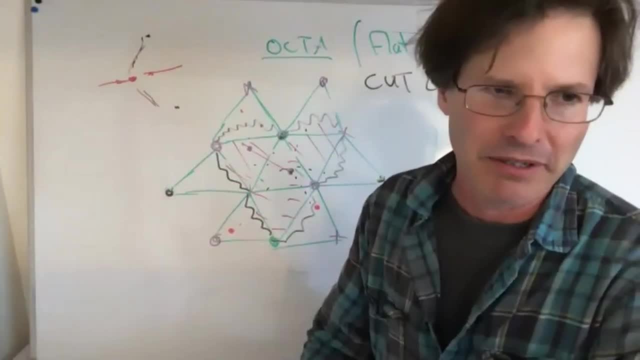 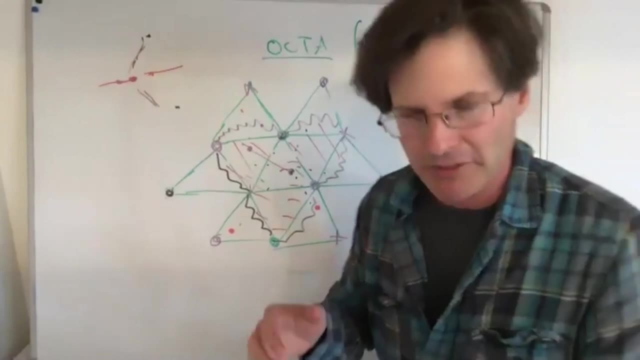 what they are, and that's the answer. That's the farthest point map. but it's neat, You can interpret this in a dynamical systems point of view. What a dynamical systems point of view is you say? well, I start with the point. 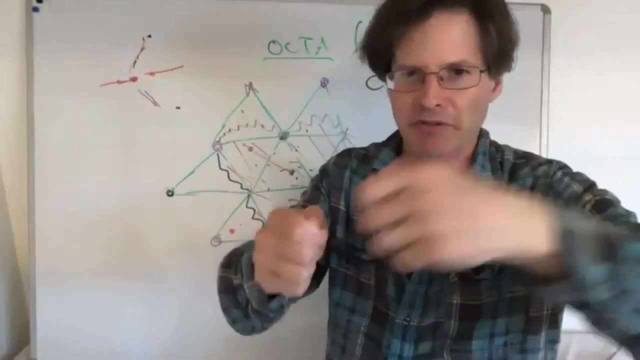 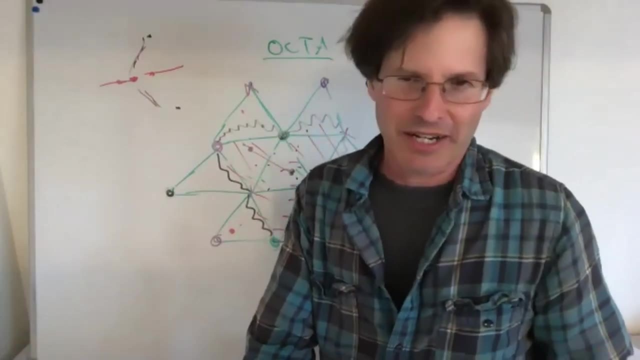 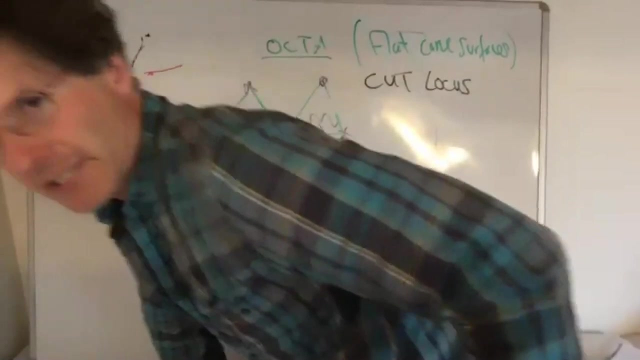 and then I pick the farthest point, and then I pick the farthest point from that and so on. I sort of watch this point kind of bouncing all over the octahedron and I kind of look at what happens. Something really neat happens. I'm going to look at something. 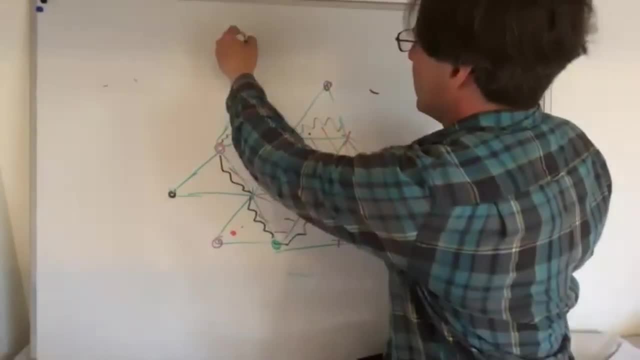 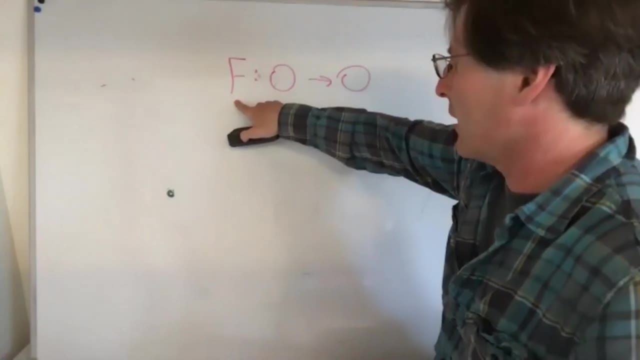 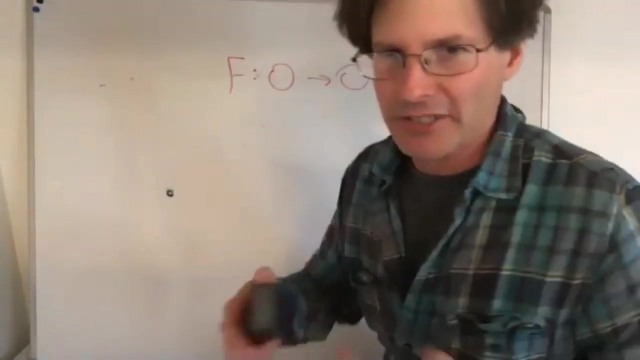 slightly different. instead, Here's the octahedron. I'll call it O. F stands for farthest point map, and so I could just look at F, squared, etc. and you could say: I start with the point, like what happens. 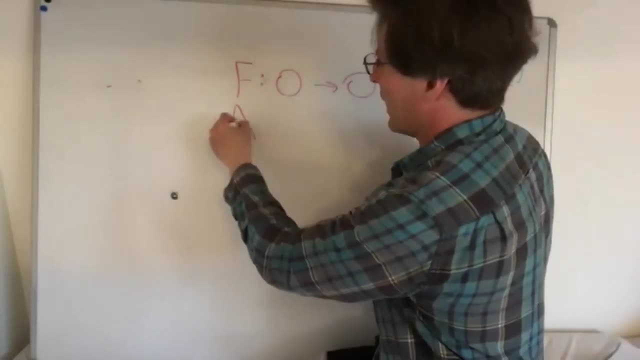 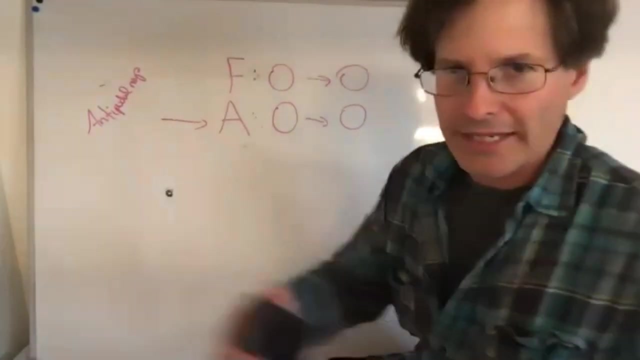 but I want to look at a slightly modified thing which is nicer. I want to look at there's another map. This is the antipodal map. The antipodal map: every point on the octahedron has an opposite point, and so what I do is I 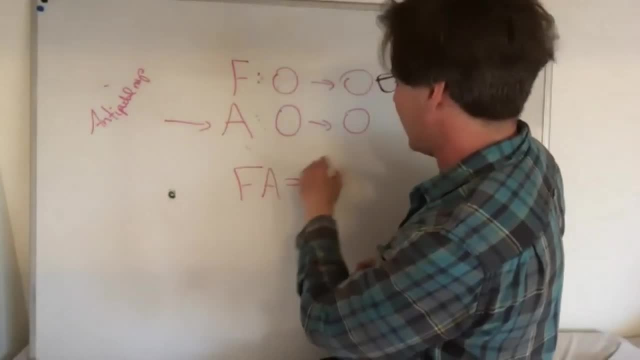 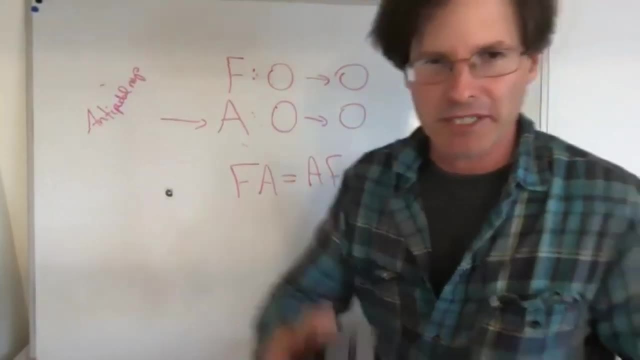 look at the, it turns out that FA equals AF, just by symmetry. so they commute. Instead of looking at F, I look at FA because it's nicer, because you pick a point that's on one side and it goes to the other. 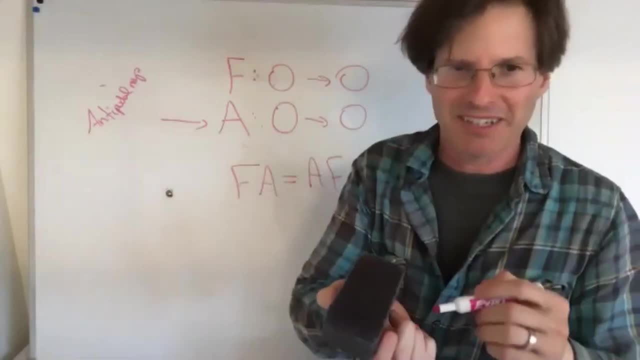 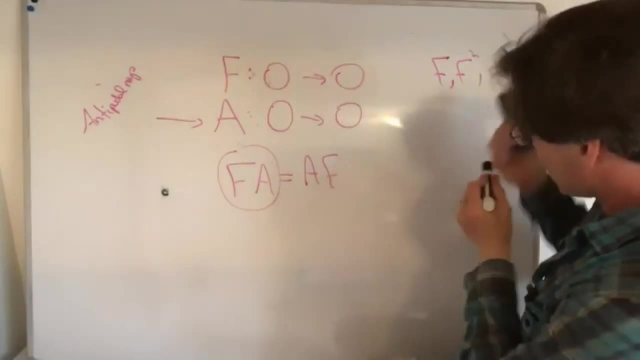 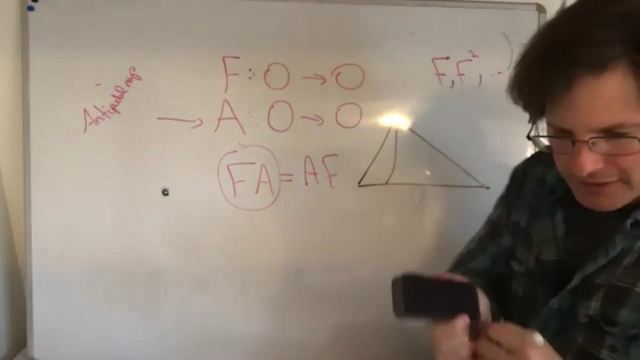 side, and then you map it back and it comes pretty close. This thing's nice and what happens is in this fundamental triangle. so I'll try to draw it like this. Here's the J curve. It turns out that there's a 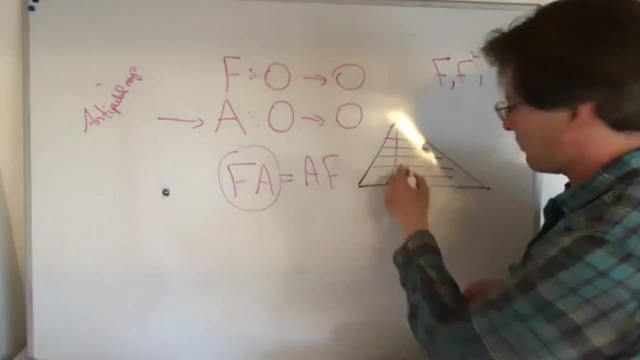 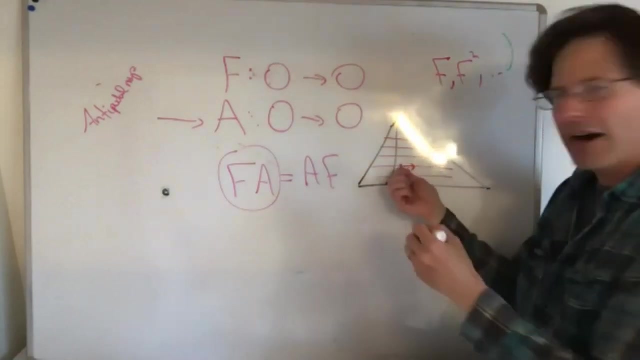 family of horizontal lines and if I pick a point on this side of the J curve it stays on the same horizontal line and it just goes out a little bit and everything kind of moves outward, and on the other side it kind of 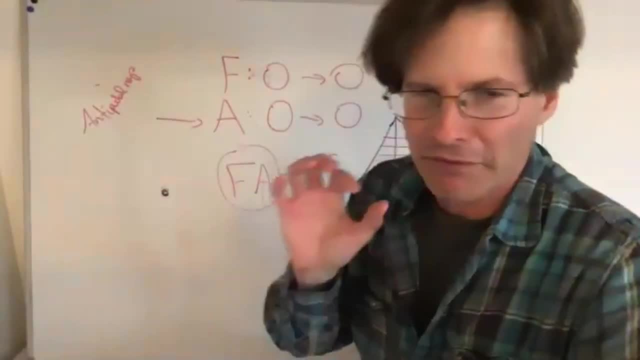 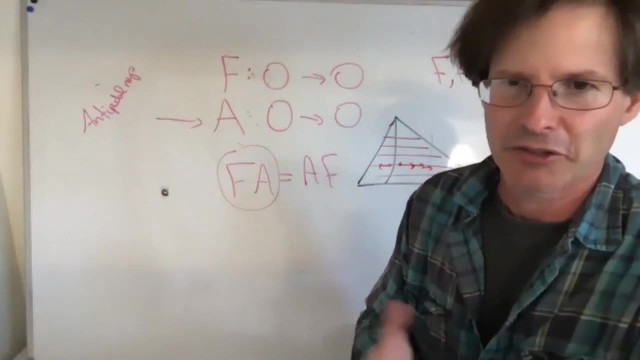 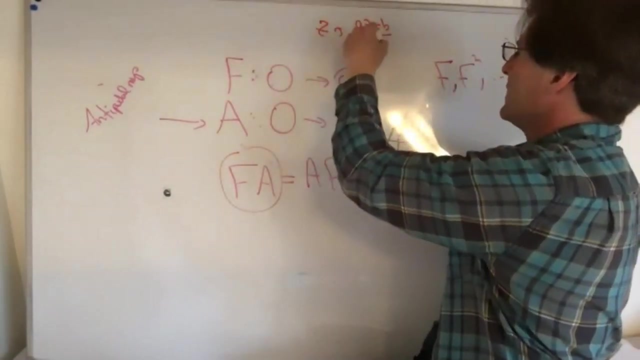 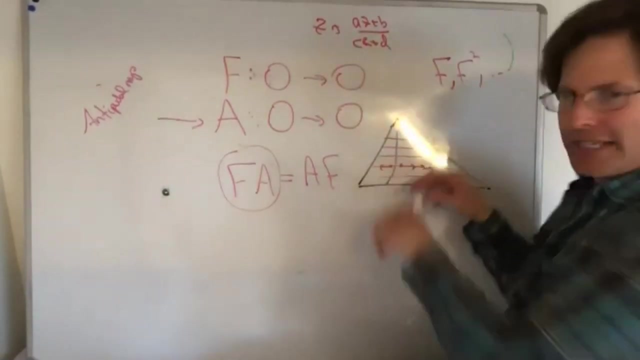 moves this way. If some of you have taken a class in complex analysis or in hyperbolic geometry, you may have heard about things called linear fractional transformations. They're maps of the form like: Z goes to AZ plus B over CZ plus D, and when you restrict FA to each of these line segments it's a. 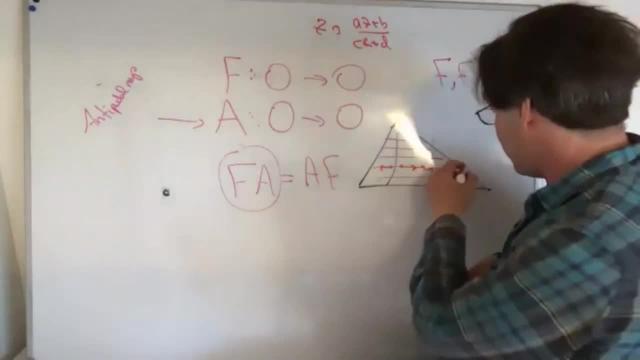 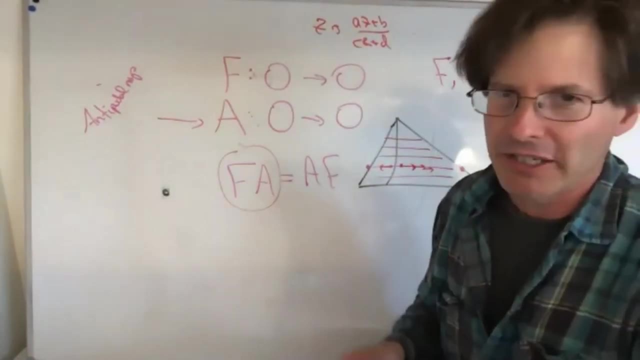 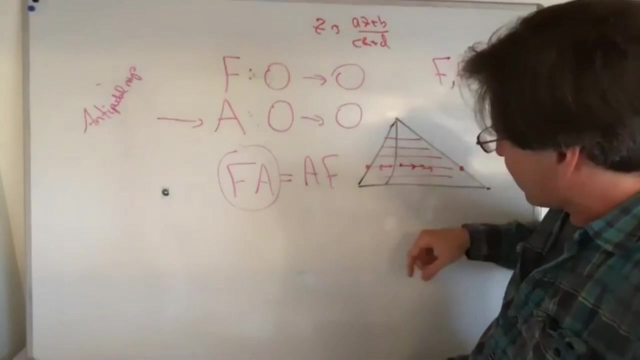 map like this and it has a fixed point of intersection over here and also over here, and the entire map is what people call birational. It's given by the quotient of two polynomials, so it's a. it's a birational map. It preserves the horizontal lines and, when restricted to, 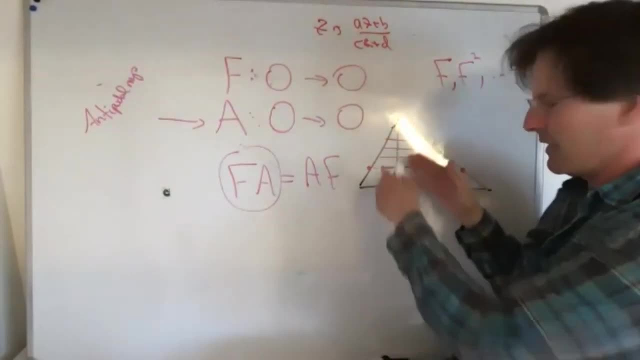 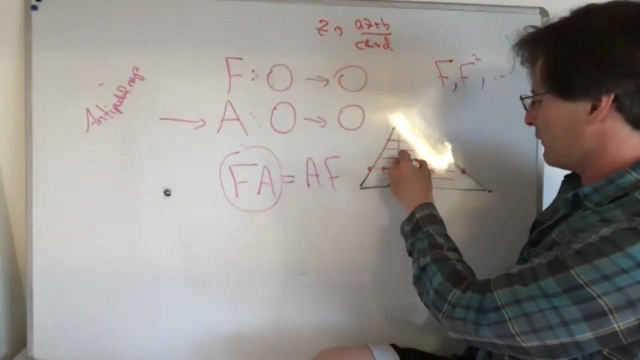 each of these segments. it's a linear, fractional transformation, and so what this means is that if I start with any point in the octahedron and I start applying the four-point map, it goes boom, boom, boom, boom, boom and it. 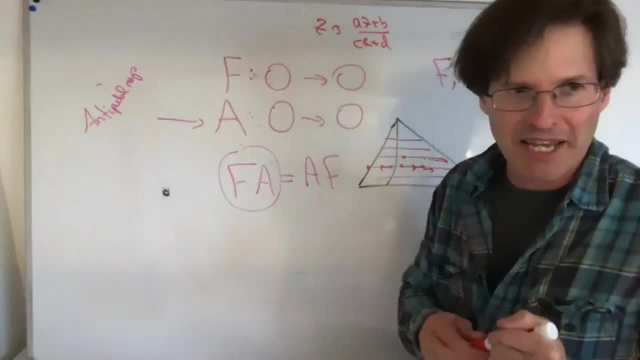 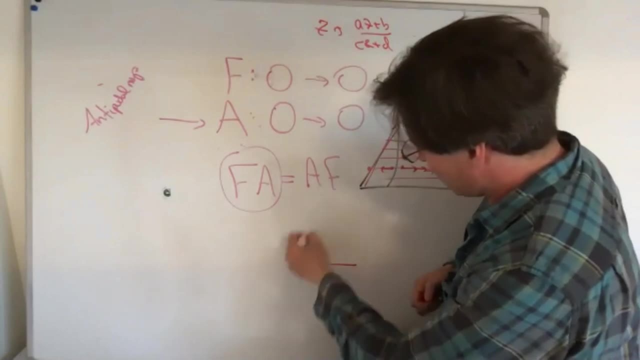 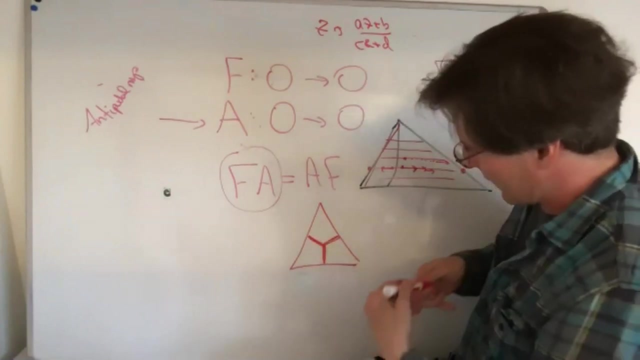 just pushes it to the other side. It pushes it to the edges. so the long-term behavior is that everything just goes into the edges, or I mean, or this edge In the full octahedron, you have these kind of kite-shaped things and the picture is: 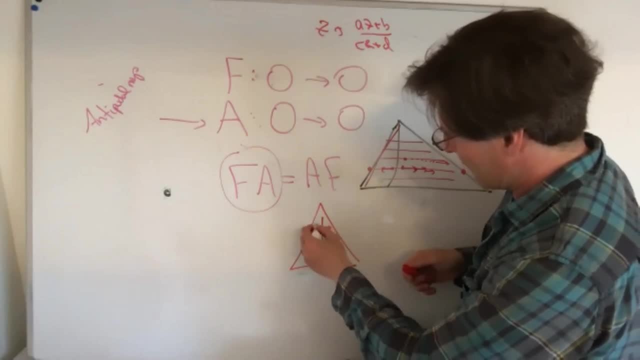 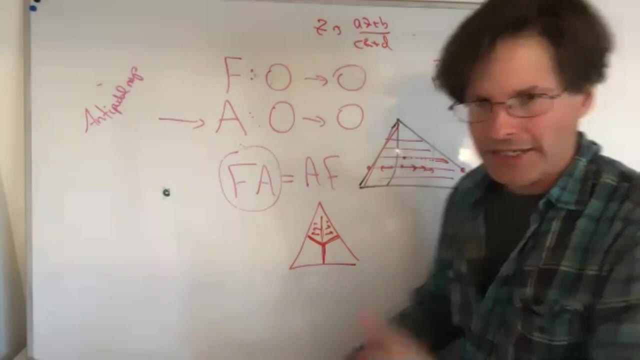 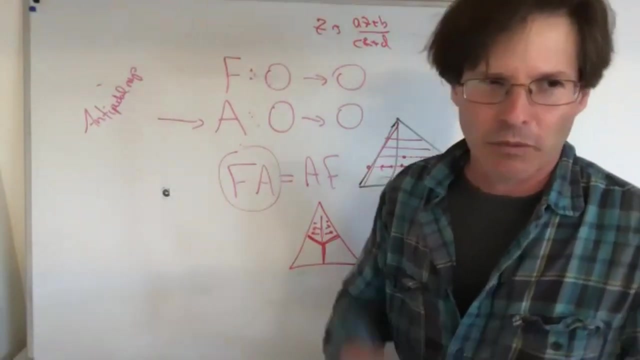 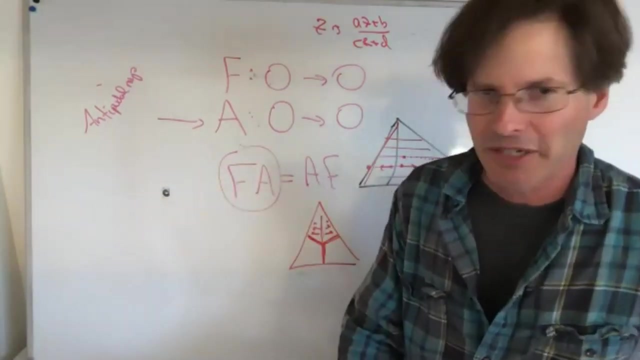 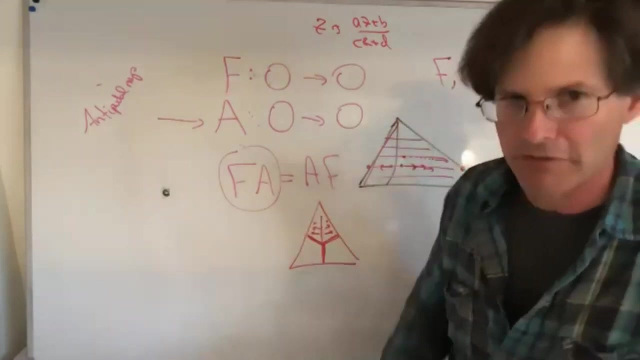 that everything kind of pushes out to the kite-shaped thing. So that's sort of the final answer. It says if you've had a dynamical system you'll find you're at a cross. Then you can are the octahedron. For this class. I'm really interested in what it is. People are interested in this thing they call the Omega Limit Set. What it is is you just pick points and you see where they go and where they accumulate. That's what the Omega Limit Set is. 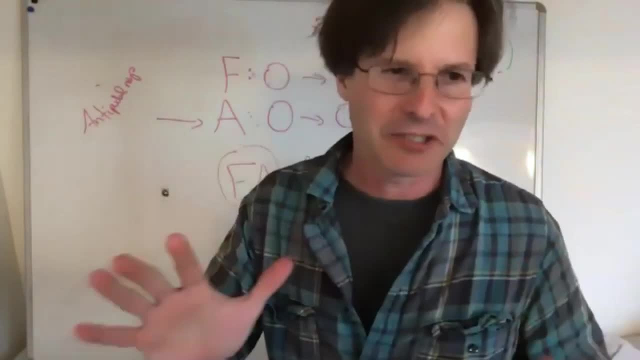 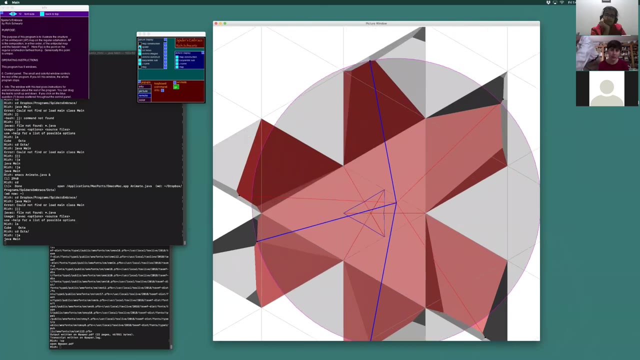 thing, and then I'm going to- and then the rest of the talk is algebra. I'm going to sort of show you what this map is geometrically. I worked it out, uh, and I'll tell you again. I once had a kind of very elegant geometric proof in mind, but then in the end I- just when I wrote the paper I just got- 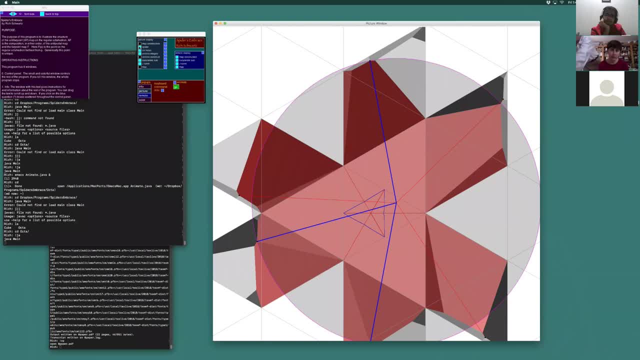 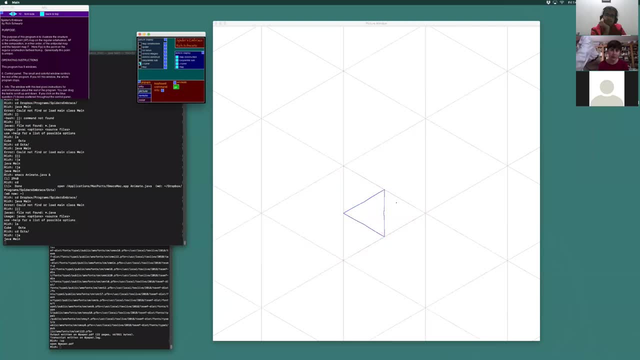 lazy, I just just wrote the equations down, you know, and said: here it is. it works but, but I did take the time to actually so. so in this picture that the, the place where my cursor is is the point X, and then the other point is f a of X. so what you do is you can be generated by a straight line. 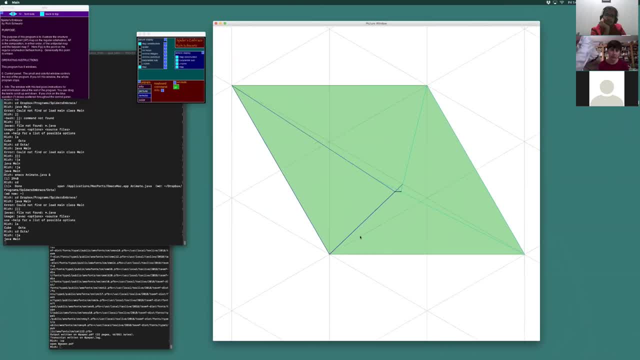 construction. you, you take this, you take this big parallelogram and you, you start at this point and you, you draw the lines to here. you see where it intersects this midline, and then you come down from here and you see where it intersects the same horizontal line, and that's the map. so 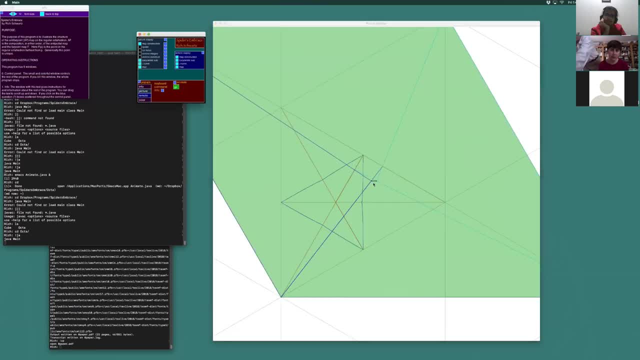 that's, that's sort of a geometric description of the far point map and you can see how this sits with respect to the whole contraption. so it goes around and here it the description changes, but it's the map changes continuously and then when you go through here it's sort of it actually kind of switches from the 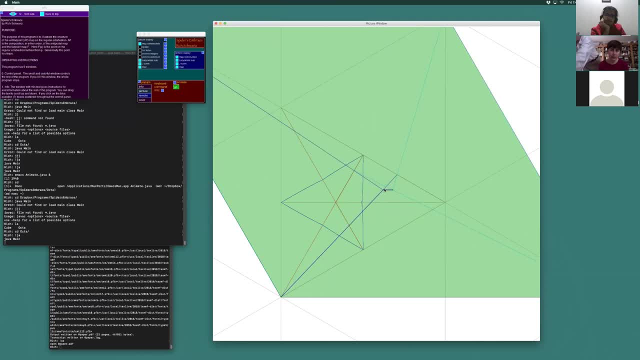 map to its inverse. so so that's the final answer. the far point map on the octahedron. when you compose it with the antipodal map, it's given by this geometric construction. that's like the theorem. but now let me just kind of spend like the last 10 or 15 minutes just talking about algebra and, like I 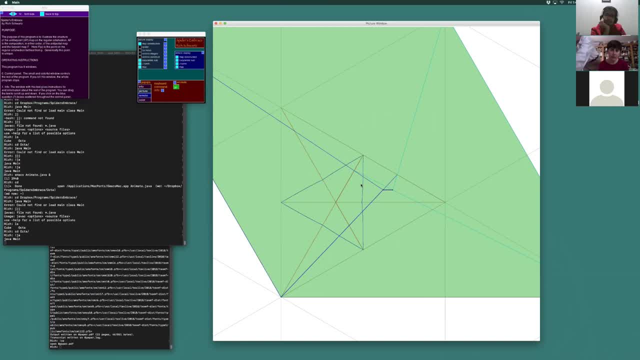 would say that, like the gold standard in a geometric group, in a some kind of thing like this, is to find a nice geometric proof. you know, like when you want to prove the pythagorean theorem, it's: you know these beautiful proofs, and but then sometimes there are these results which 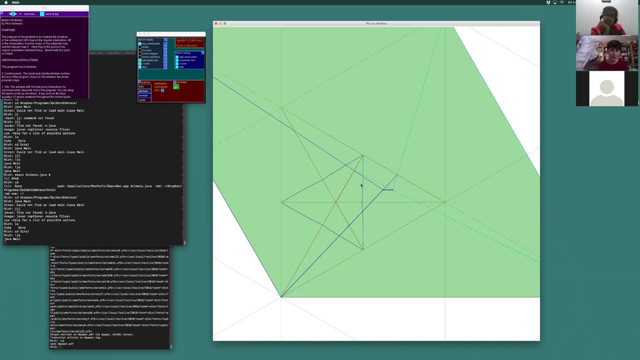 seem to be true, but they're hard to prove, and and so i'm going to sort of tell you a technique to the sort of i caught. you could call it like organized brute force, like how do you prove something algebraically, if it's sort of, even if the polynomials involved are too complicated to? 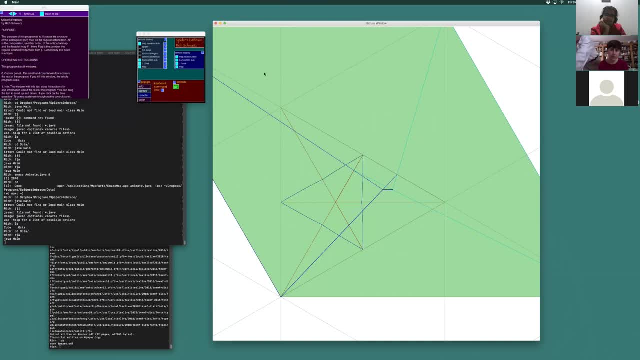 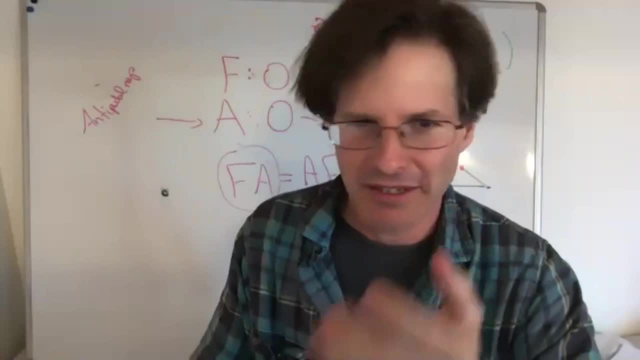 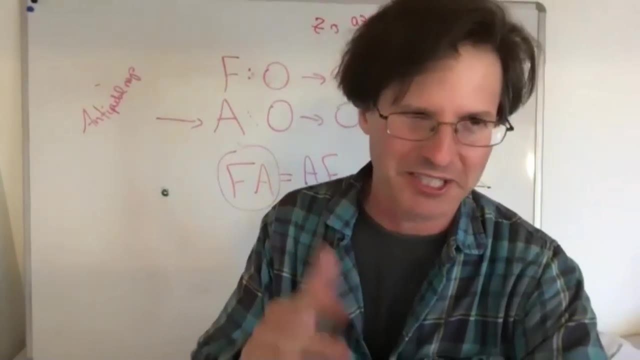 really just solve explicitly. so, um, so i'm going to sort of explain the issues and then um explain this kind of method that i i came up with called positive dominance. but i mean, there's the method i thought of. is it joins a large um host of other methods like this. so so i mean, just i like this. 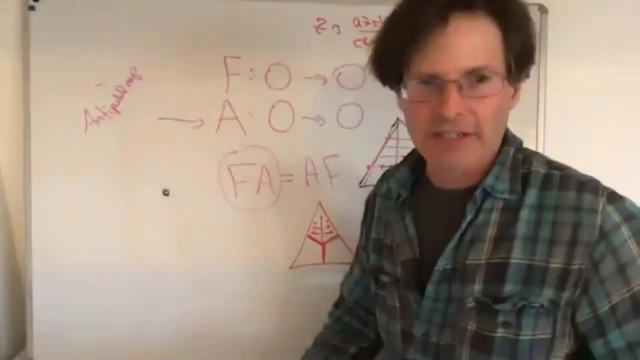 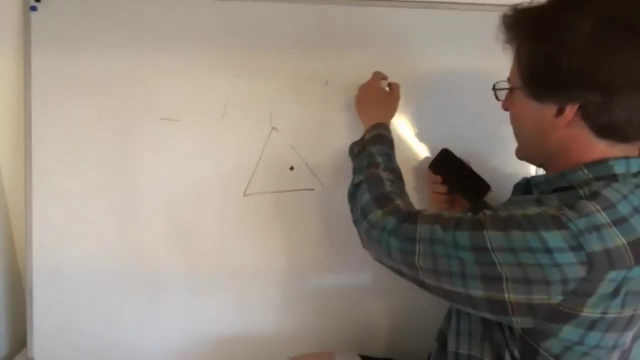 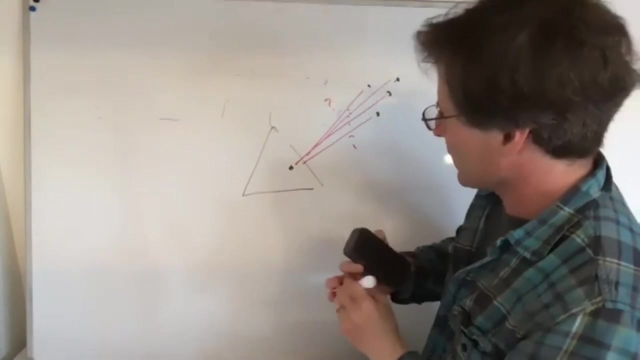 one, just because i'm familiar with it, but there's lots of things like it. so just just kind of abstractly, like again, you have this playing field and you have some point, and then there's this competition between, you know, between the four points. it's really done in, you know, in all the six regions. 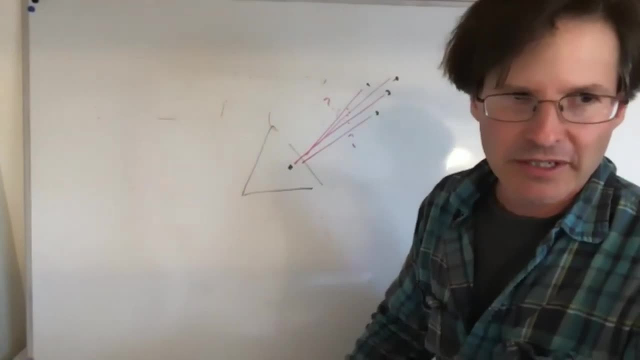 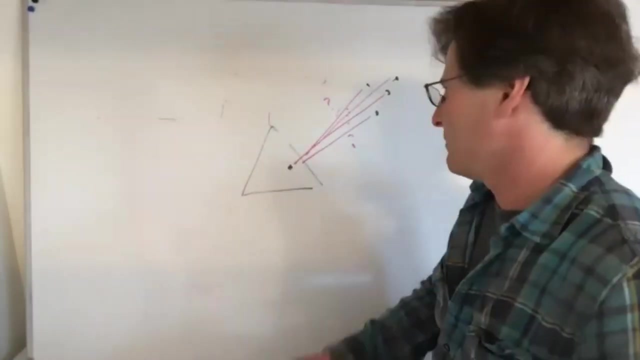 but you're basically trying to figure out which distance is the shortest and you're claiming that a certain distance is is always the best in a certain region, and you know. so you have something like you know, you know sort of like: you know d1, you know d2, etc. 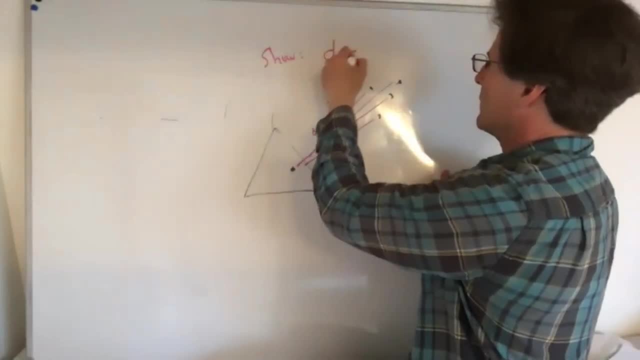 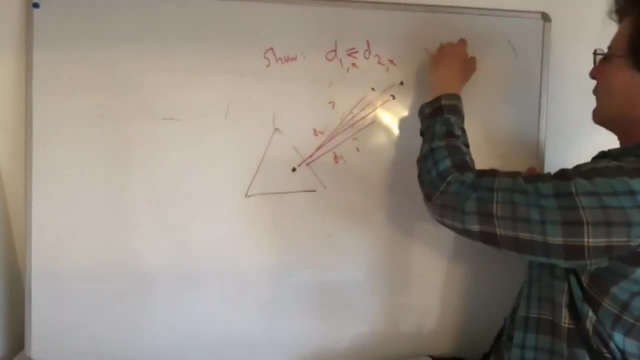 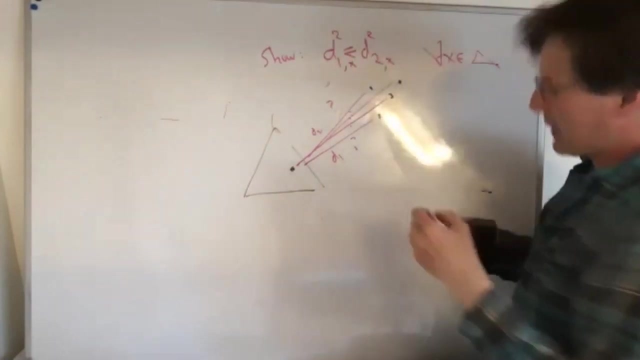 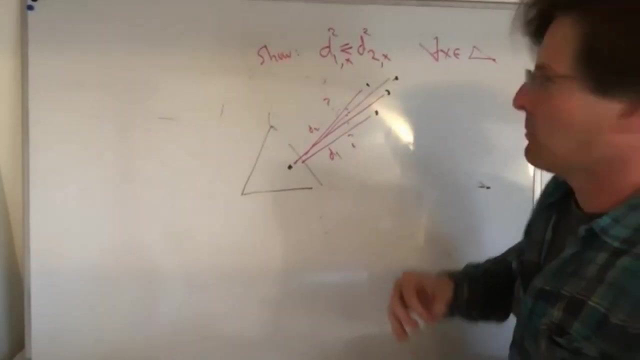 you want to show that like: so these, these depend on some point, x, you know, for all, x in some region. so it's better to it's better to use the squares, because then you, then you get some kind of rational expression in, in x it's just you know, some kind of complicated, several variable polynomial. 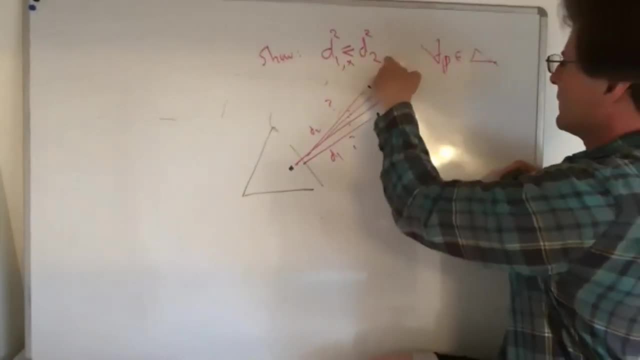 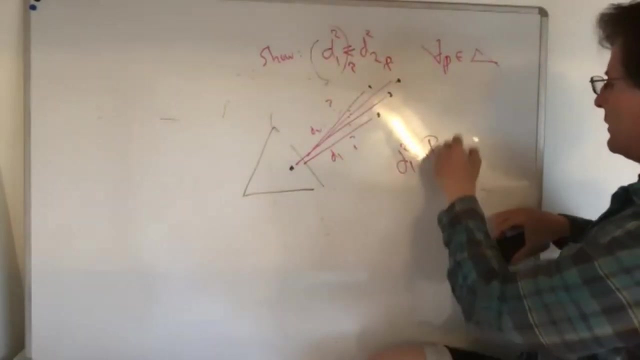 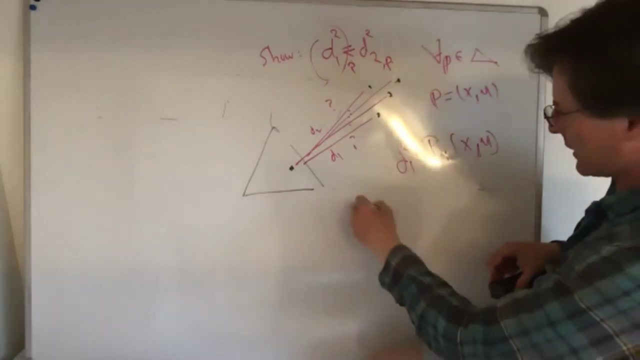 i mean, maybe i should use the point p, so so each of these things, like you know, d, d1, squared is just some polynomial in x and y and and you're trying to show that, like you know, p1 minus p2 of x- y is greater than equal to zero for all x- y in some triangle. 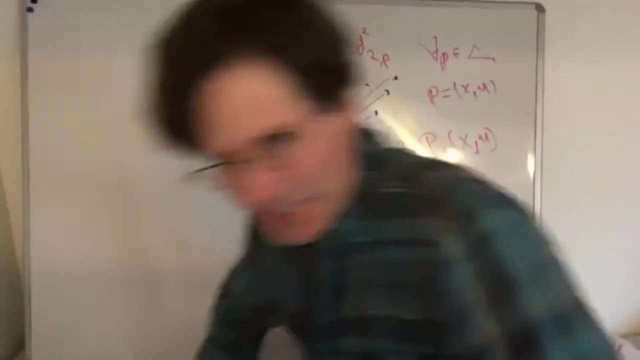 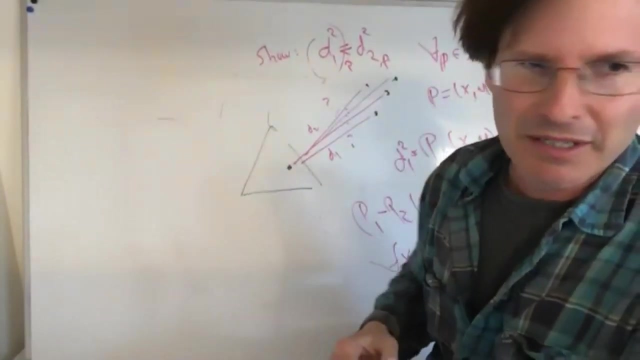 so how do you do that? so this is the kind of thing that you're left with and you know, once you're done, you can then just kind of compute that the map is what it is. but so the question is like: how do you show that? a polynomial. 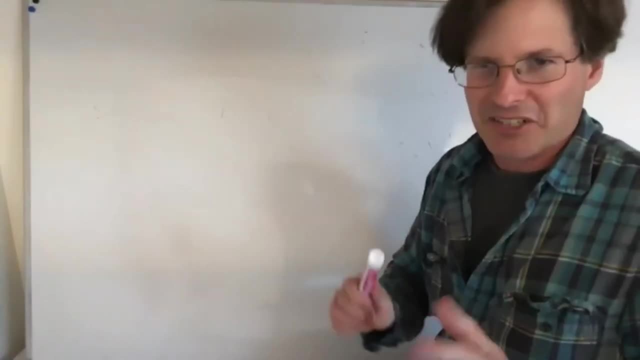 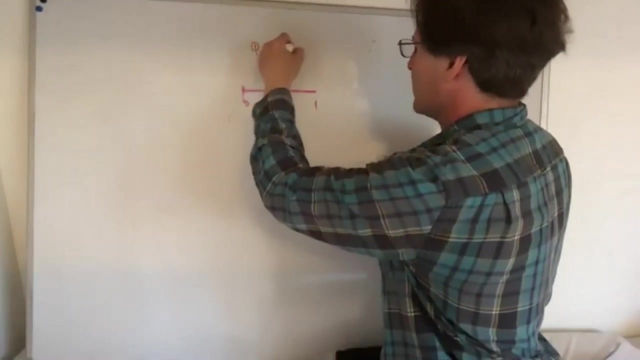 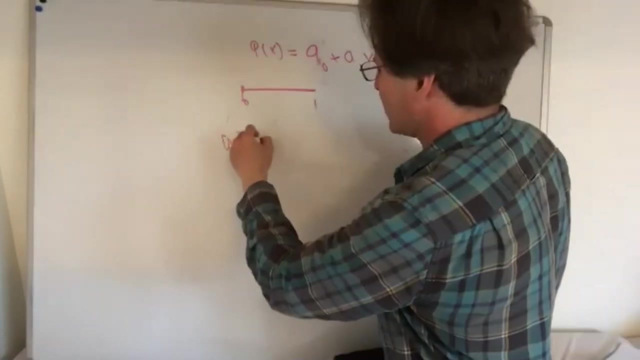 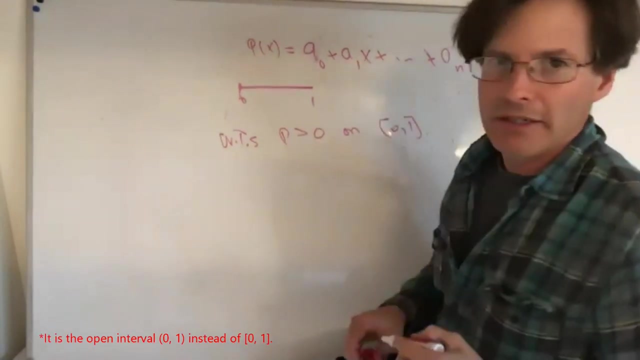 of two variables is positive in a triangle. let me start slowly and let's talk about the unit interval, like, like, imagine i have a polynomial from from zero to one. i mean i, you know p of x is just a0 plus a1x plus. I want to show that p is greater than 0 on. 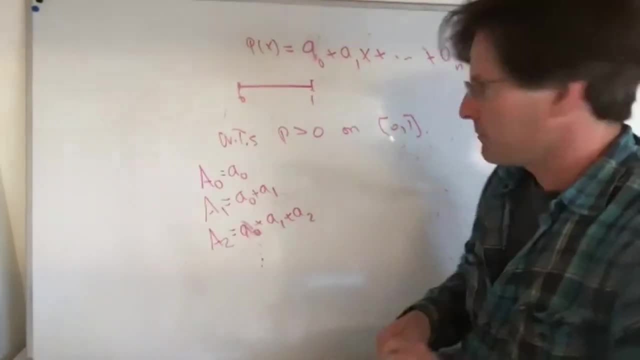 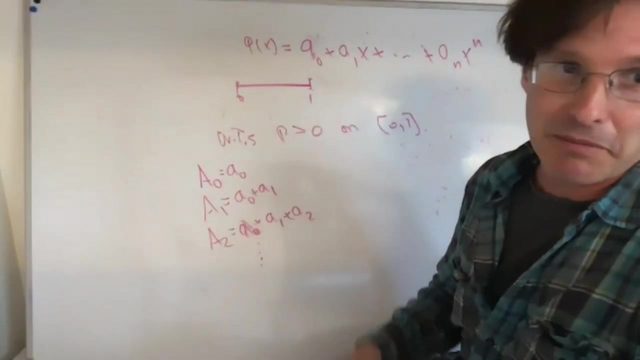 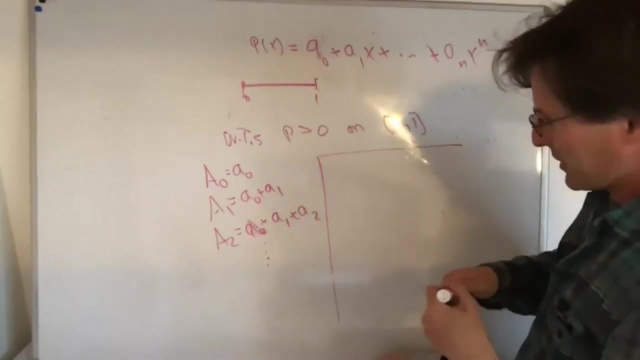 So what do I do? So here's something you can do. If all of these are positive, then the polynomial is positive. Let me give you a proof. So I'm going to try not to botch this proof. There's one idea. 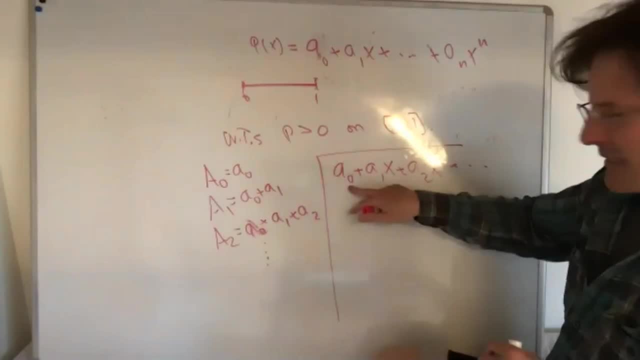 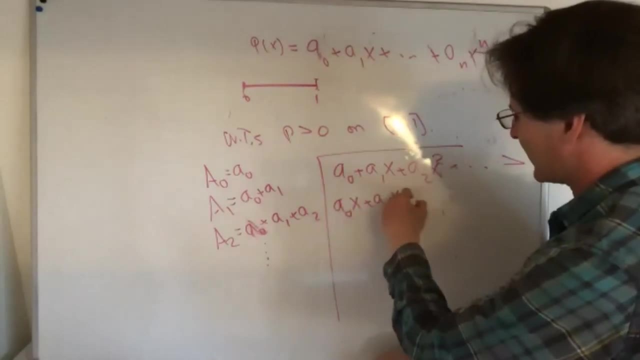 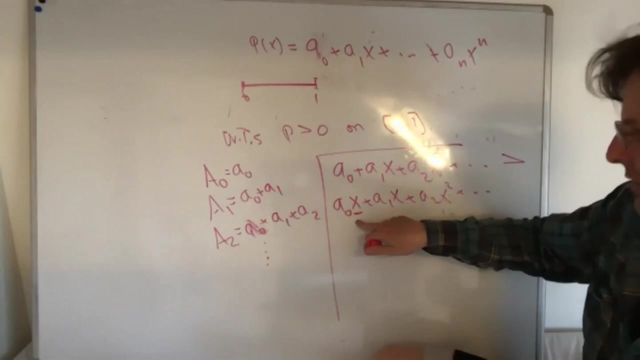 So a0, since x is between 0 and 1, this is greater than a0x plus a1x plus a2x, squared plus, et cetera. All I did was just multiply this single number by x, and I brought it down because this is. 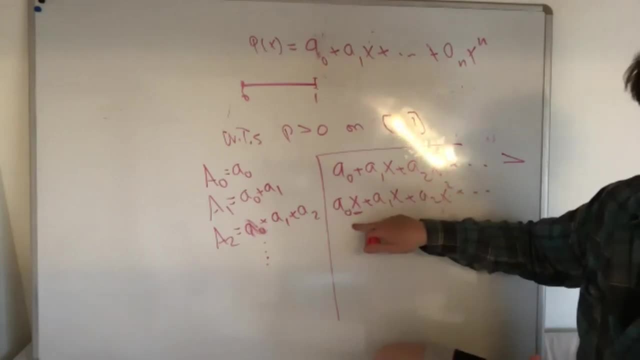 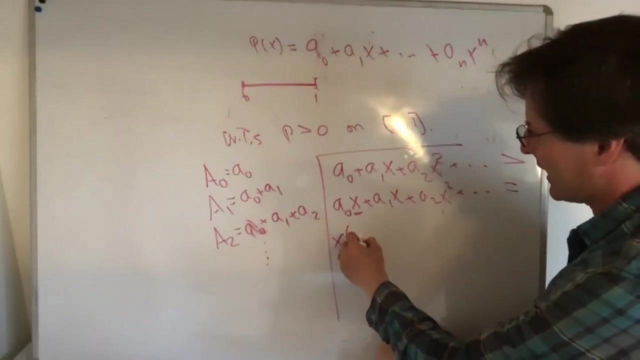 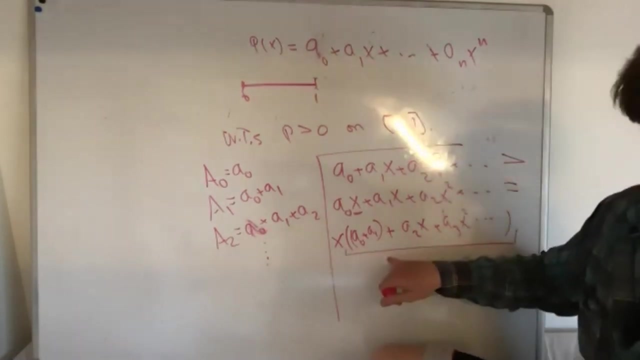 positive. So this is smaller. So far, so good. But this is equal to: I can factor out an x and I get a0 plus a1 plus a2x plus a3x squared dot dot dot. And this polynomial satisfies the same criterion, but its degree is lower. 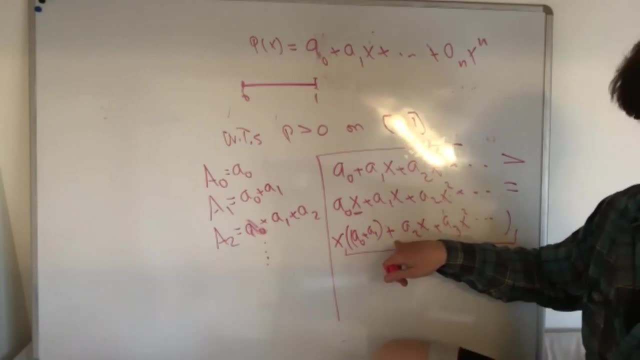 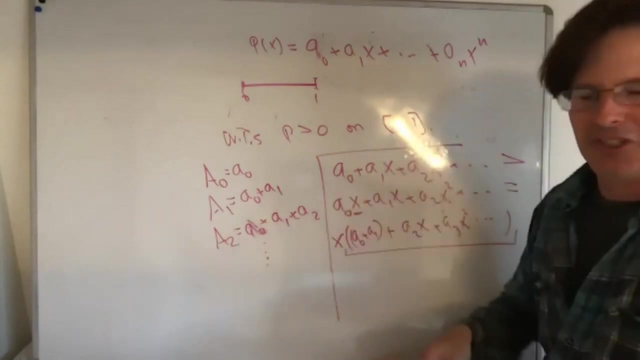 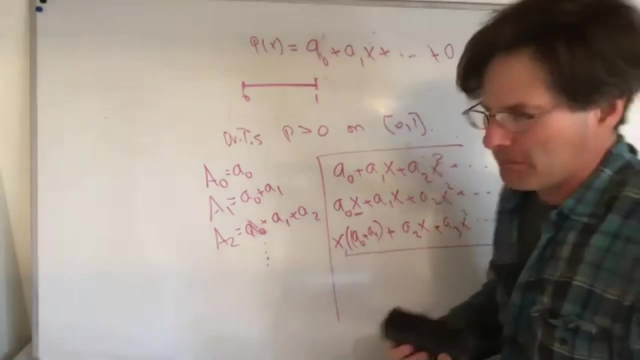 And so this is lower. This is positive by induction on the degree, and then I'm just multiplying by x. So that's a proof that if this criterion is true, then the polynomial is positive. So OK, this is the vanilla version. 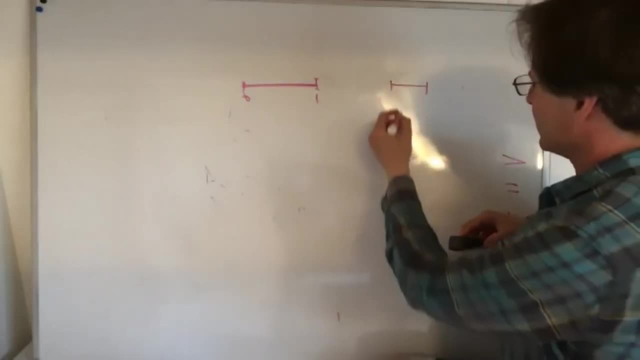 This criterion doesn't always work, but suppose I wanted to show that some polynomial was positive on 0, 1, 1.5.. 0, 1.5. 0, 1.5. 0.5.. 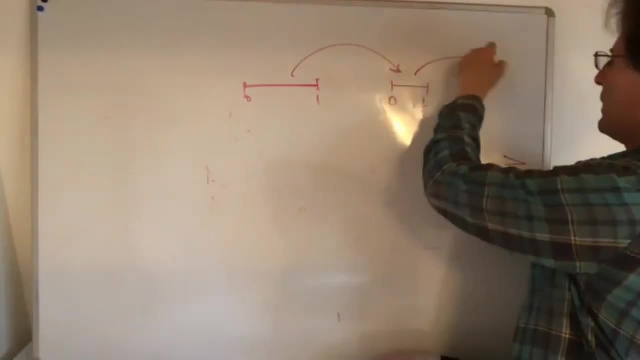 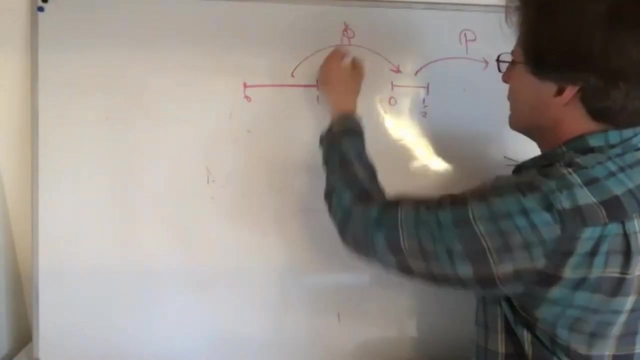 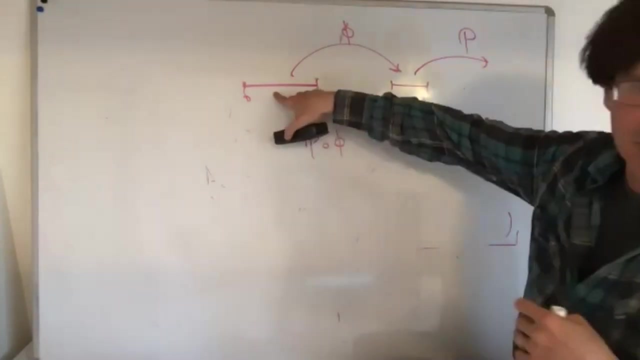 0.5.. So how I'm going to do is I have my polynomial p like this And I have my map here. I call it: say phi, phi just shrinks, And if I look at p composed with phi, that's a polynomial. on the unit interval again: 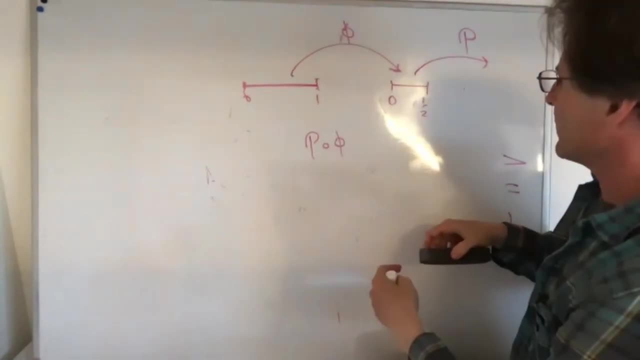 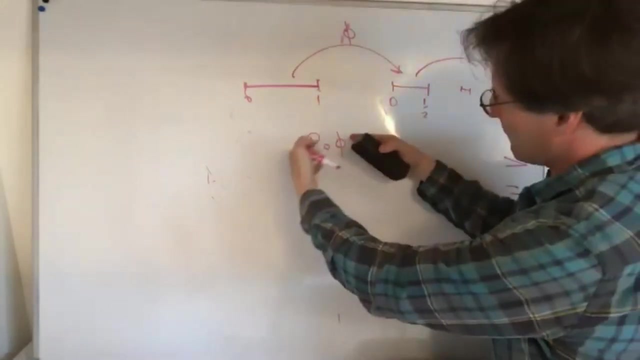 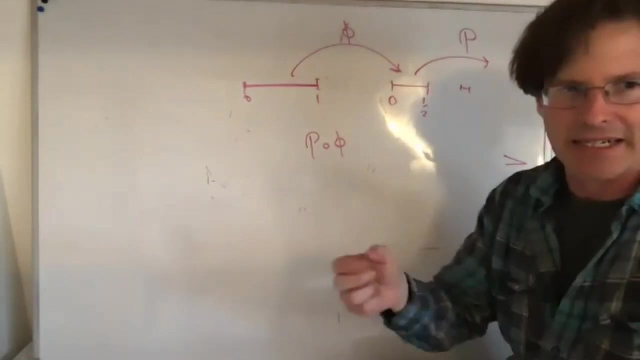 And I can try my criterion Now. Yeah, instead of 0, 1 half, I was using a very tiny interval. then when I, when I pull back the polynomial and look at it here, most of the coefficients are very, very small because, like, I'm taking X and I'm replacing it by X, over a billion, so the 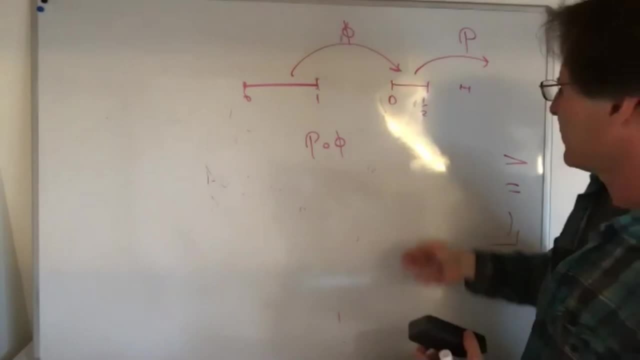 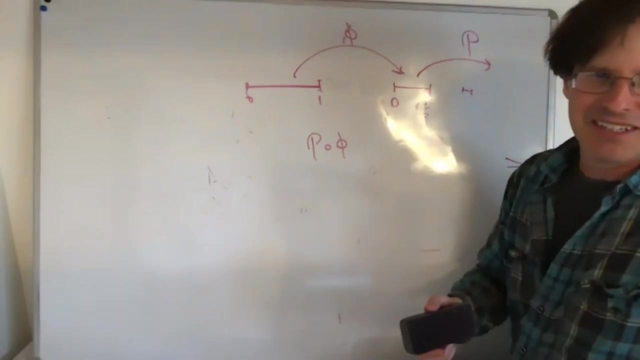 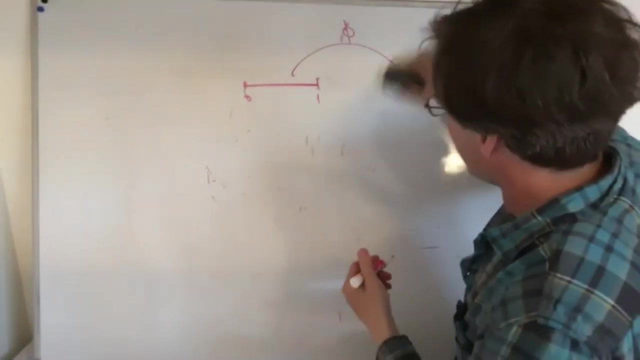 first coefficient is dominating, and so this, this scheme, like if I'm interested in some small piece of this, this scheme is likely to work because I'm likely to be left with a polynomial where I, with it, does satisfy the criterion. so the idea is that if I want to know if a polynomial is positive on the unit, 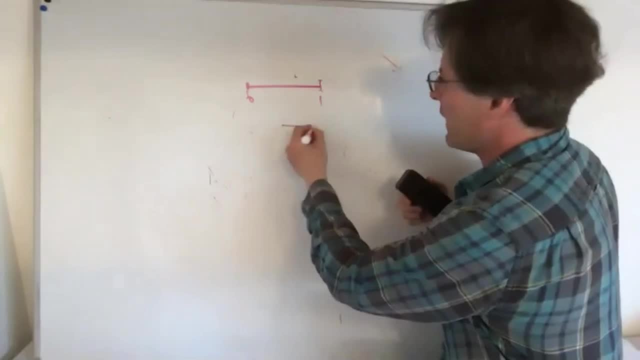 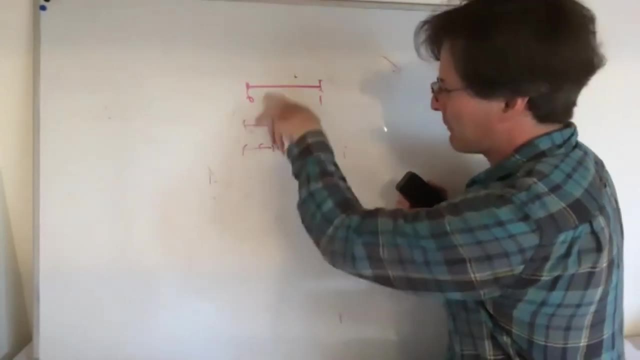 interval. I try my criterion. if it fails, I subdivide the interval in half and I try it on each of these and then I just go through and I do like a depth first search through the intervals and I just go down and when I finally succeed, I you. 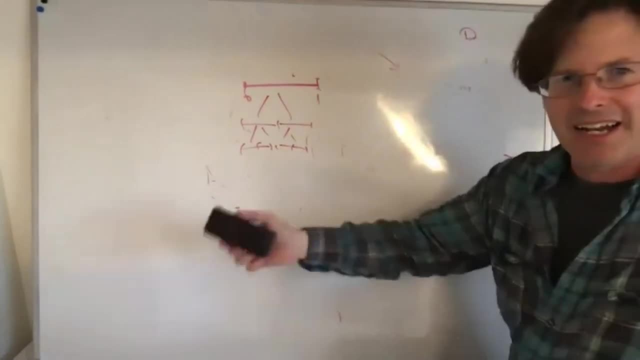 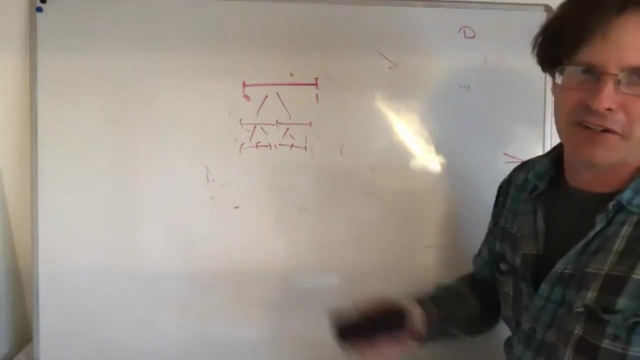 know, I have this kind of tree and and I run through it and when the whole thing halts I can't do anything about it. I've proved it's positive. so this is a this thing. it's if. at this algorithm halts if and only if it's positive. so it's very robust. um, okay, but I wasn't. 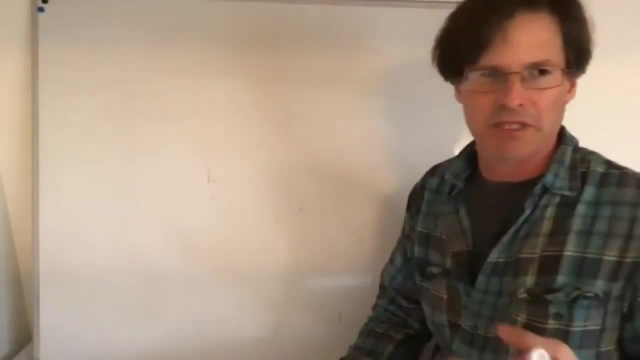 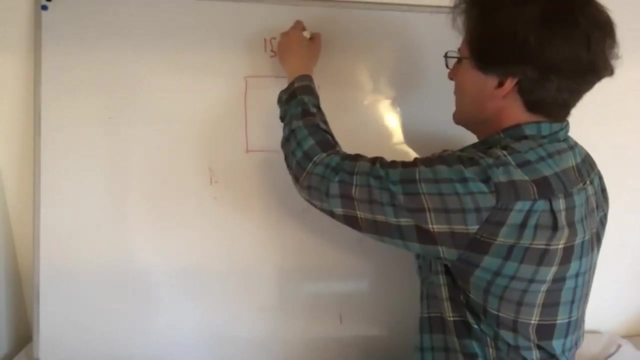 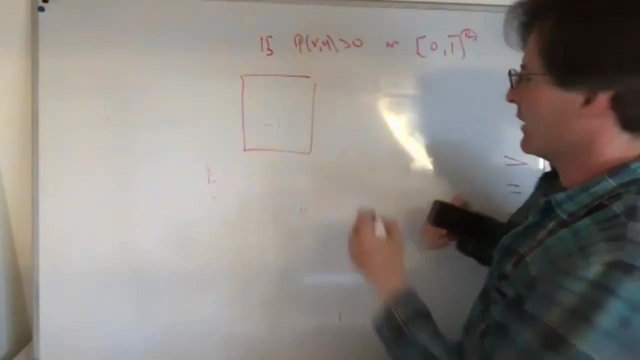 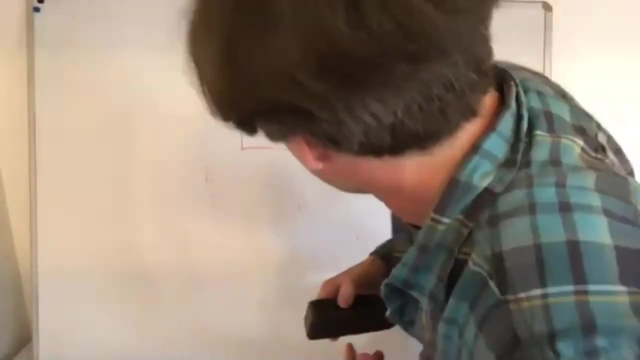 talking about polynomials of a single variable. I was really talking about polynomials of two variables. so suppose I I want to know like: is P of XY positive on 0, 1 square? so what I do is I I write out all the coefficients. sorry, I take my polynomial. I write it out as like: 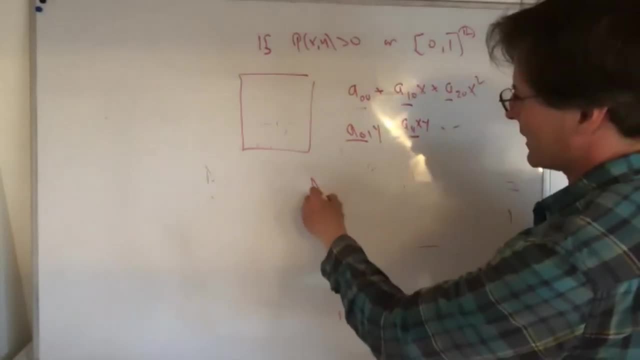 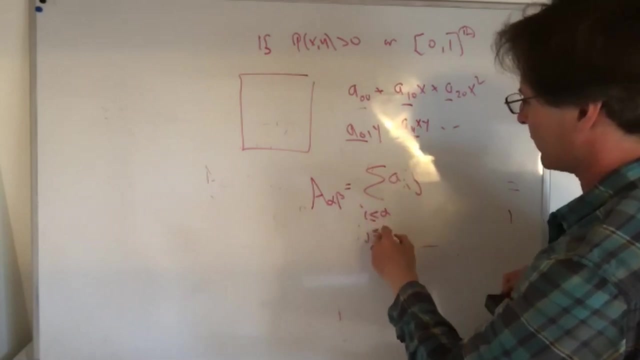 an array and then then I make these things like a alpha. beta is like the sum of all a, I, J, with I less or equal to alpha, J less or equal to beta. so I I put my finger somewhere and I just sum up all the things going to the left and and. 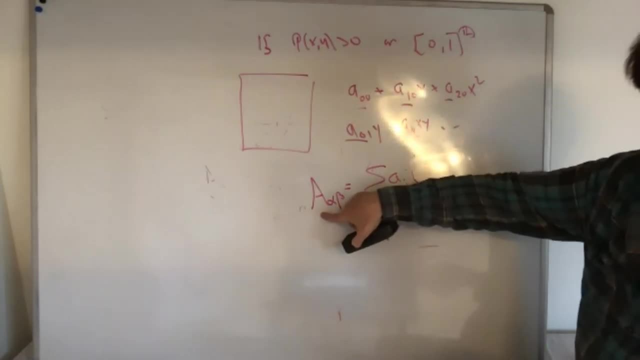 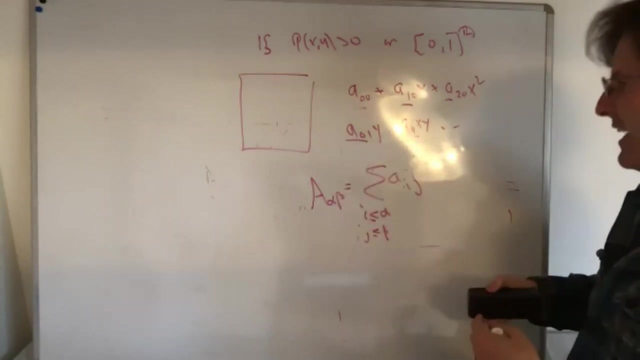 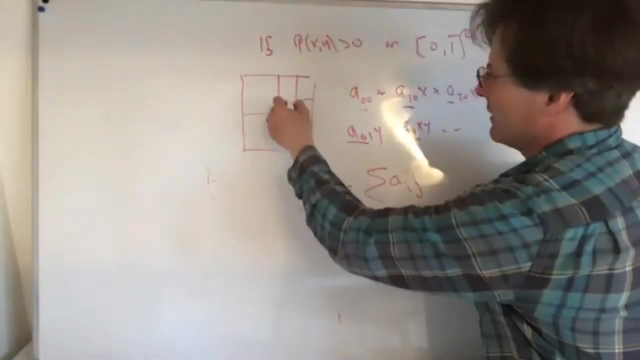 up, and if all of these are positive, then we're good, it's, it's the same kind of argument, it's positive, and if this fails, I can kind of divide the thing up into quarters and retry it. so again, there's a kind of a subdivision algorithm which will, which will verify it. so 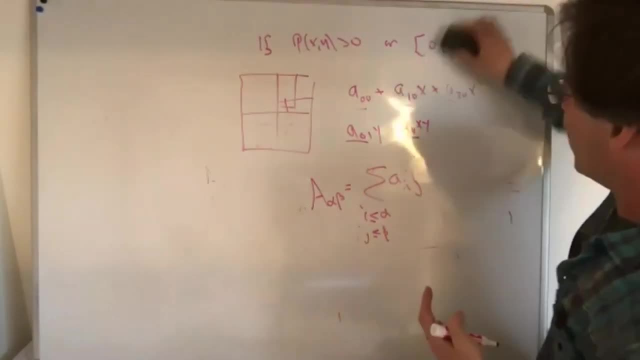 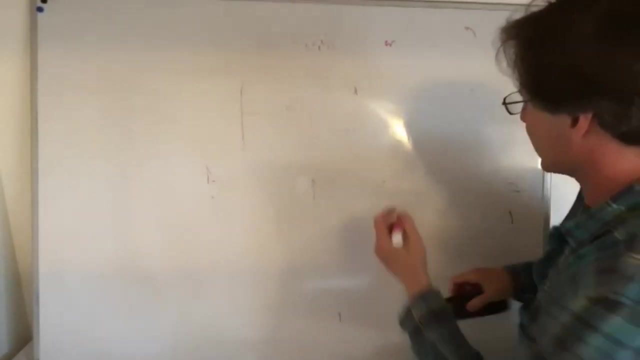 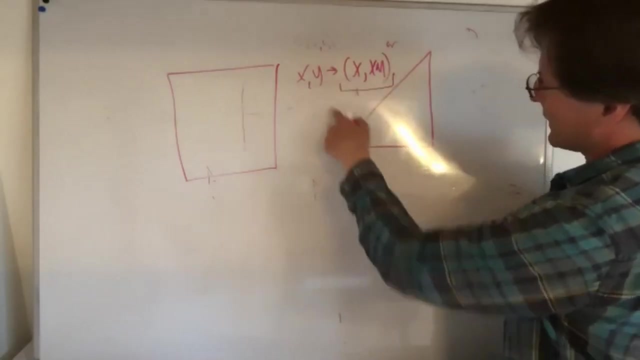 okay, almost done. um, unfortunately I don't have a square. I have a triangle, like. like, let's say I have a square and I just say I'll do a square. so I take a square and then I give it to a small triangle. the triangle like this: If I look at this map, xy goes to xy. this is a polynomial map. 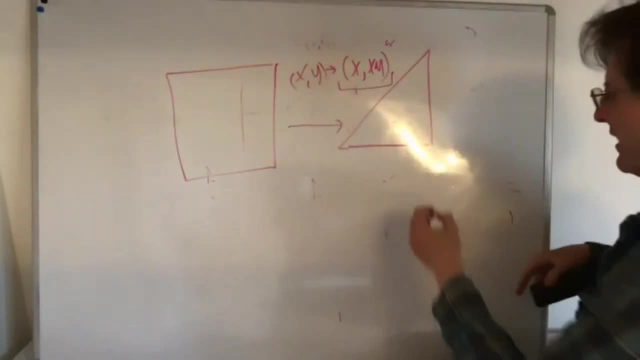 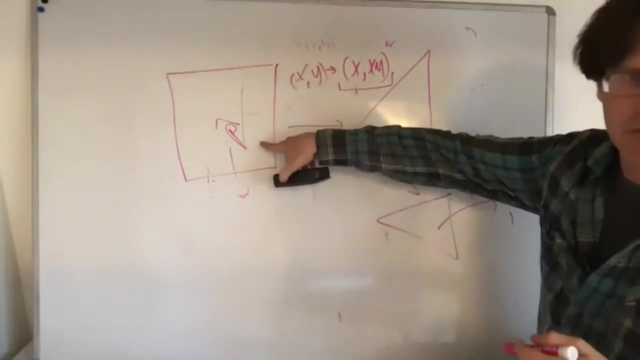 from the square to this triangle. Then if I have some other triangle, I can take some linear transformation. If I have a polynomial coming out of here, I can compose it. and get a polynomial coming out of here, Then I can try to use my subdivision algorithm If I 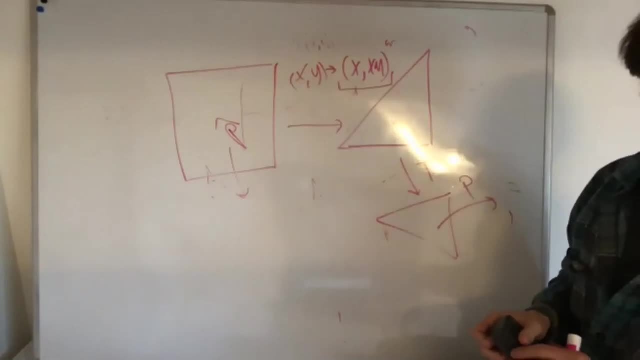 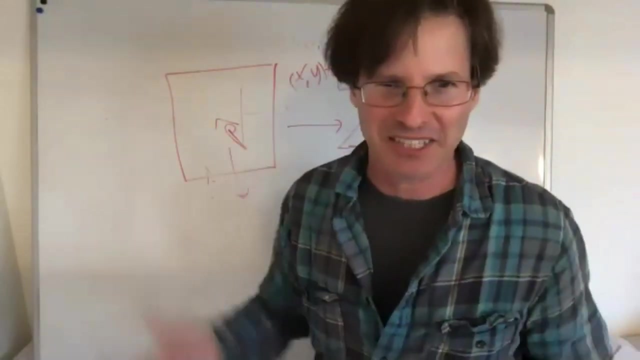 can show that this thing is positive. it implies this thing is positive. That's what I did. I just set up the maps, I got the polynomial on here and I just checked the criterion for every polynomial on site. That's how I proved that- the vertex I thought. 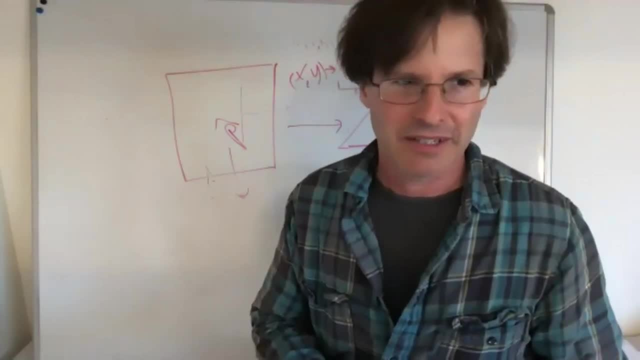 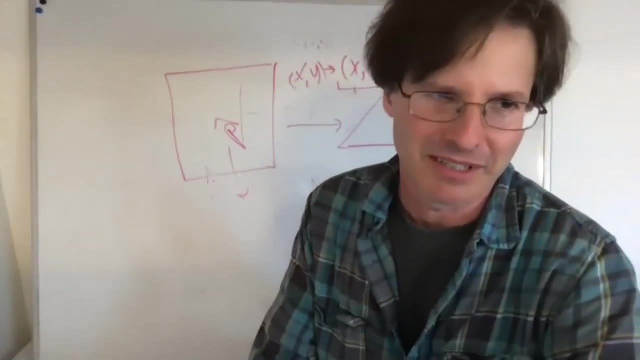 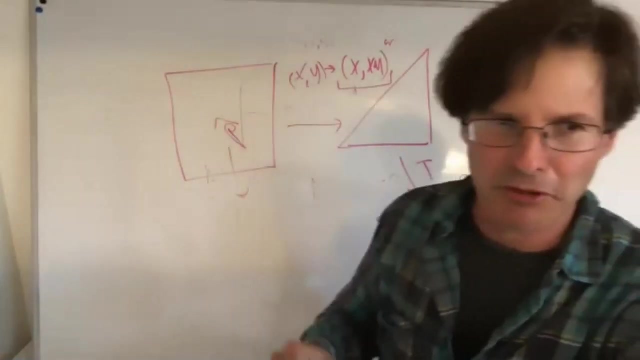 was the winner in all cases was the winner. Then, once I have the winner, I just compute what the map is. That's the end of the story. The idea is that the polynomials you get in trying to prove this are slightly too much. 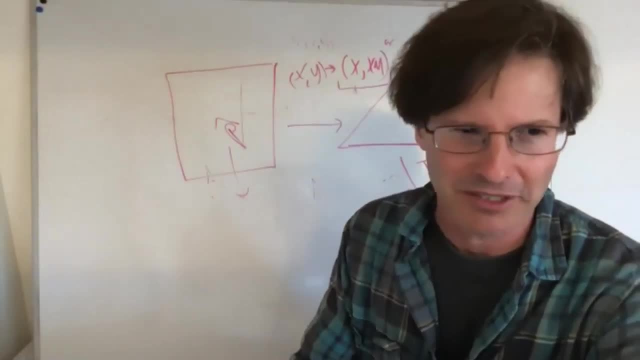 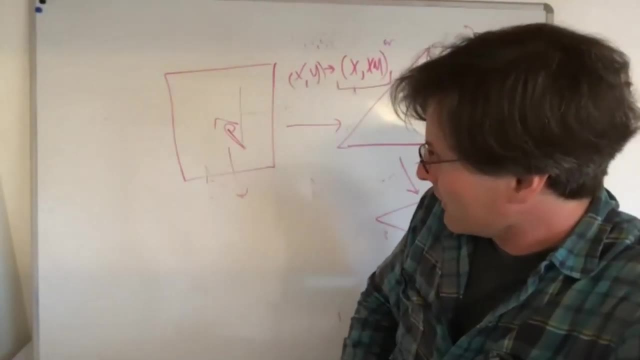 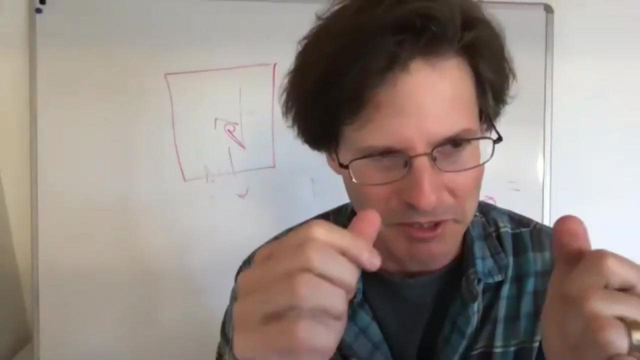 to do by hand, unless you're really good at algebra. Being lazy, I just use this method of positive dominance. This is kind of big business in computational algebraic geometry. You have some polynomial and you want to know it's positive on some region. What do you? 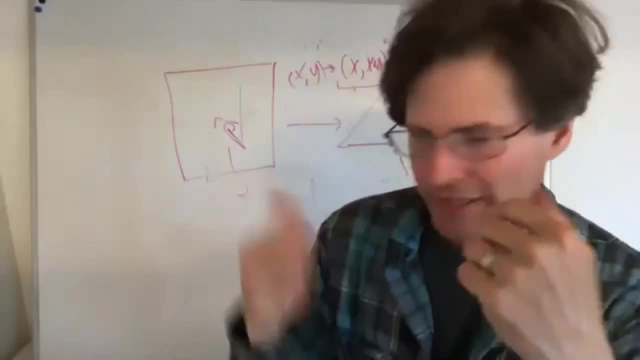 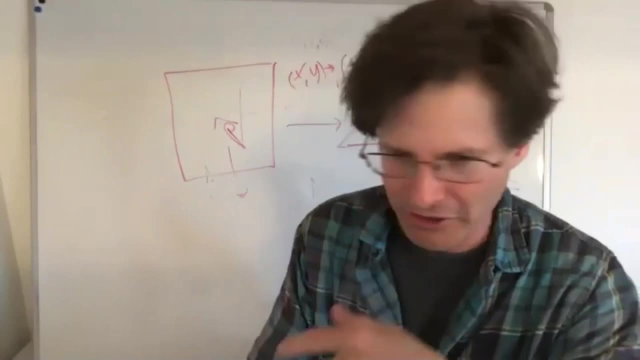 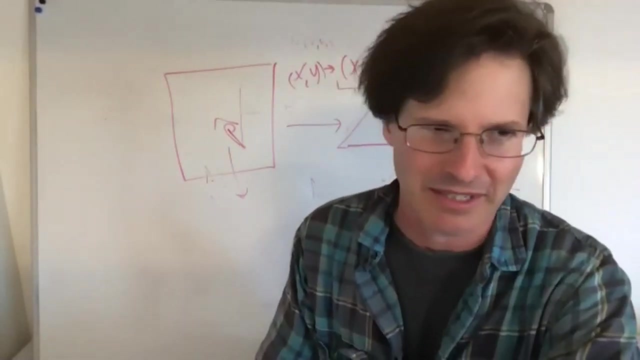 do. You could do this. This will work in n dimensions. There's some generalization. You can try to write the polynomials as sum of squares of other polynomials. There are various things that people try with more mixed success. At some point I thought of this thing and I like it because it worked. 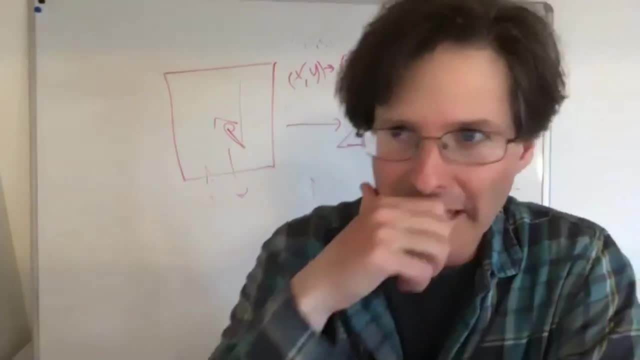 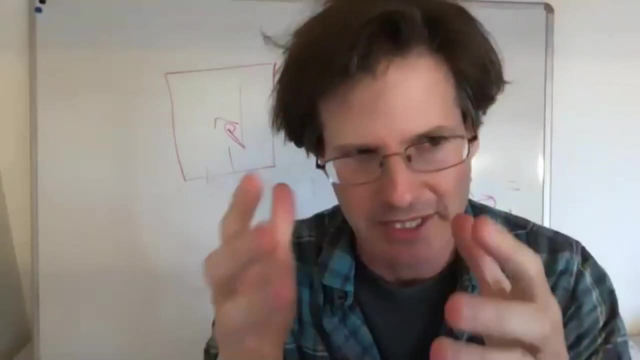 once and it worked many times. Anyway, that's the end of it. What I want to say is that the same sort of thing happens on the cube, and it's easier. more or less the same. I'm embarrassed to say that I actually don't know what happens. 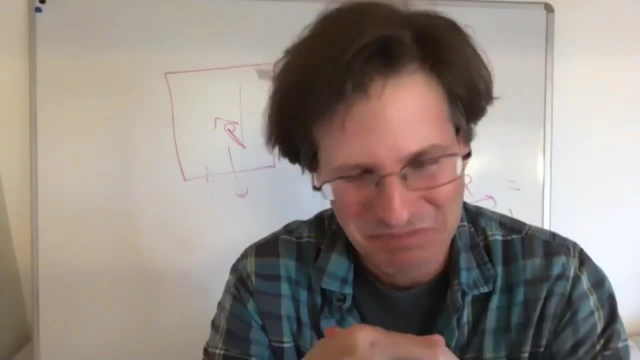 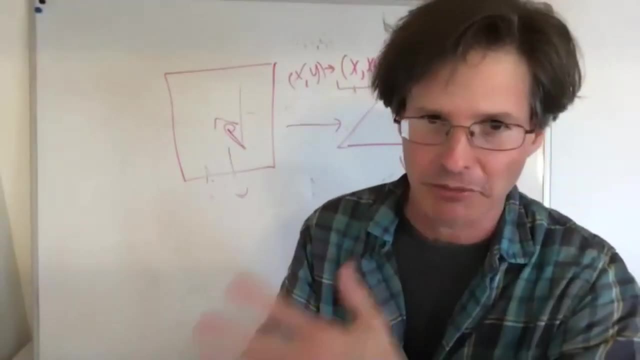 on the tetrahedron. You'd think I would have done that case first. I wasn't able to find it in the literature. What's better about the cube and the octahedron is that they have this antipodal map It makes. 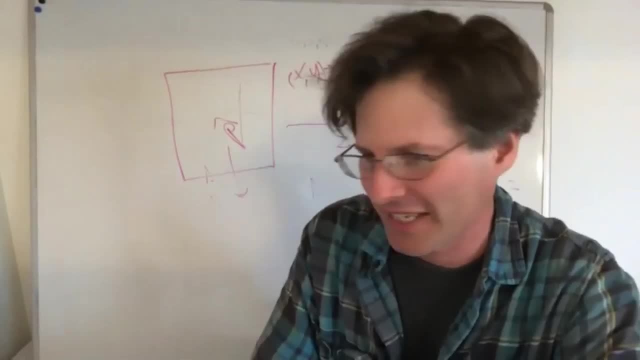 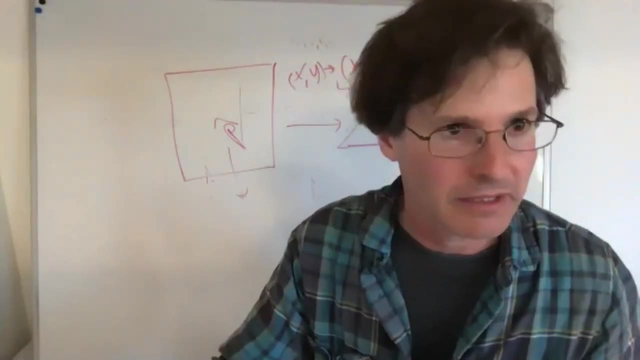 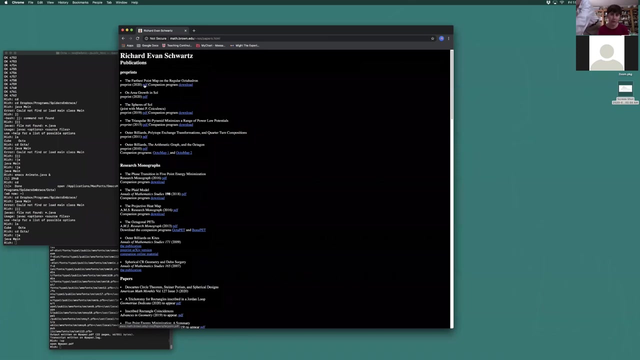 it nicer. Probably it's a nice answer for the other platonic solids. I just didn't work it out. Let me just show you a link, Then this will be the end of the talk. That's my website. If you go to publications and you click on this, you can read this paper. It's got all. 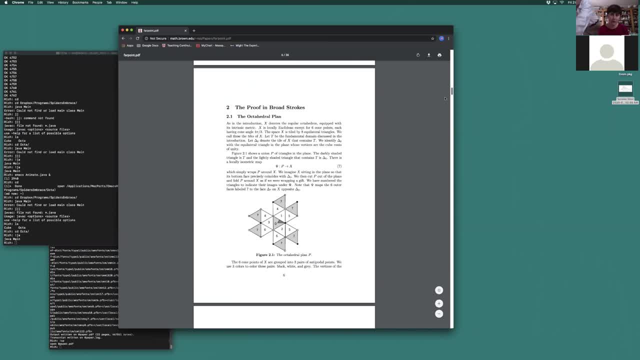 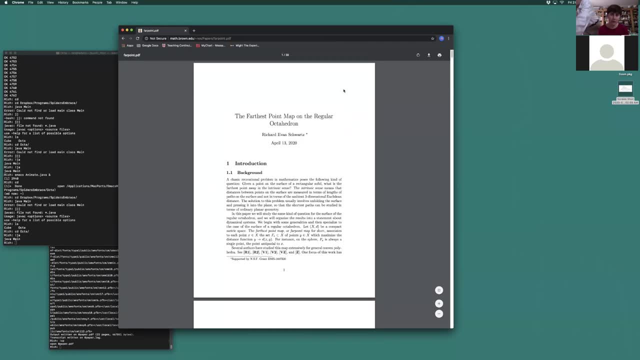 those pictures. Basically, I just took the program and put it into the paper. If any of you guys is interested in this, you can read about it here. I didn't talk too much about this in the past. There's a bunch of references of other 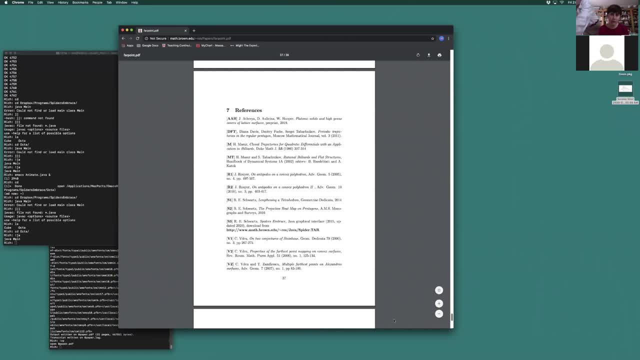 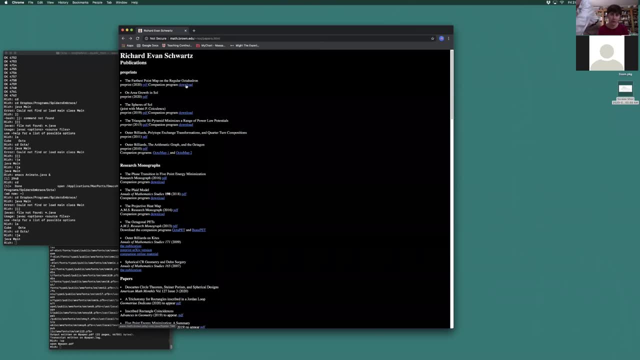 papers in the back. If you're interested in other things about this, there's places Then. the last thing is that if you can click the download and this will give you the program, you can try to use it. If you have a Java compiler, you can run it. 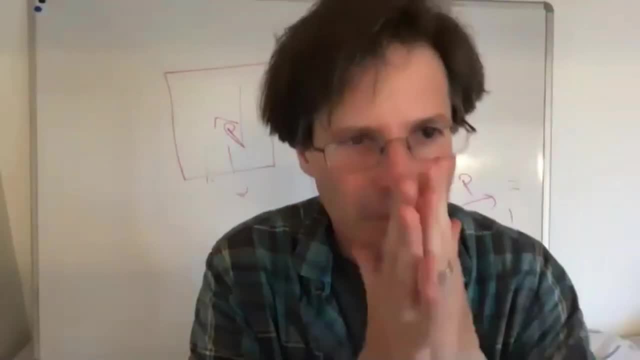 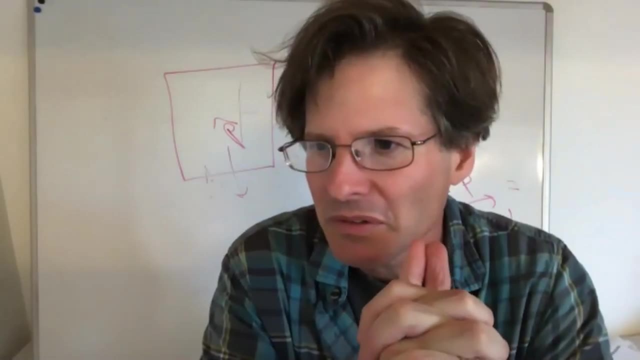 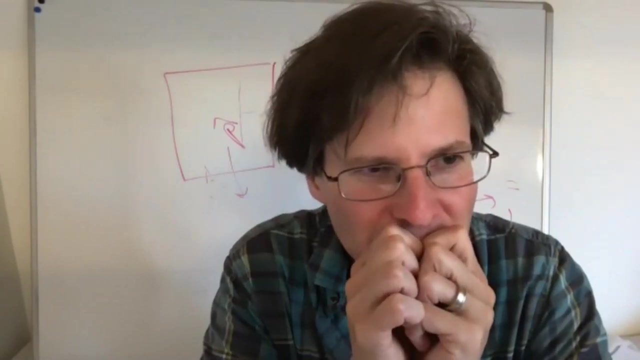 Yeah, so that's it, Thank you. I just had a question. When we got the J shape, did you have to do anything else? No, Is that directly obvious that we should divide a fundamental triangle into two parts, rather than say more? 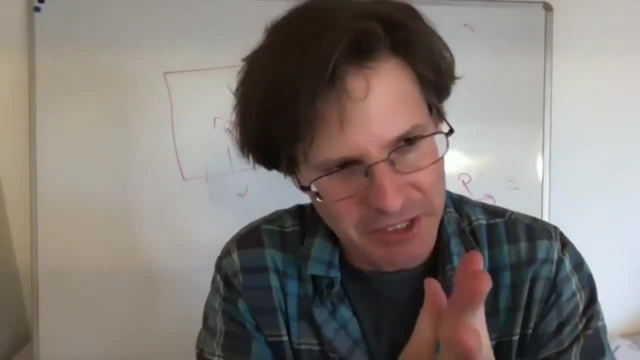 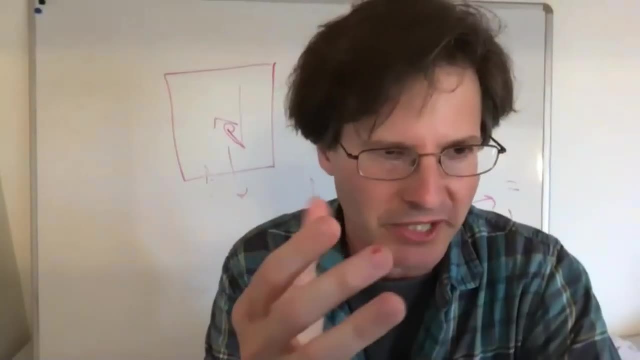 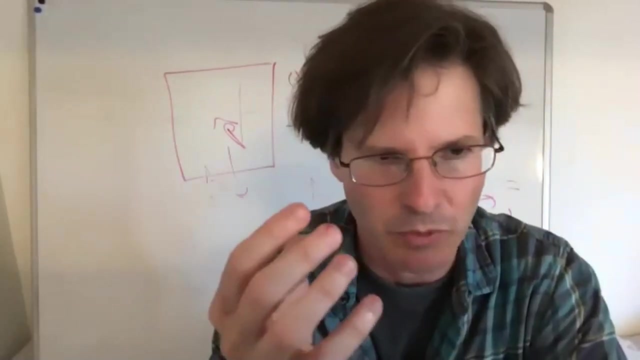 No, Let me tell you something about that. That's a good question. I had a PhD student named Zili Wang. Zili looked at this on more general kinds of octahedra. All the cone angles are supposed to be the same as the regular one and it should be centrally symmetric. 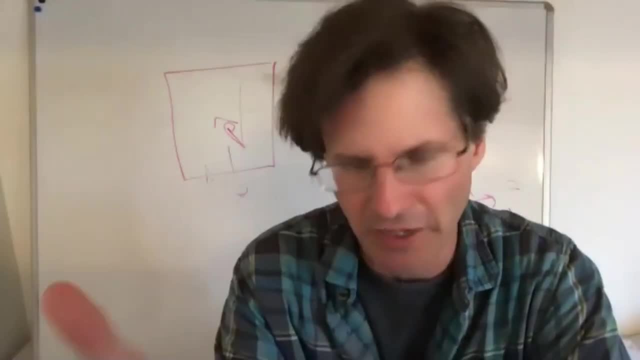 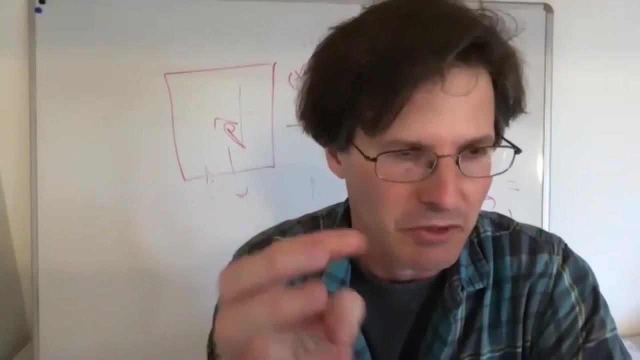 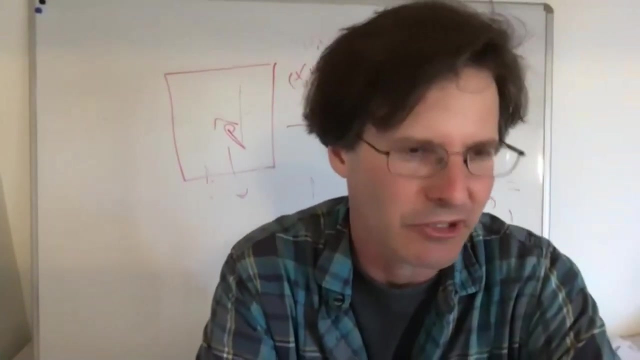 But otherwise It's not. It's not. And then she also tried to find these various regions where the thing splits apart And basically it looks like a mess. So if you go away from the regular octahedron there's many different zones and stuff. So I'd say the answer to your question is it's. 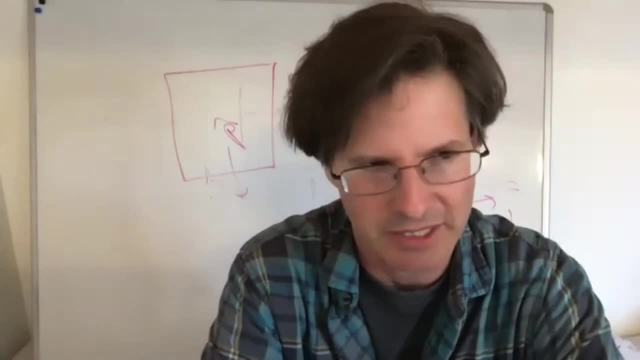 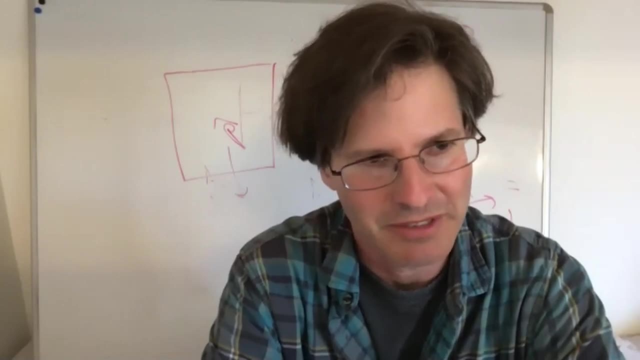 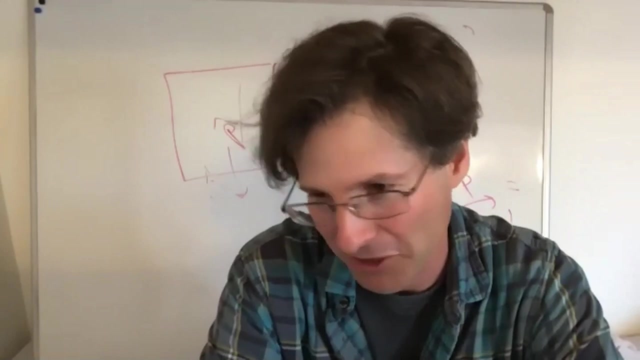 not obvious at all And in fact, for more general things it doesn't work that way. It just somehow is very clean for the regular octahedron. This is why I thought this would be a good project. I was hoping like, oh, there's going. 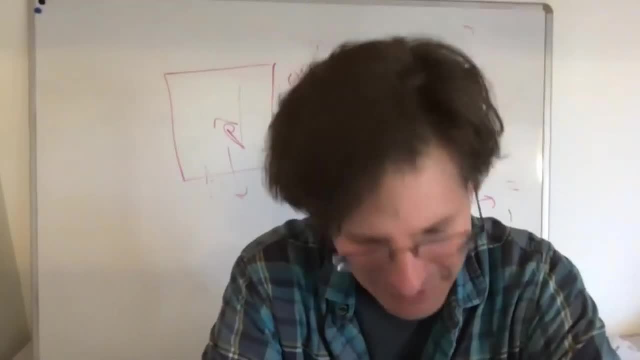 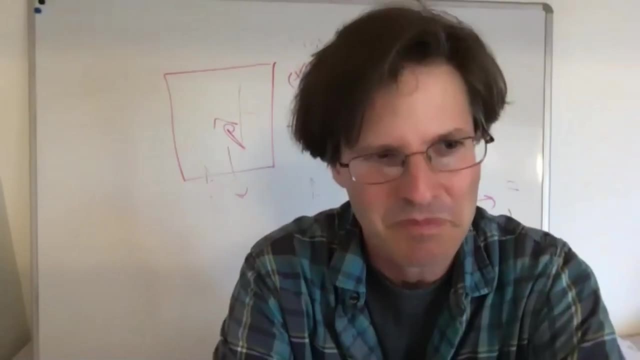 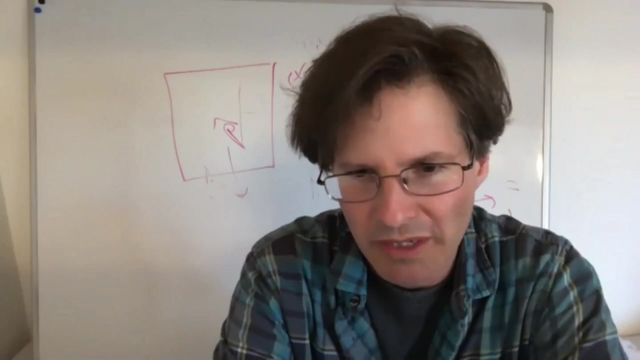 to be some beautiful answer for the general, like a more general thing. But I mean, it turned out to be pretty cool, but it didn't have the same crisp sort of feel to it. Yeah, Thank you. Sure, Are there any other questions? 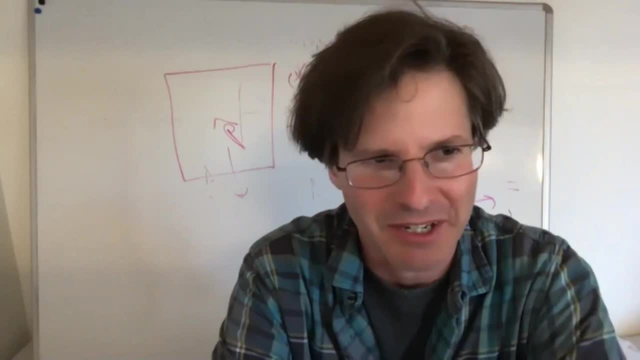 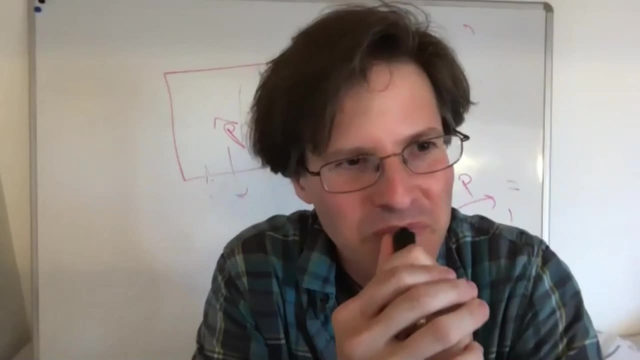 Yes, I hope that made sense for you guys. Yeah, Yeah, I guess there's other new questions. Let's just thank the speaker. Thanks, It was. this was really interesting. Yeah, And because we slightly messed up and didn't introduce. 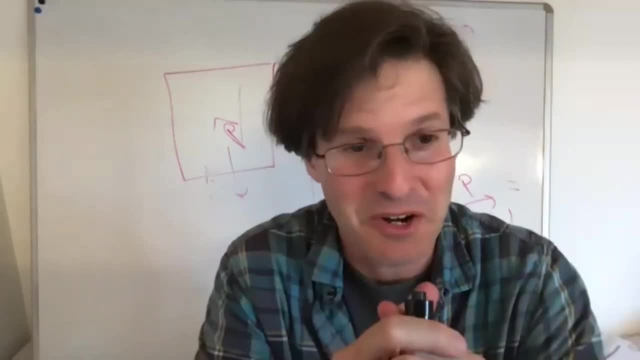 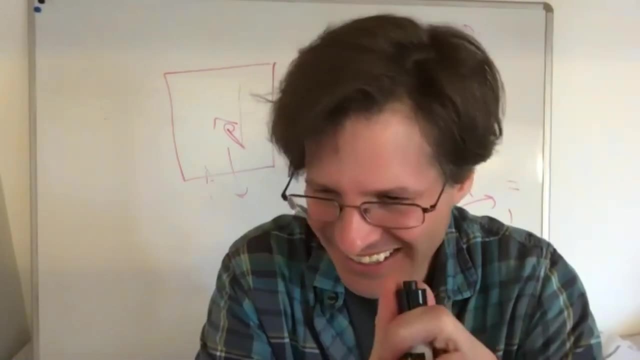 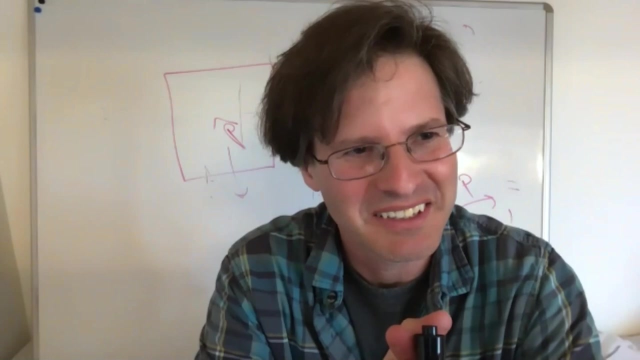 you at the beginning, sorry about this. Just so that everyone knows who this was, This is Professor Richard Evans-Schwarz. He's a Chancellor's Professor at Brown University And, as you can probably guess from the talk, he studies geometric group theory And he 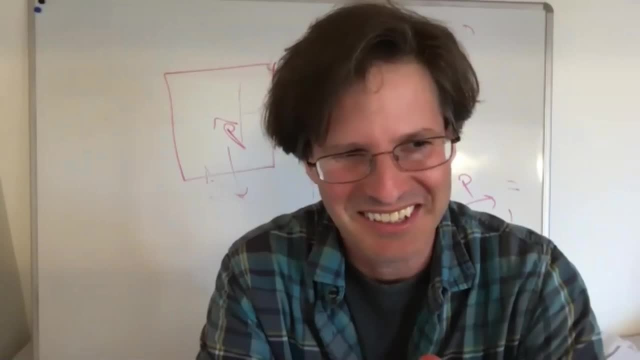 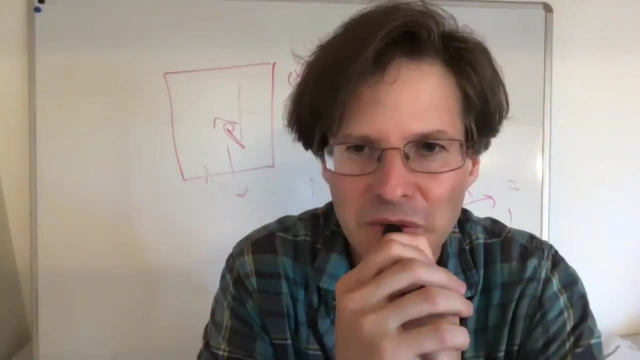 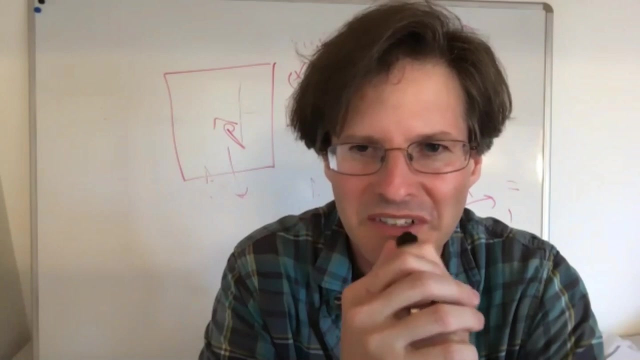 also writes picture books about maths. Yeah, that's right. Yeah, that's right. Actually, I had a question: What happens when you look at different polyhedra? So if you looked at like other regular ones, like, I don't know, like a dodecahedron, 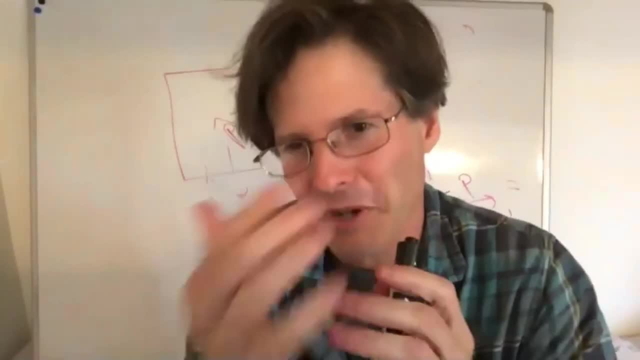 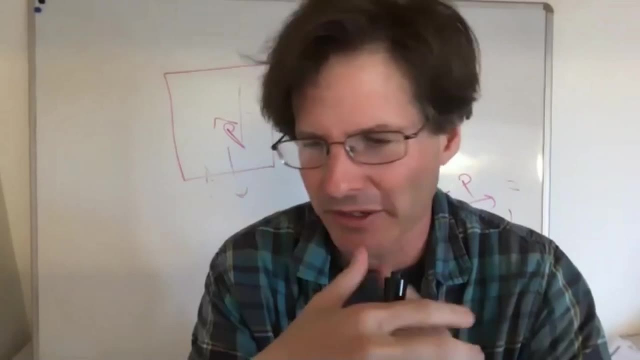 Right, Yeah, That's a really good question. So so for the cube: okay, So for the cube, the answer is somewhat like like what I described for the octahedron, but a little bit simpler For the icon. 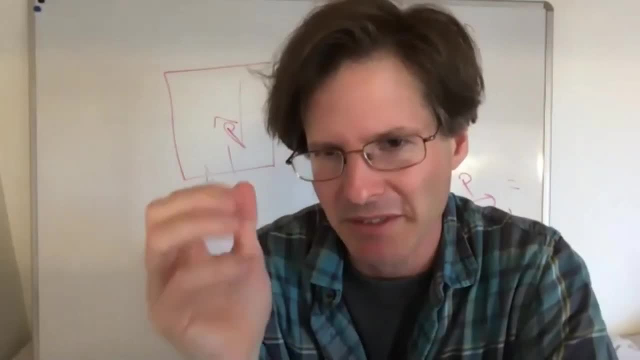 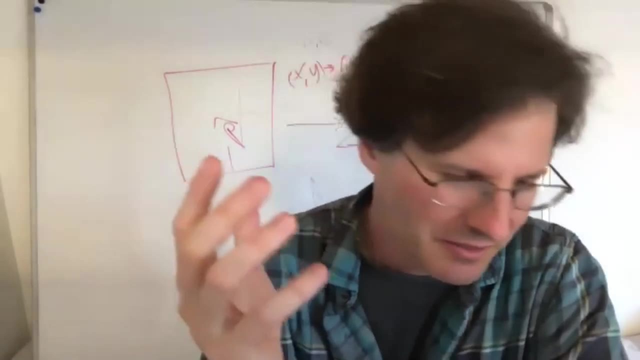 Okay, For the dodecahedron it should be about the same as the octahedron. For the tetrahedron it shouldn't be too hard to figure out, but I don't know the answer For the dodecahedron. 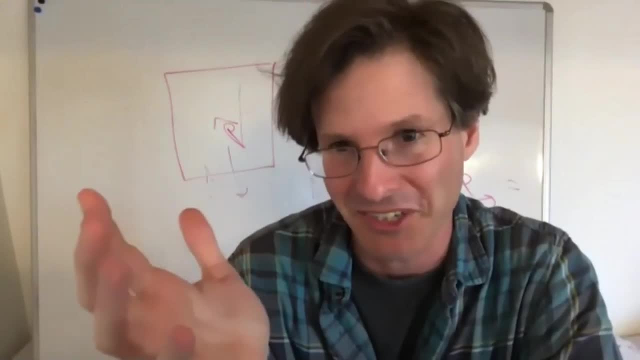 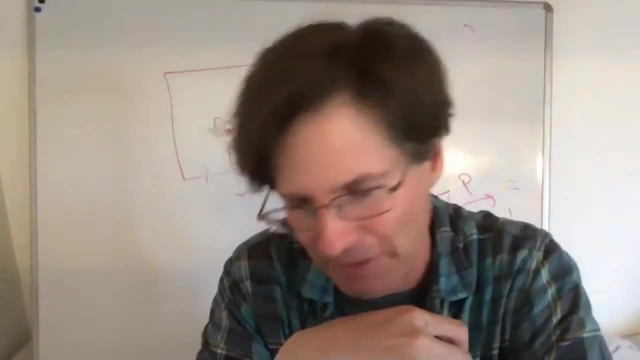 I just have no idea. Like that would be a really fun one to do. actually I think people kind of don't know. But you know, I thought about trying that. I mean I'm not, I'm not sure if I will, but but and and then the other case I was saying is that my, you know. 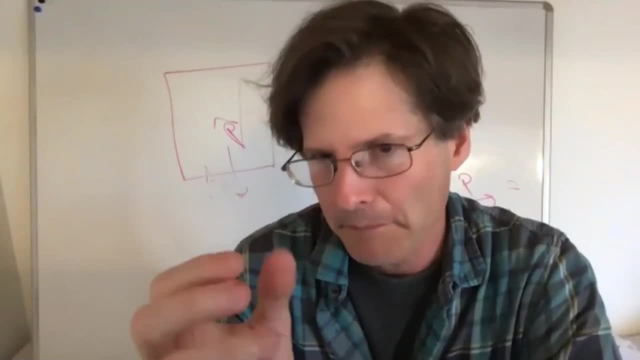 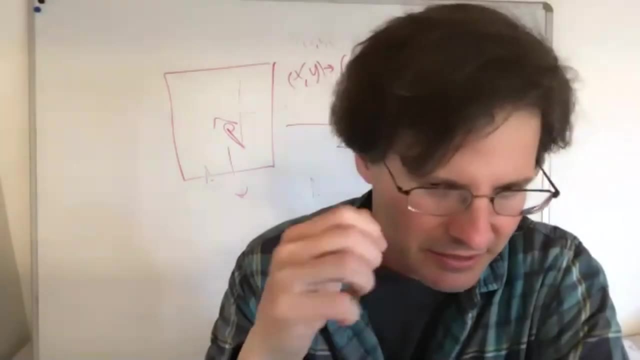 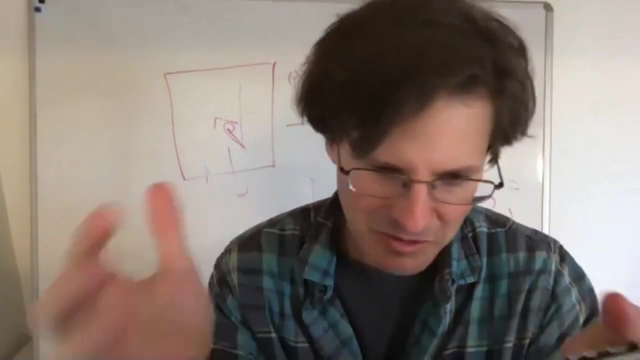 the other case I was saying is that my graduate student, Zili Wang, she she looked at other octahedra, other centrally symmetric octahedra, And she, you know I'd say she proved some of the same things that I proved in this case, but but sort of more general and less specific. 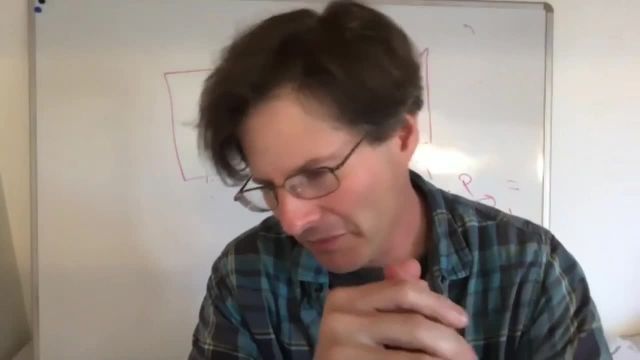 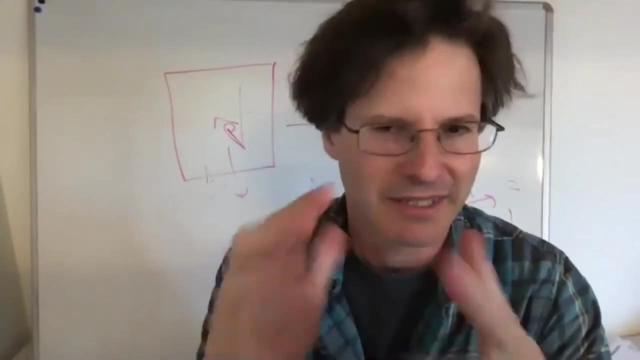 you might say: But you know, I kind of like these kinds of problems where, like you have a family, like you, could look at all possible tetrahedra and you could say like this is the map. and you could say like how does the map change as you vary the tetrahedron? 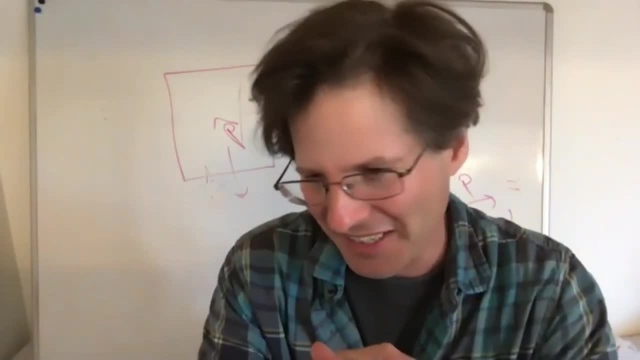 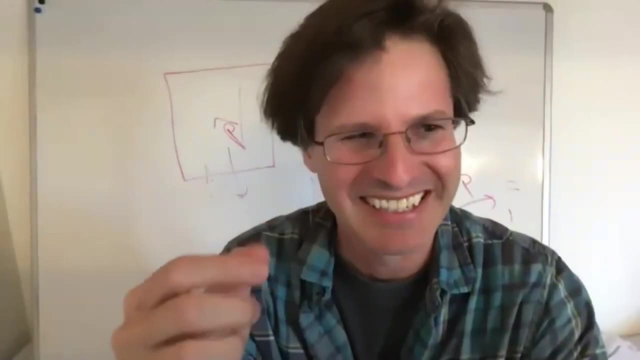 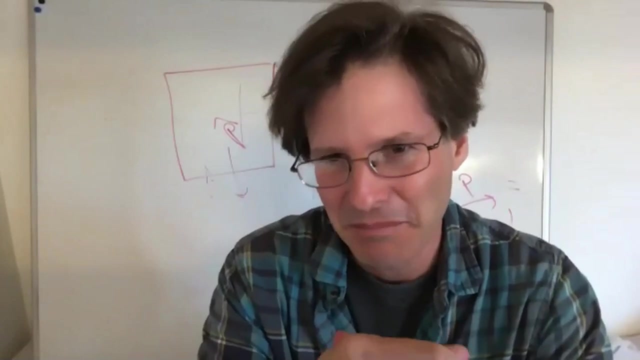 I mean, yeah, like I said, I feel a little bit stupid because I somehow I just got into this because of my friend Peter and then I was so focused on the octahedron I didn't think about, like, what happens for the tetrahedron. You know so, but again, it's not centrally. 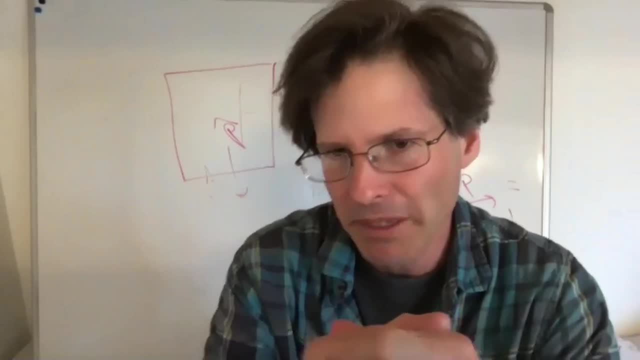 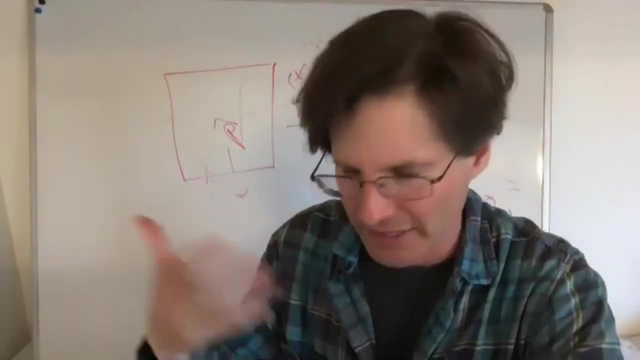 symmetric, so it's a slightly different. you know, probably, But you know my, my guess is it's. I would say that in general, the answer is that it should be piecewise, algebraic, like like there are. these zones should be able to break the thing up into zones and 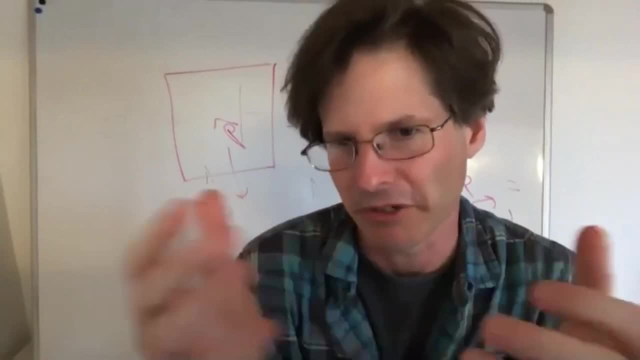 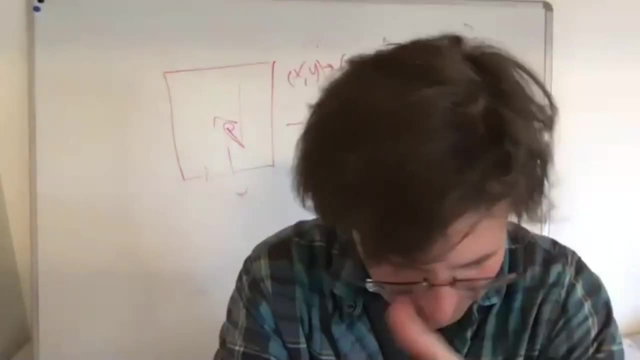 in each zone. the map should be given by a ratio of polynomials or something in the right coordinates. So I actually think it's like a good thing to study, because you know you can, you can take your pick, you know you can try your favorite. Again, there's some. 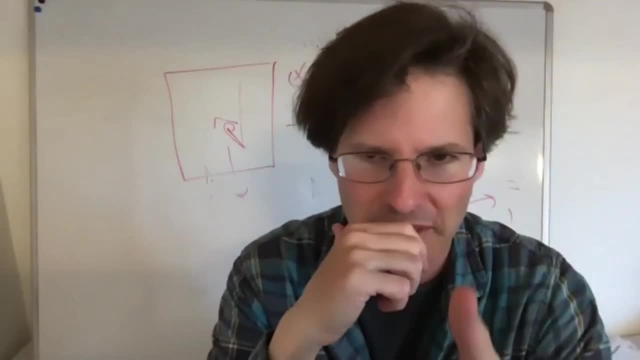 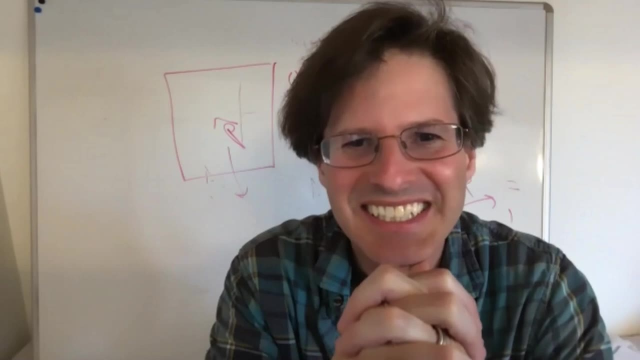 there's been some work done on this and for general convex shapes And there are some references in the in the paper. To ask another question. but the most surprising thing for me was that they were in fact bilinear maps, So movies transforms on those single components. 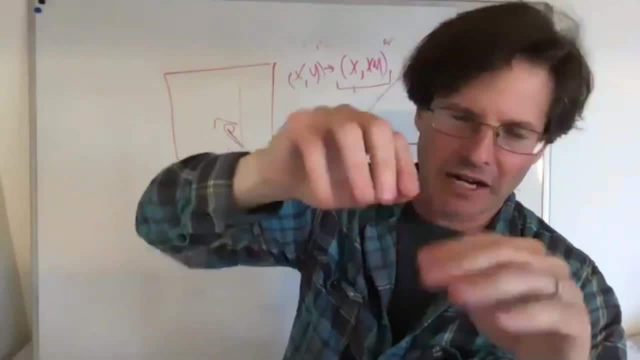 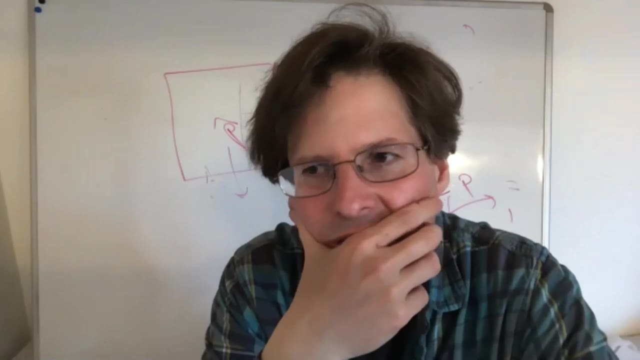 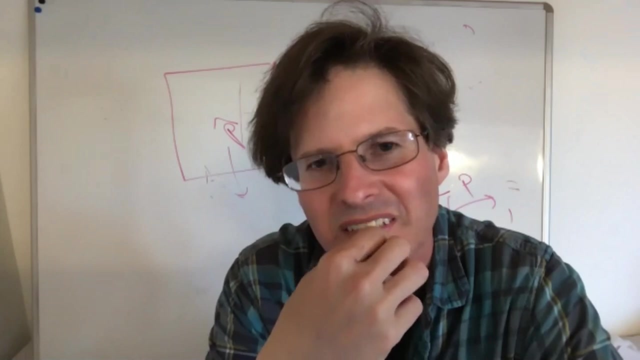 At least on the lines. Yeah, on the on the lines, But do we have any? yeah, do we have any relation in how we have different movies transformed on each different line? Or maybe, to ask the question concretely, What I kind of want to know is what happens to images of circles. So if I take a small 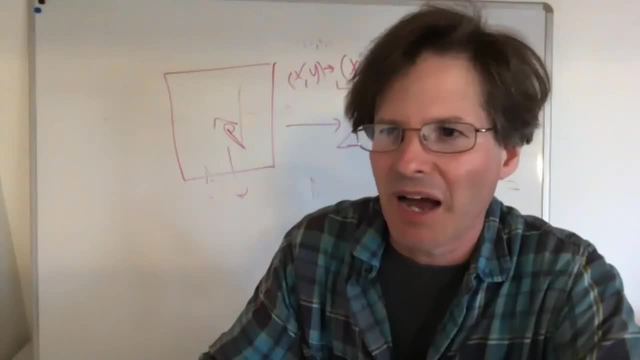 circle, because whenever I see movies transform, I want to map to a different circle. So okay, So I mean the paper, okay, So. so one thing I can say is: like you can write down the formula, Okay. 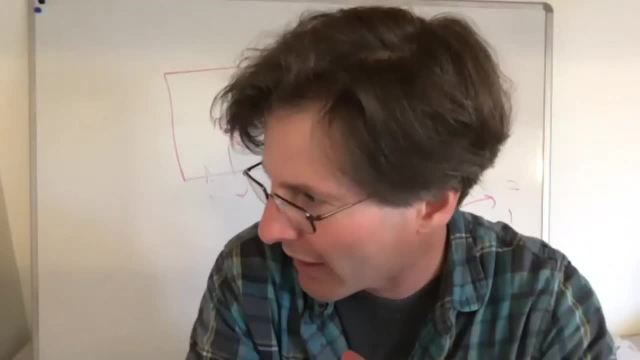 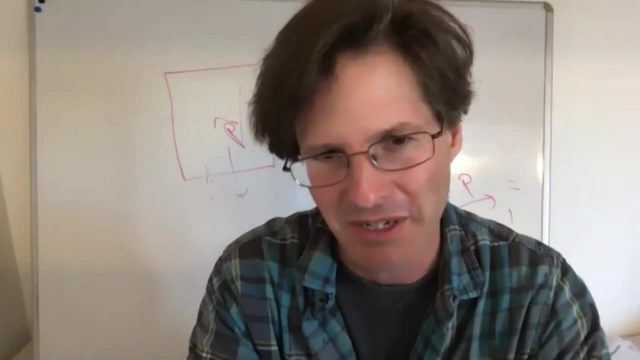 And and then, like what happens to circles? That's a really good question. I mean, well, you know they, they turn into some kind of you know algebraic blob. Okay, I mean, they get, they get compressed. 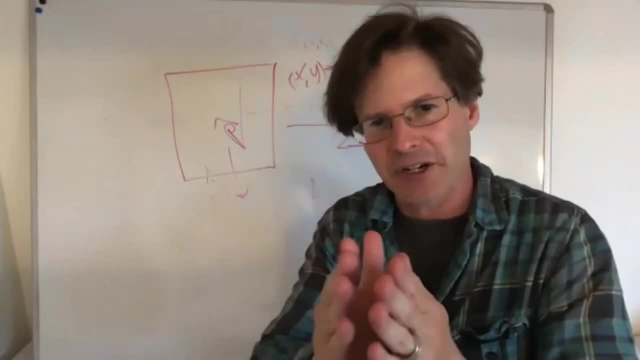 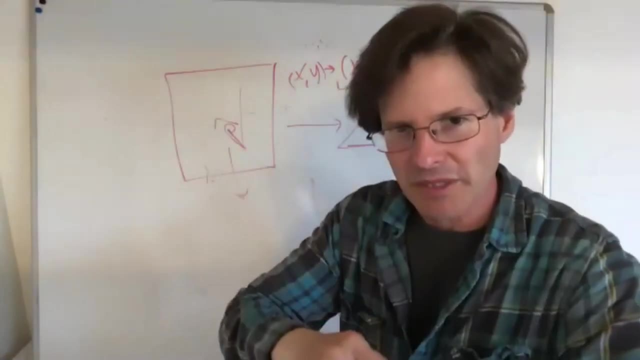 So like. so, if the circle doesn't cross this J curve, it kind of gets squashed into the boundary. So it'll become, you know, more and more like a noodle and just. But it's not something very simple like just becoming elliptic, or it's going to be a bit. 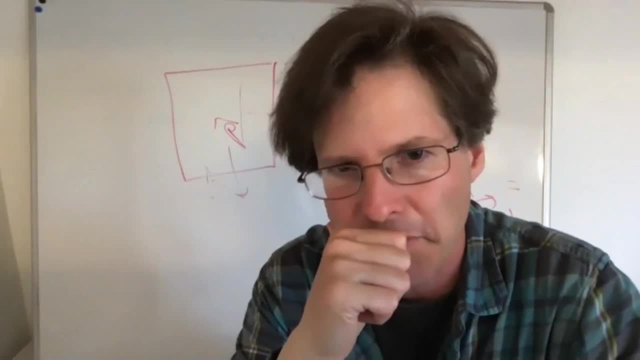 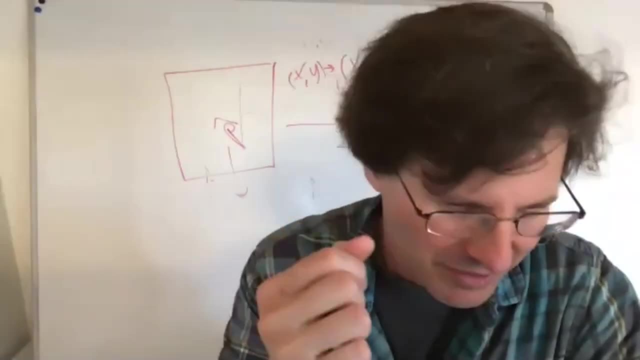 more tricky. I think so. It would be cool if it was an ellipse, but I don't think it is. I didn't. I mean, actually there were some additional things like I actually wanted to sort of plot what happened to the J curve under both sides of the map. 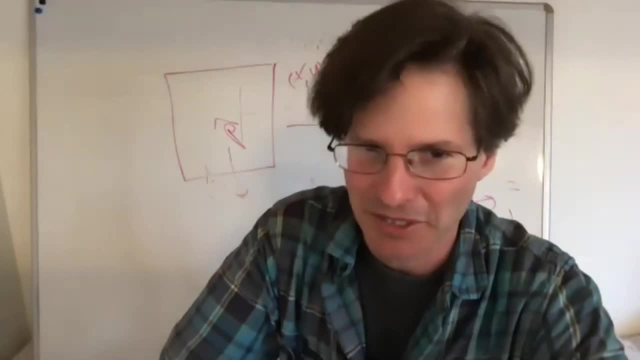 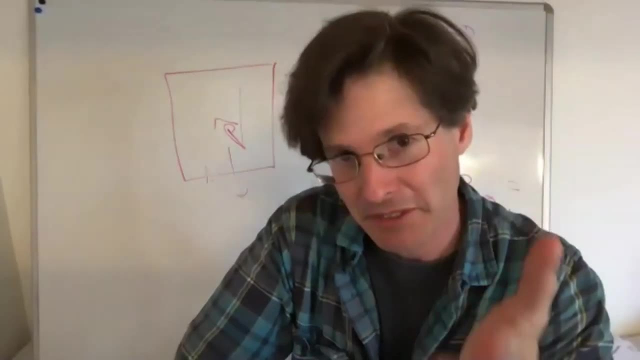 I just- I'll probably add that at some point to the program, but I mean, that's like, that's a really good intuition, a good instinct, Like when you, when you have maps of the surface, it's a it's a good idea to look at what happens to curves. 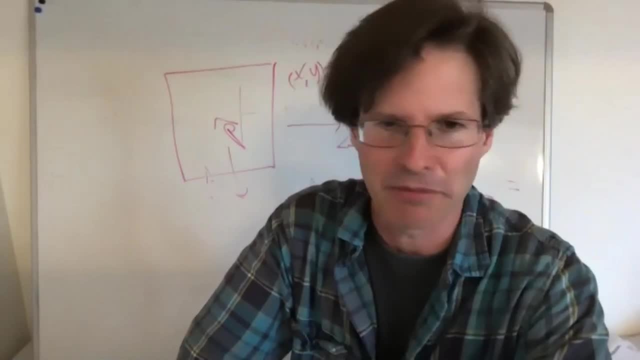 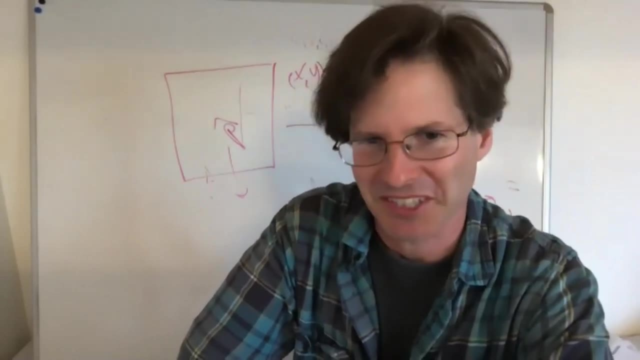 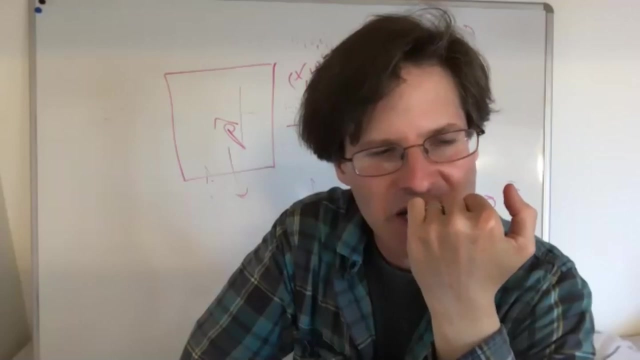 I know this will. this will tell you a lot about what's going on, But but I didn't think too much about what you actually get. Thank you, Sure Awesome. So do you think there might be some other geometry on the surface of the octahedron? 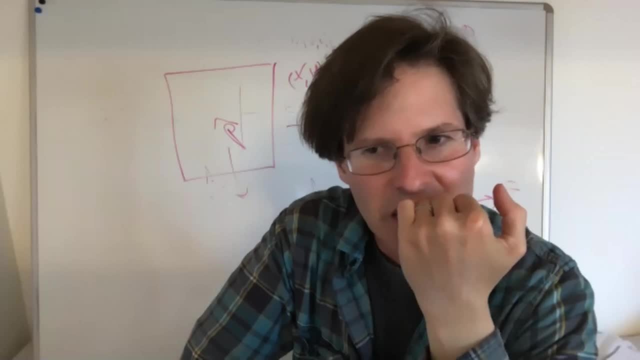 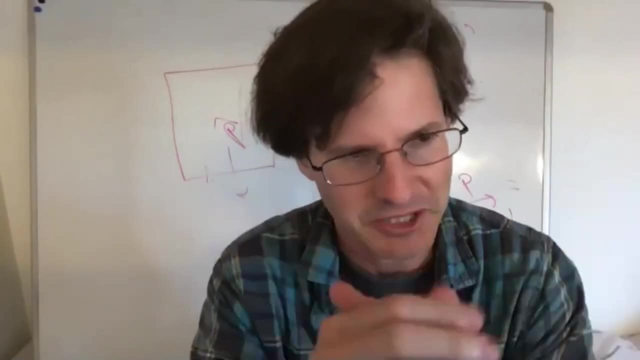 which could make them up even nicer. That's a good. there is, yeah, there is. So the other, the other geometry that you would want to try would be hyperbolic geometry. If you know about hyperbolic geometry, it's well, it's like a non. if you don't, it's a. 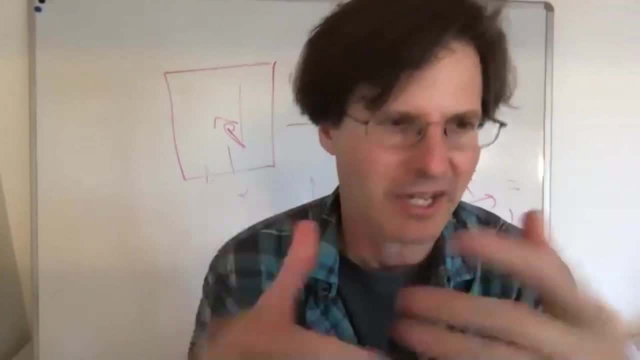 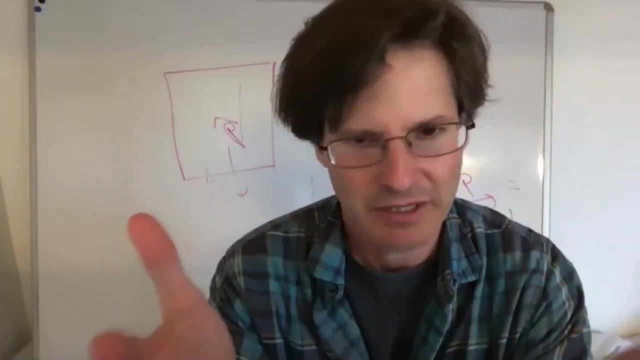 it's a non-Euclidean version of the Euclidean plane and it's got all the same stuff. It's got symmetries, it's got geodesics- you know straight shortest paths- it's got triangles, Polygons. 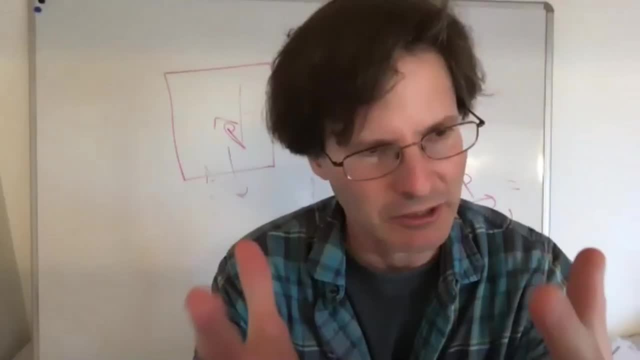 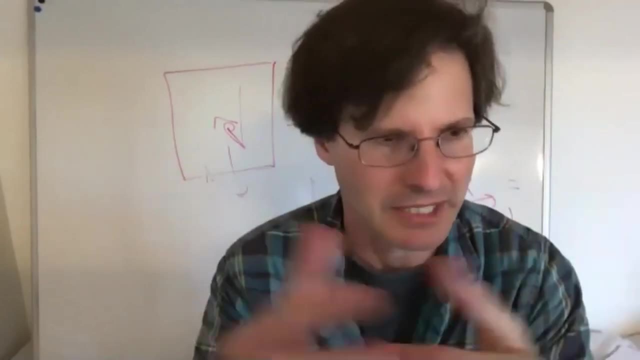 And you can. you can take eight, eight identical triangles, and and, and glue them together and and, and get a kind of hyperbolic octahedron. And, and probably the nicest one is where all the triangles are what's called ideal. 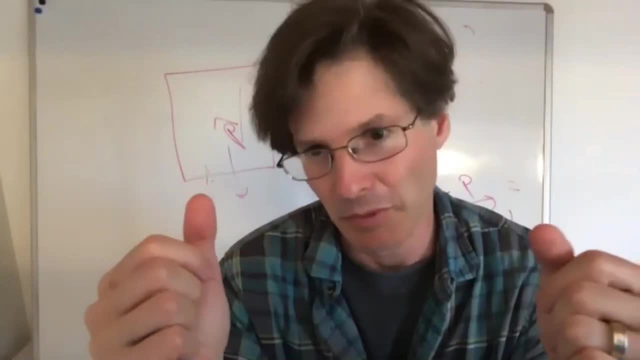 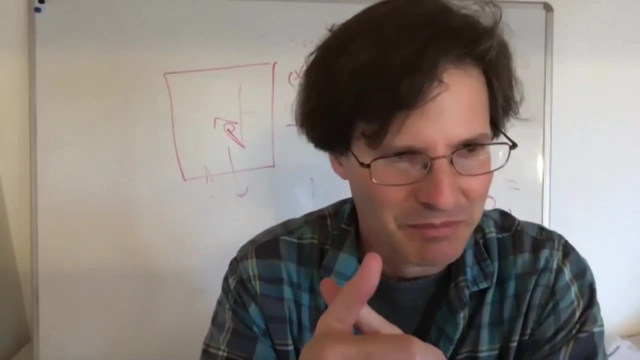 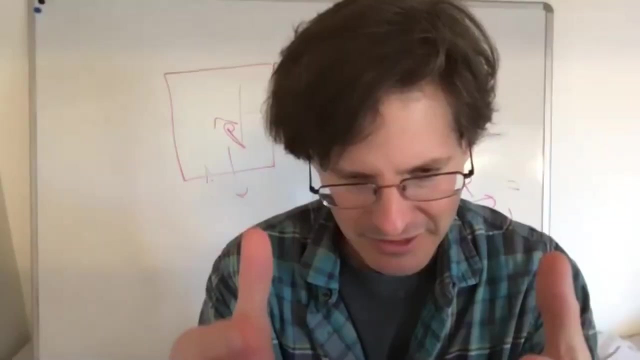 It's sort of all the angles are zero. So this is what people call the ideal octahedron, And you can like look at, look at that metric. There's an interesting thing: When people, people study these flat surfaces a lot, there's somehow two geometries to them. 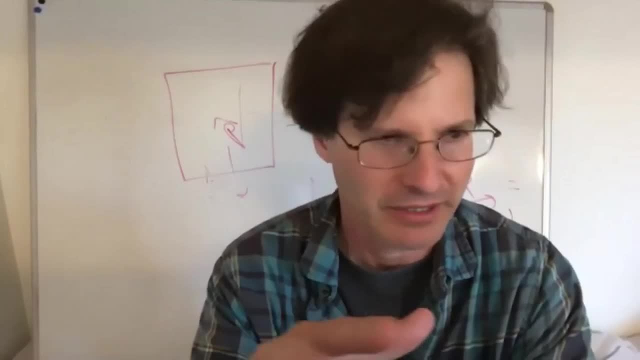 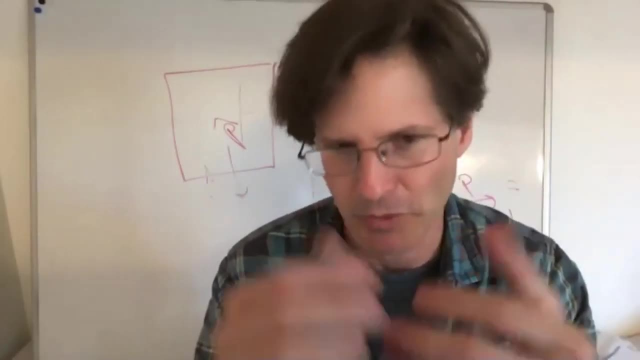 One one is: there's like this kind of flat metric that I was talking about, And then there's also this hyperbolic metric, which comes from thinking about it as a Riemann surface and applying what's called the reuniformization theorem. 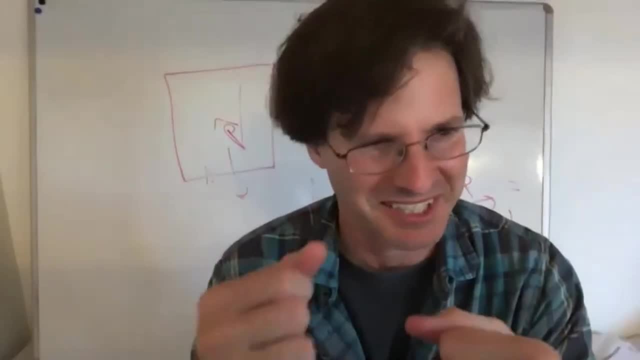 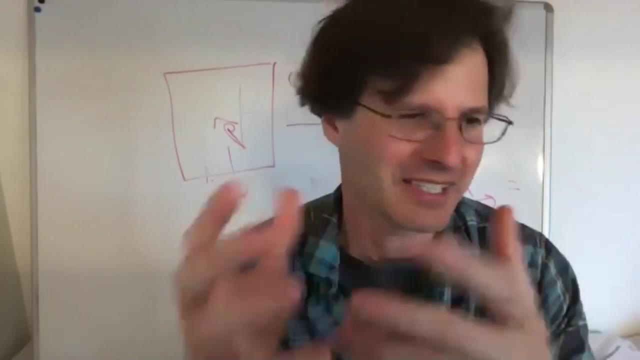 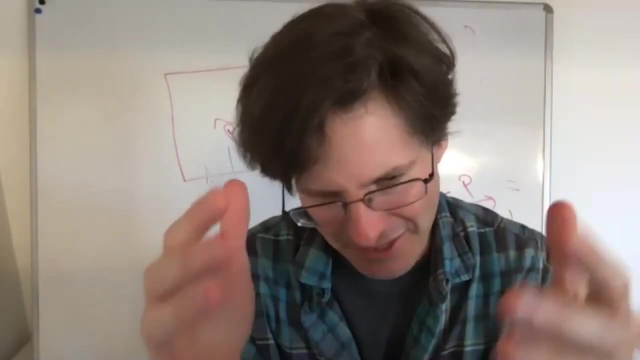 And people sort of like study these things simultaneously. Like it's not exactly clear how the metrics are related, but but somehow you know that the thought is that one metric kind of gives information about the other and vice versa, And somehow, like it's like this other very, very symmetric metric on the octahedron. 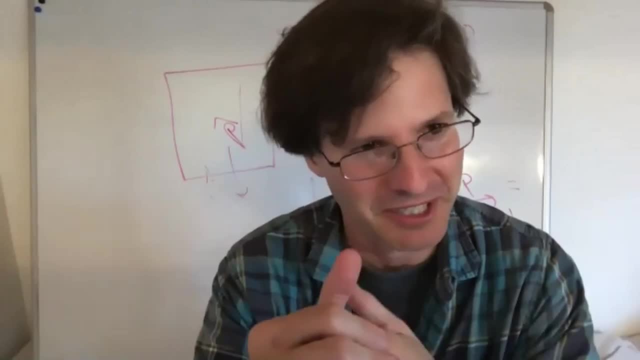 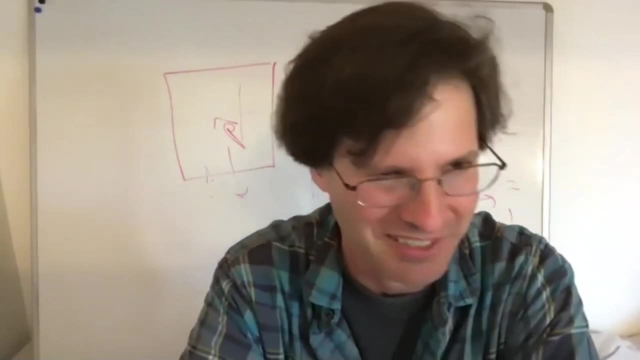 And you know it probably. yeah, it's probably an interesting thing to look at. I mean, I didn't try it And some some problems become like infinitely harder in hyperbolic geometry and some become easier. It's sort of a weird. 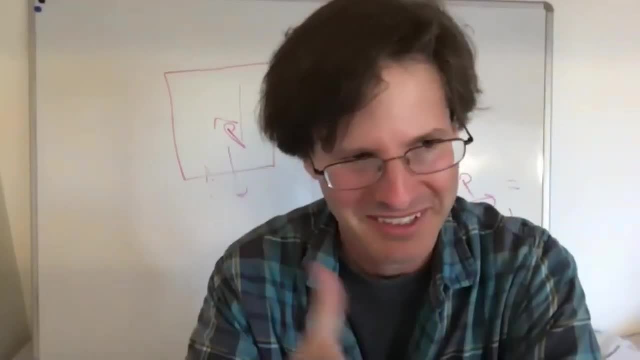 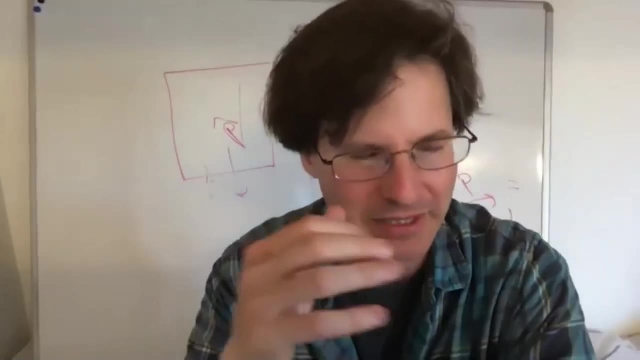 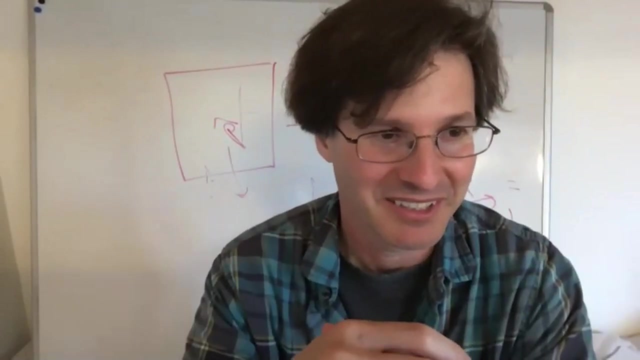 state of affairs, like like you know, sort of. so I guess I'm saying like that would be the other thing to try. Or you could make it out of spherical triangles and think about what happens like on a sphere, kind of a spherical cone metric, where it's like it looks like a sphere everywhere except it's six points. 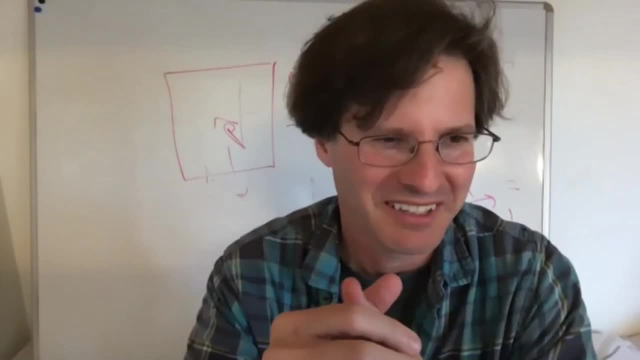 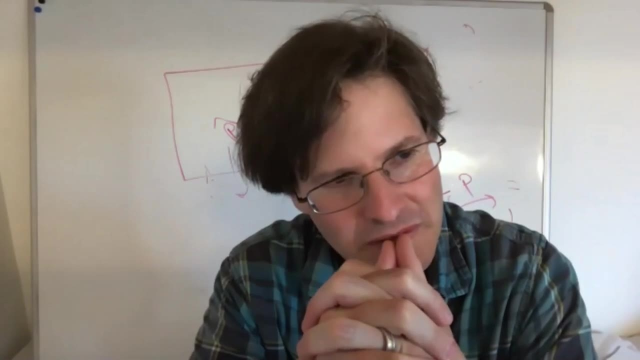 So that that that's also kind of a cool thing. I mean, I would just say that if you did on a sphere, wouldn't this essentially be just a phasor point map into a sphere, which is slightly boring It would be, but imagine. but imagine now that you modified the metric on the sphere. 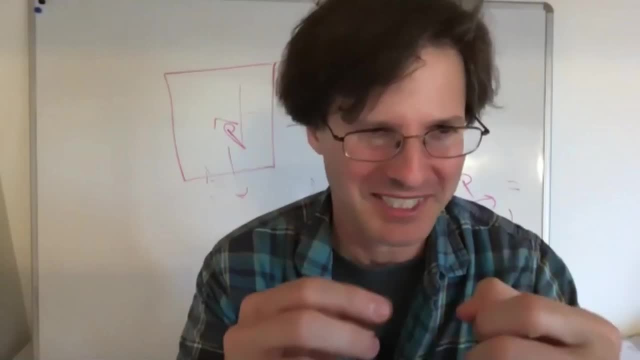 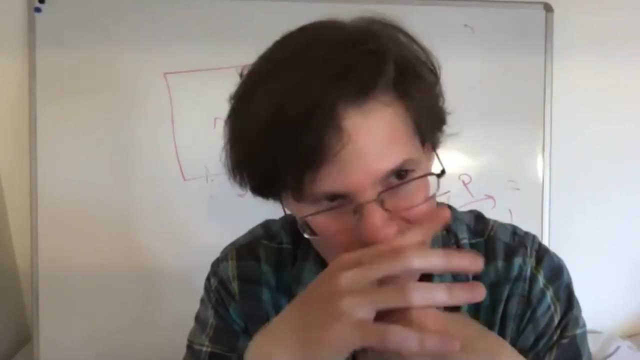 so that it was still spherical, except it's six points, And at these six points it had a. it kind of looked like a kind of a spherical ice cream cone. Yeah, Okay, So you can do that, And I think these things are, I'd say, not well understood. 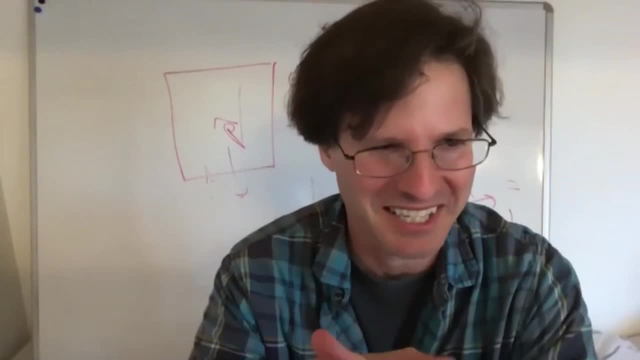 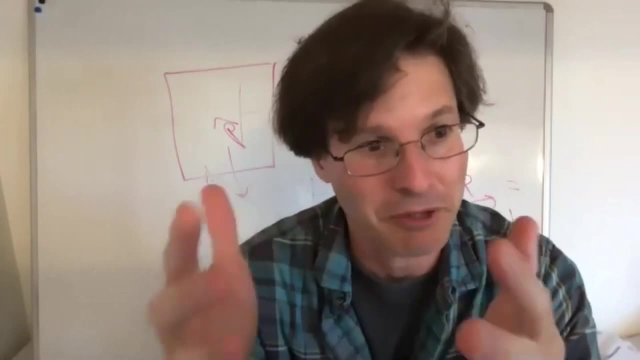 even though you know people, people study these things. I think people are pretty interested in what's their geometry like And I think these are kind of great projects for for people you know: students, grad undergrads, grad students. 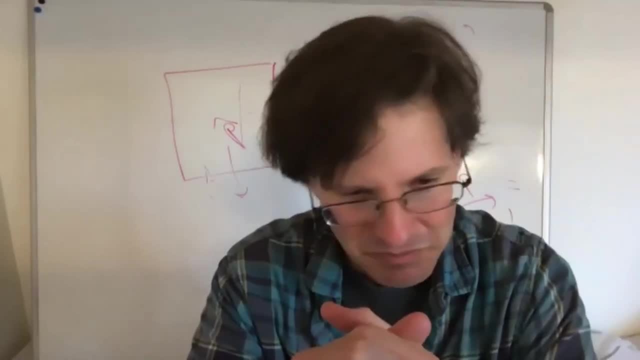 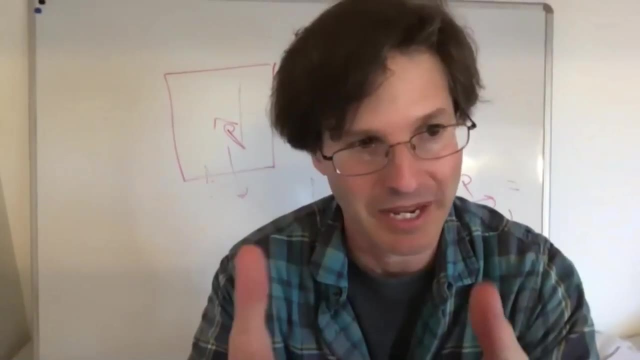 And you know, just because, like you can sort of, if you're, if you like coding things, you can actually just try it. You know, you can eventually code it up and just see what happens, And then, if you're lucky, you can prove what you see. 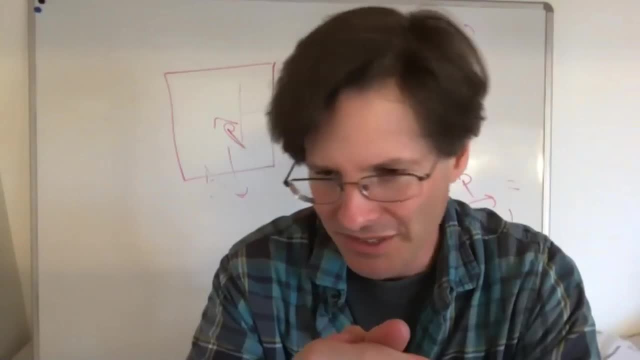 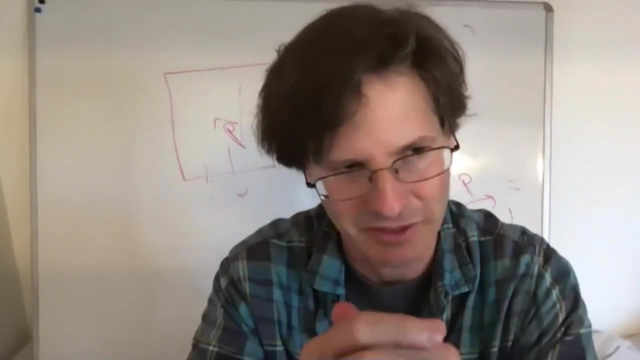 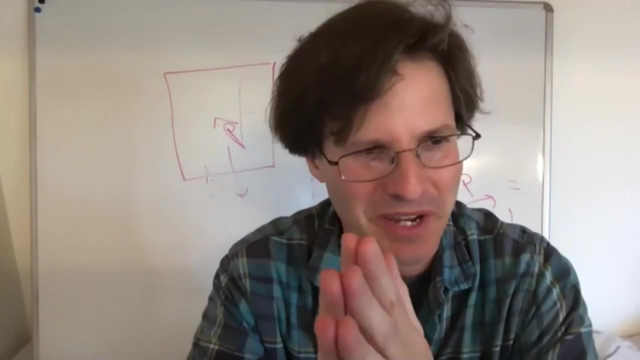 So yeah, So anyway, those are. those are like the three metrics you would. you would try- I'm hyperbolic- some kind of spherical thing and flat. Yeah, Thank you, Sure, So anyway, well, I mean, yeah, I mean thanks for thanks for having me do this. 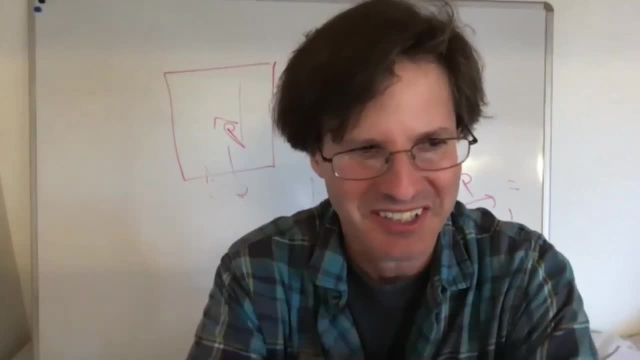 Yeah, Thanks a lot, It was really interesting. Yeah, Thank you Thanks.